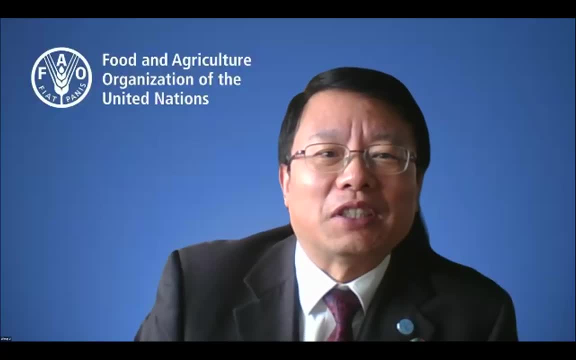 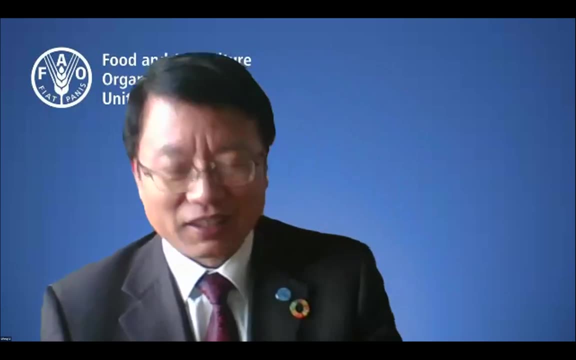 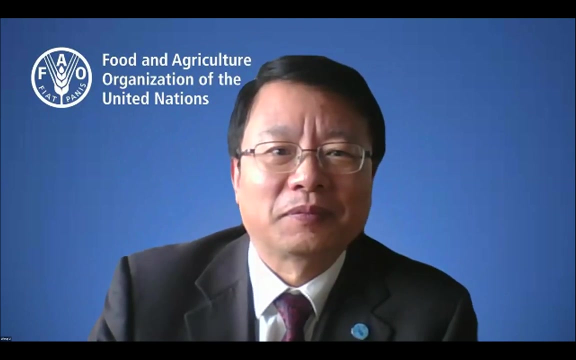 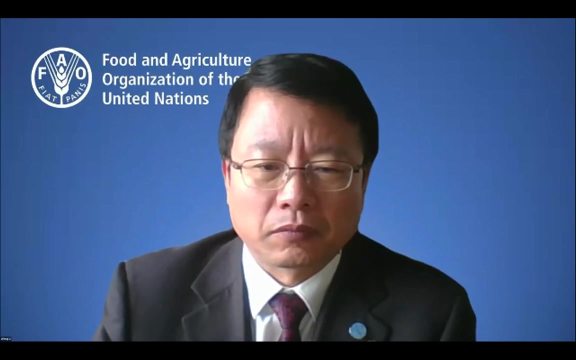 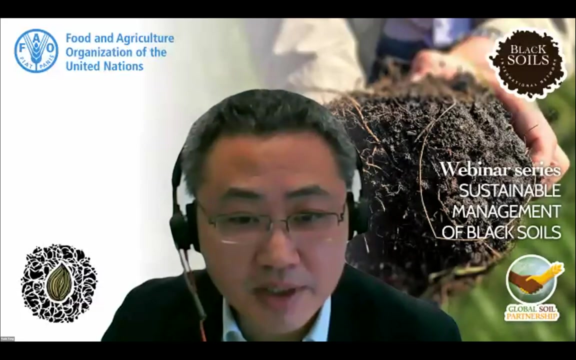 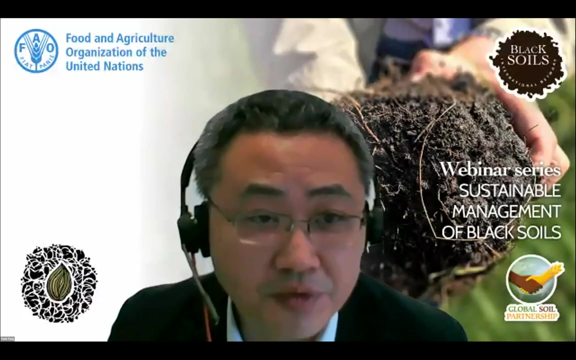 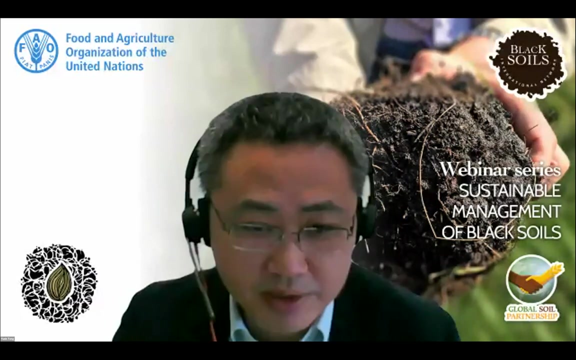 And good evening to Professor Jia. Thank you, Nice to meet you. Good morning, colleagues, participants. Perhaps we should begin because it's 1 pm of Central European time. Good morning, good afternoon, good evening, dear participants. 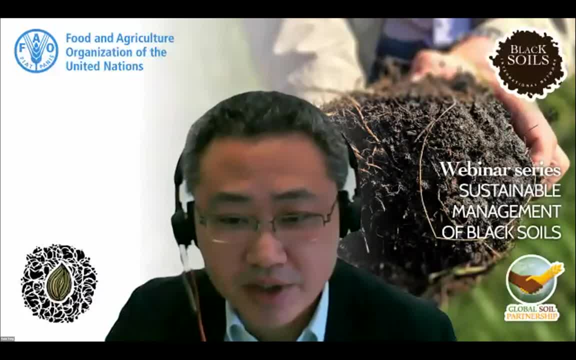 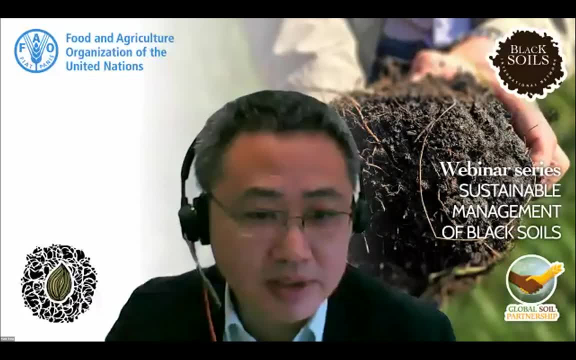 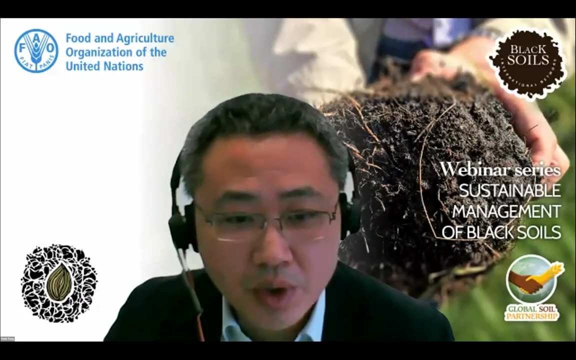 On behalf of the Food and Agriculture Organization of the United Nations, may I welcome you to this webinar entitled Sustainable Black Soil Management: a Case Study from China. I'm Yuxin Tong, working at FAO, and will be the moderator of today's webinar. Black soils have been prized for their rich organic matter content. 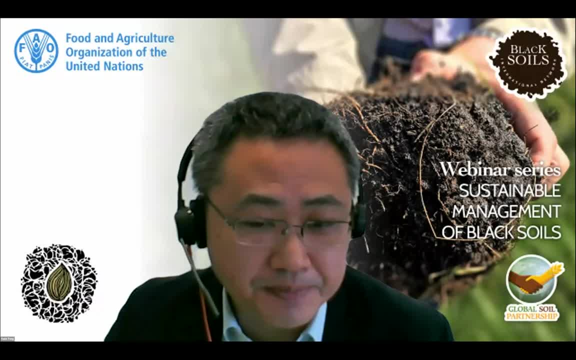 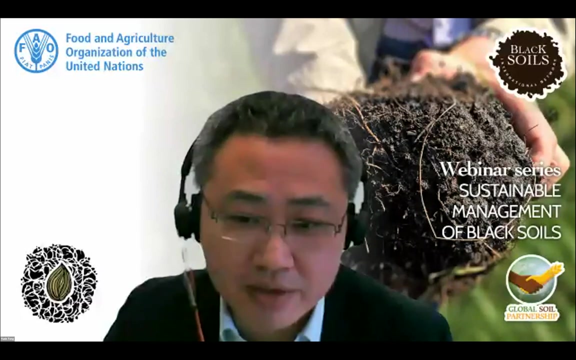 and the great nature, fertility. However, this rich treasure is under threat. FAO, through its international network of black soils, is committed to the conservation and sustainable management of black soils In order to raise awareness about the vital role of black soils for food security and climate change mitigation. 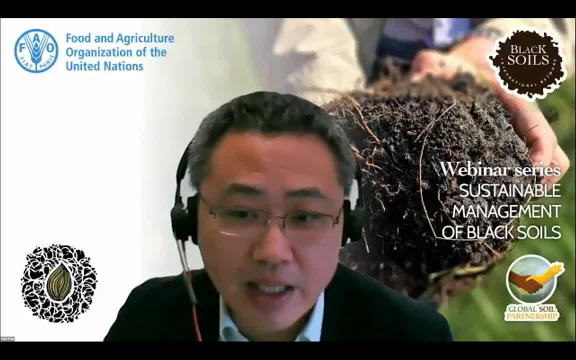 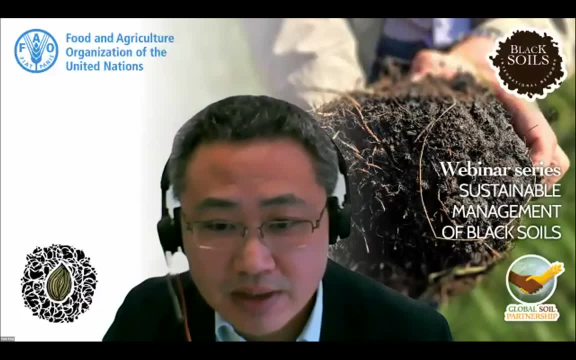 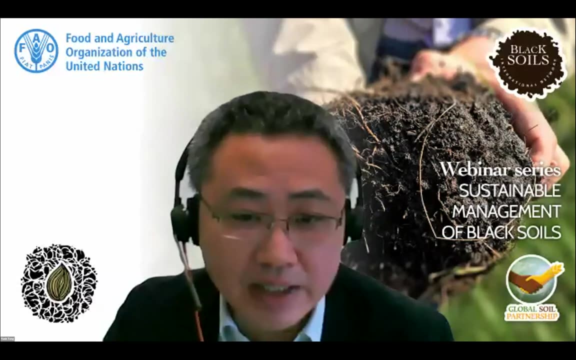 and introduce good practices on sustainable black soil management. Black Soil Network and its members decided to organize a series of webinars, So today we'll be listening good stories and practices from China, a big black soil country, In today's webinar there. 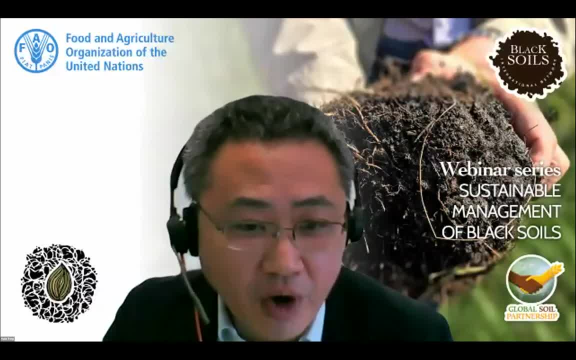 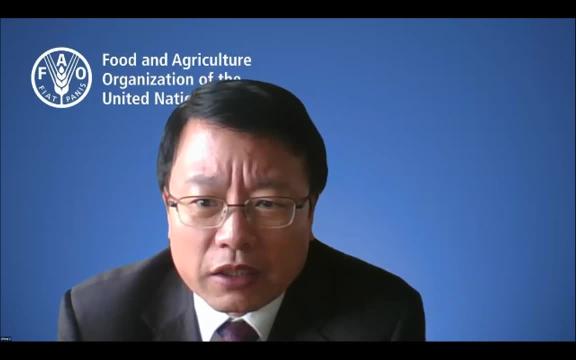 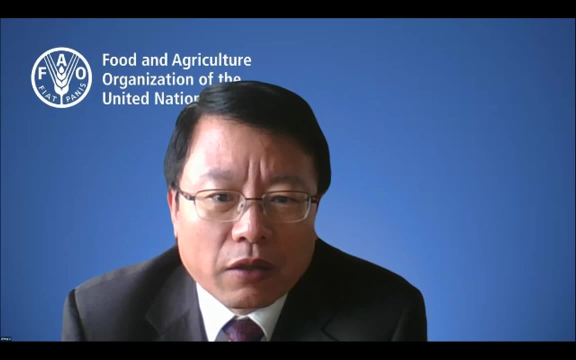 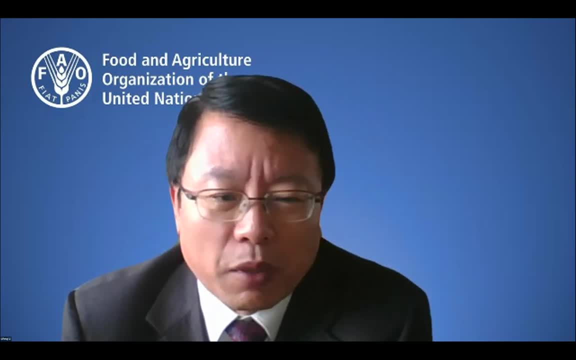 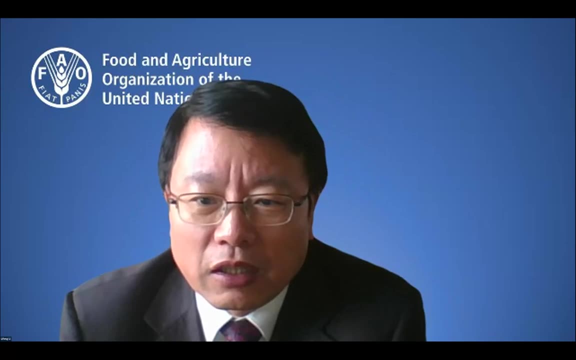 of the seven technical networks of FAO's Global Soil Partnership. As mentioned already by Dr Teng, black soils are the most fertile soils on the world. They are distributed in many regions across the globe, such as the Great Plains of North America, the Tan Pas of South America, the Eurasian steppe in the northeast of China. 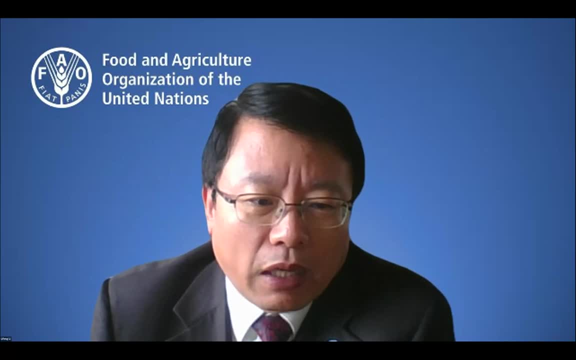 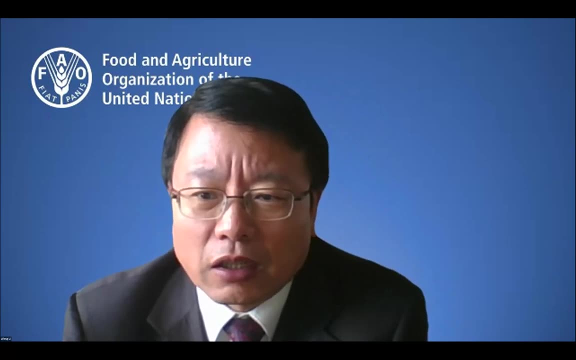 and other places in Africa as well. Black soils are characterized by their high organic matter content, dark color and also their fertility and ability to retain water. They are essential for the production of crops and livestock. To understand the status of black soils: black soils are the most fertile soils in the world. 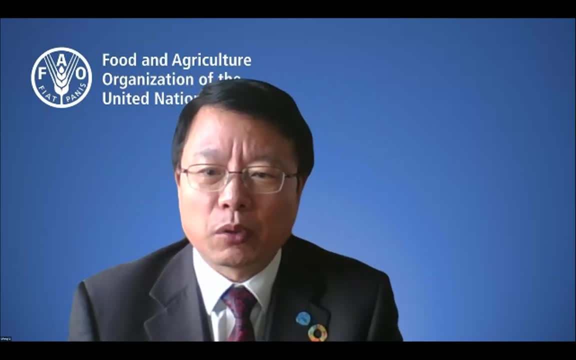 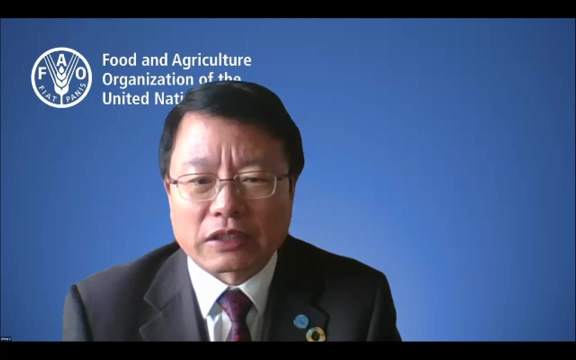 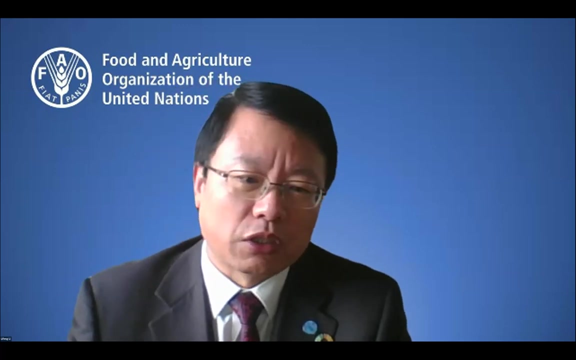 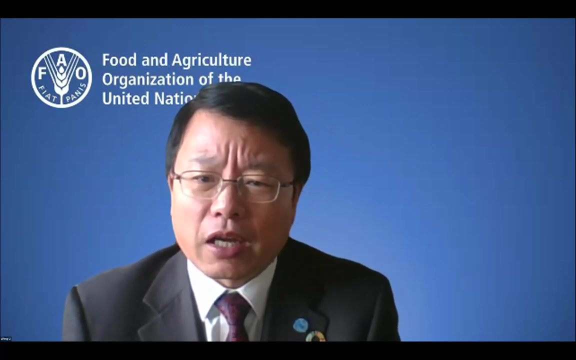 The status of the challenge of the black soils at the global level. with the support of the International Network of Black Soils members, FAO launched the Global Status of Black Soils report on the World Soil Day in December 2022.. I can share with you that the report highlights that black soils are carbon rich and highly. 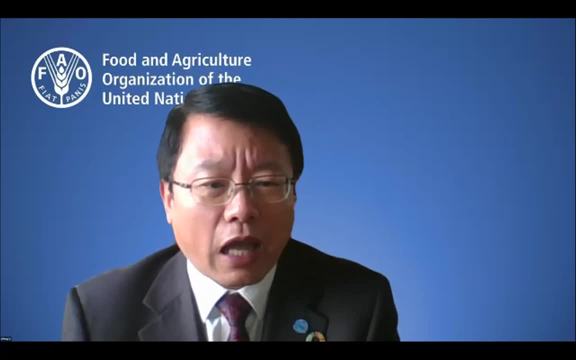 fertile soils that cover 722 hectares. The total amount of carbon generated in black soils is approximately 320 million hectares of the land surface. The total amount of carbon generated in black soils is approximately 220 million hectares of the land surface, Although only approximately 7% of global crop land occurs on black soils, 66% of the sunflower. seeds, 51% of the small millet, 42% of the sugar beet, 30% of wheat and 26% of potatoes were harvested globally from the black soils. This is why black soils are called the food bucket of the world. 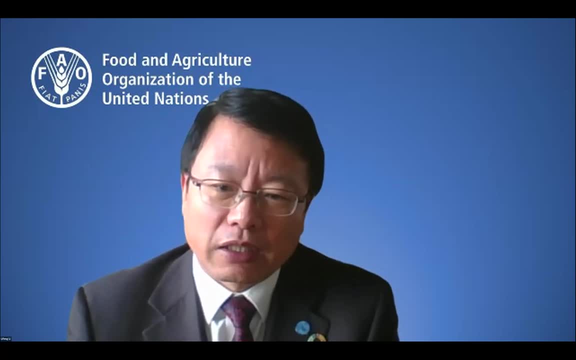 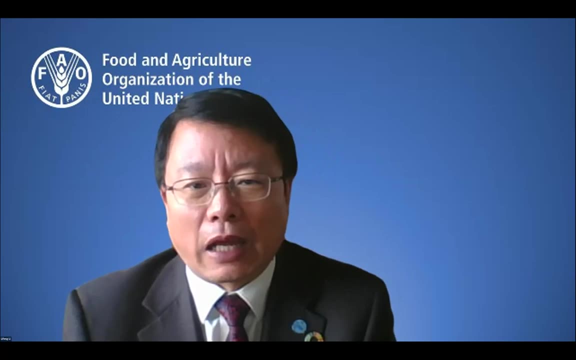 And this is also the reason why they are intensively and extensively being cultivated. Dear colleagues, today's webinar on sustainable black soil management, a key study from China, will turn our focus to China, a country that has made significant strides in managing these precious resources. 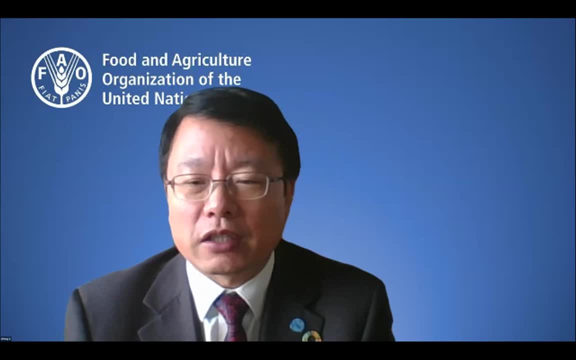 Our journey. in this webinar will explore innovative strategies and the practices that have been implemented in China to preserve and enhance the sustainable management of black soils. Moreover, China is the only country with a national legislation specifically focused on black soils: to protect, to conserve. 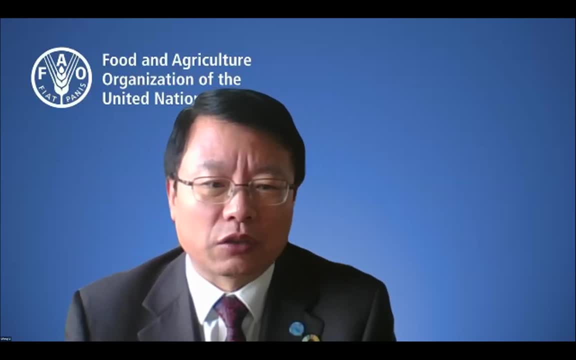 and also to sustainably use black soils in the country. These models are not just beneficial for the crop yield, but also instrumental in combating climate change. In closing, I want to extend my sincere gratitude to the dedicated members of the International Network of Black Soils for your unwavering commitment. 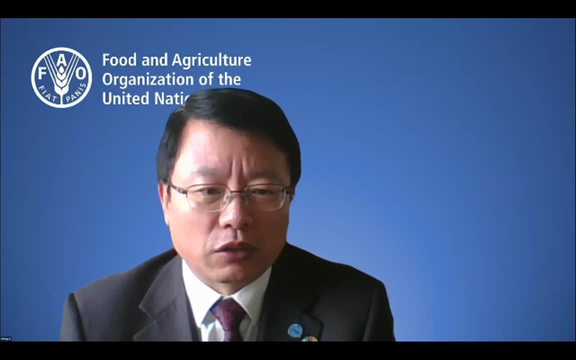 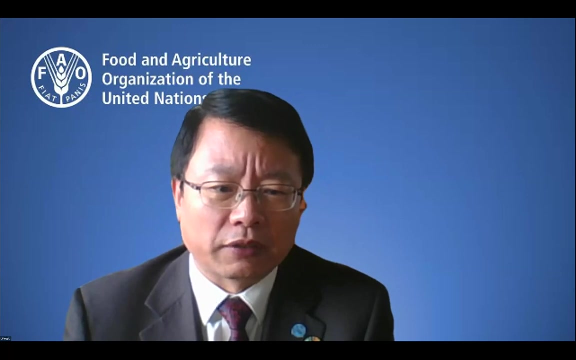 invaluable insights and collaborative spirit towards the conservation, management and sustainable use of the black soils. I also want to say to all the distinguished audience and the speakers my heartfelt appreciation to your interest and your support and your time today. Together, our collaborative efforts will contribute. 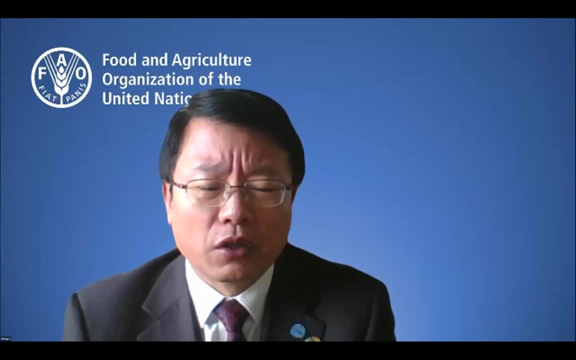 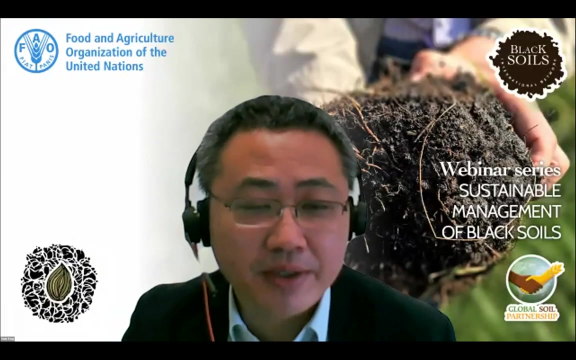 to sustainable black soil management for food security, better nutrition and a living planet. Thank you very much for your attention and I wish you very fruitful discussions. Thank you very much. Thank you very much, Mr Li, and your inspiring speech. 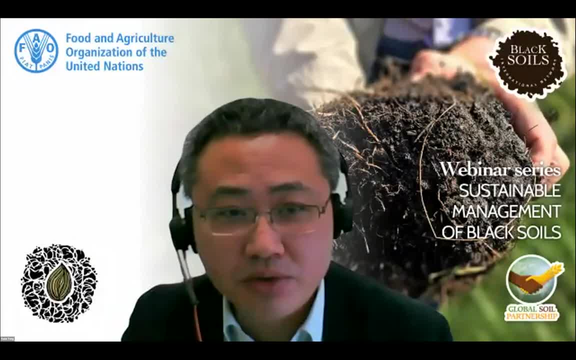 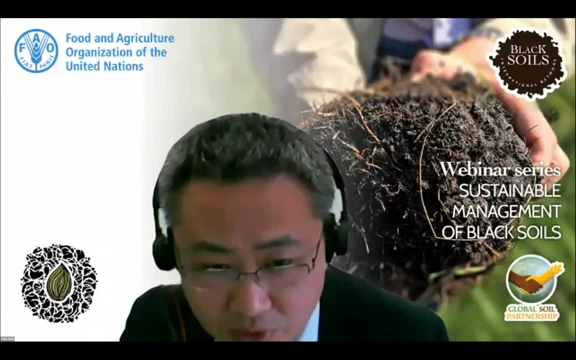 It was very sweet to hear from your colleagues, And I want to give a big thanks to everyone who started this discussion here today. So we are very grateful to all the good people at the International Network of Black Soils for this opportunity to support us. 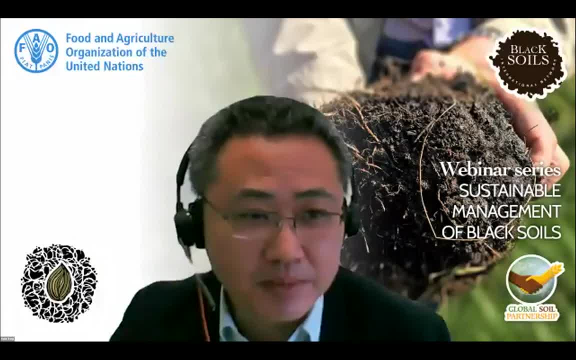 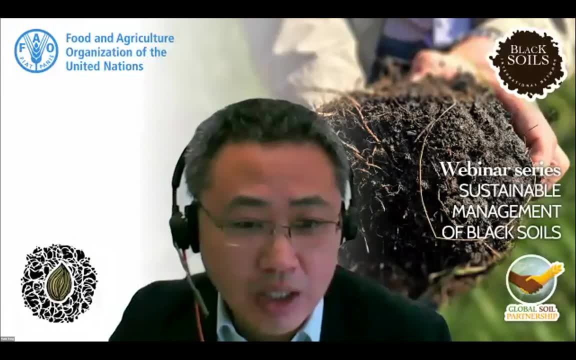 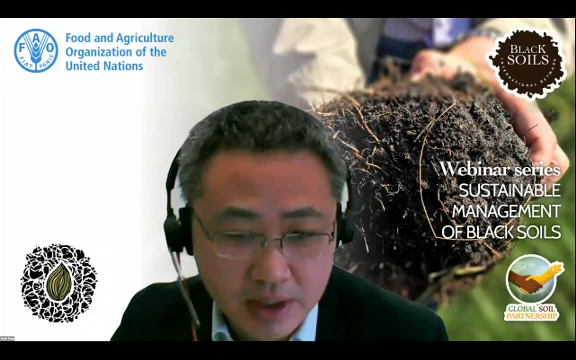 And I am proud to say that black soils are so vital, so important, not only for black soil countries but also for the global food security, because black soil countries export a lot of food. Mr Ganlin Zhang from the Institute of Soil Science, Chinese Academy of Sciences. 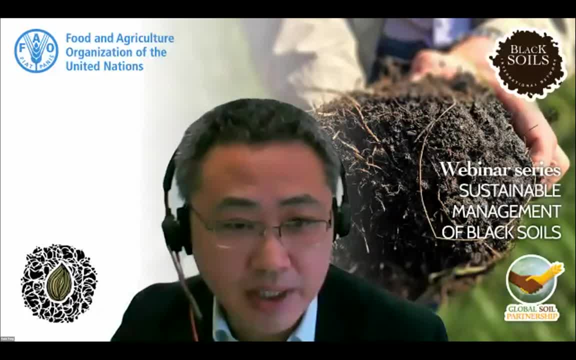 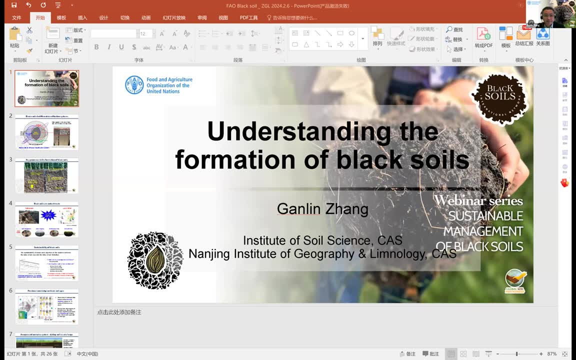 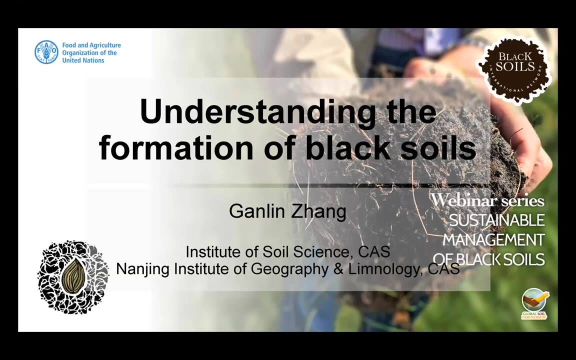 Professor Zhang, the floor is yours, Over to you, Thank you. Thank you, Yuxin. Dear Director Li, dear participants of this Sustainable Black Soil Management webinar, First of all, I'm very much honored to be invited to talk about our most recent study. 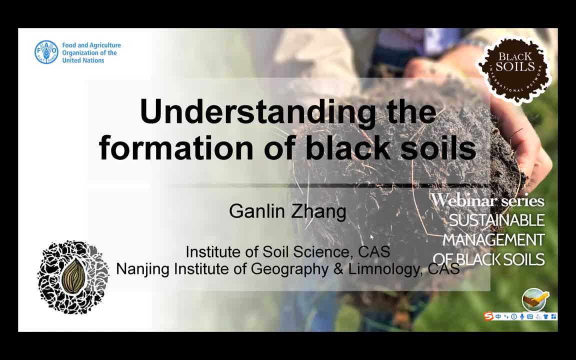 Well, so I changed a little bit the title of my presentation. It was understanding the formation time of black soil. So in this presentation I talk both time and key processes. So now it's understanding the formation of black soils, Some key processes actually. 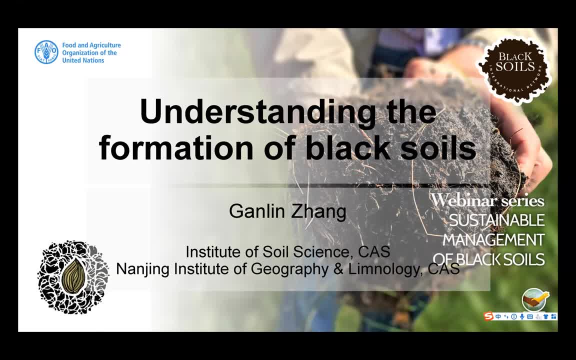 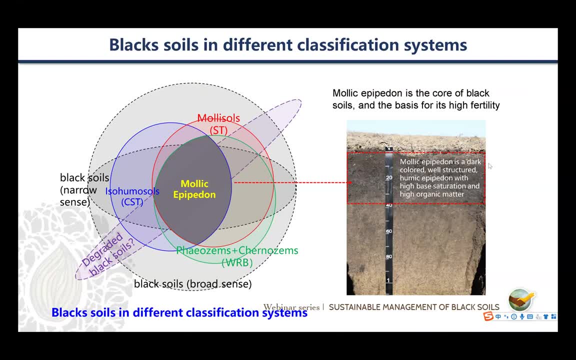 I'm from Institute of Soil Science and, in the meantime, 19th Institute of Geography and Liberal Knowledge, both Chinese Academy of Sciences. Well, all of us, we know that the essence of black soil is it is mollic. we call it dark, dark surface horizon which is dark colored. 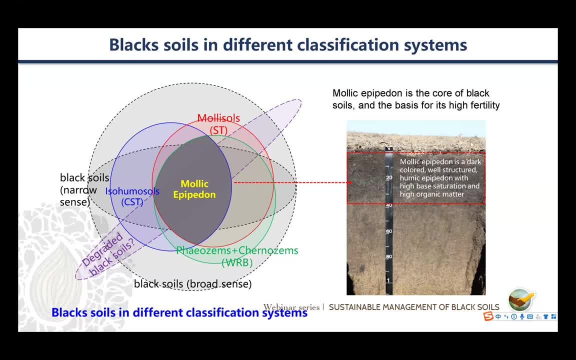 We are structured, It has higher best duration, Most mostly, and high organic matter. So in different definitions it can be more than 1%, or according to iron base it's more than 2% of soil organic matter, But in different national systems, though, 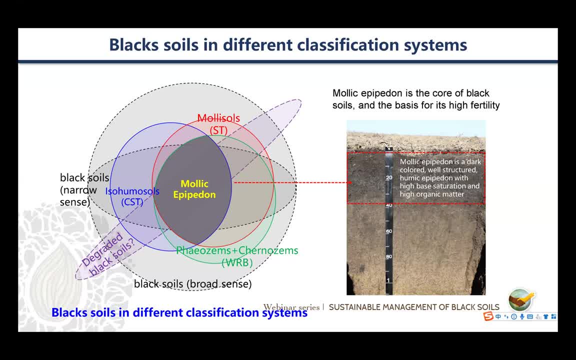 the definition can be a little slightly different, But the essence are the same. So this is. So one thing is important: That the accumulation of humus, the soil organic matter, in this fertile soil. Well, besides accumulation of soil organic matter, 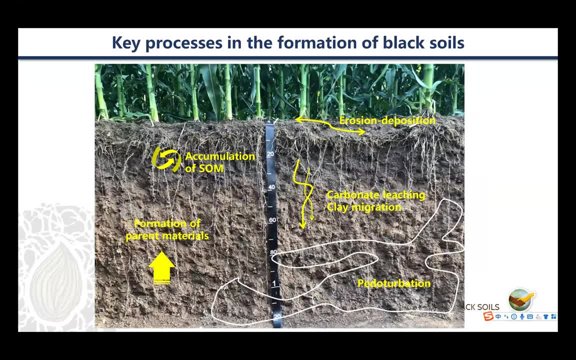 there are many, several other key processes affect soil formation and development of black soils, including erosion, deposition and the carbonate leaching and clay migration. Migration And also we have to understand the build up of the soil is very much, is very much determined by the formation of apparent materials. 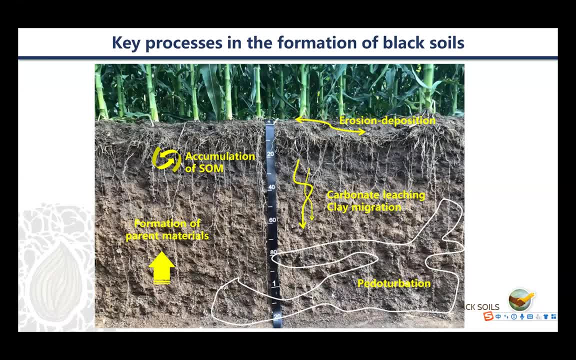 So besides this, we should know there are also very important process, that is, bioturbation or, in general, pedoturbation. We see this figure in the low right bottom, Low right part, this pocket which has a slightly different color. 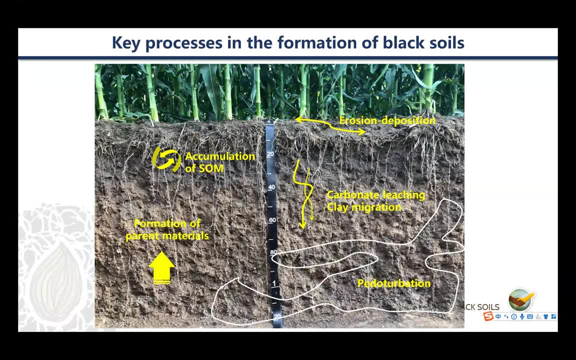 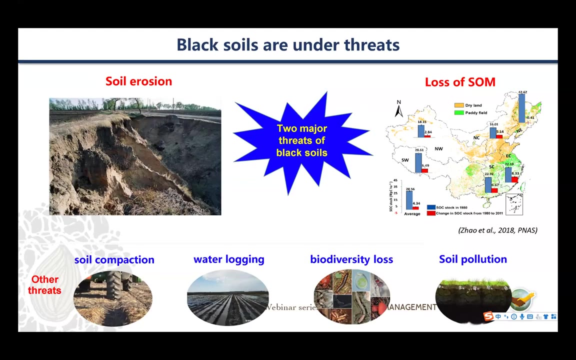 which means the surface material is broad. in this place, That means in black soil, bioturbation or pedoturbation is very common. This is also a very crucial process for the formation of black soils. Well, globally, the black soils are suffering degradation. 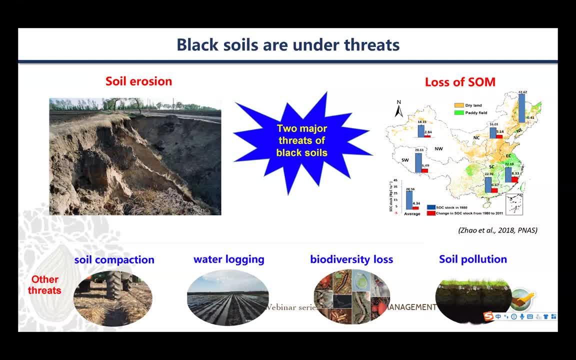 So major degradation process, including soil erosion and the loss of soil organic matter. Besides soil compaction, water lodging, biodiversity loss and soil pollution, So these two major process of soil organic matter declination also involves the loss of soil organic carbon. So if we want to understand the pressure of soil degradation, 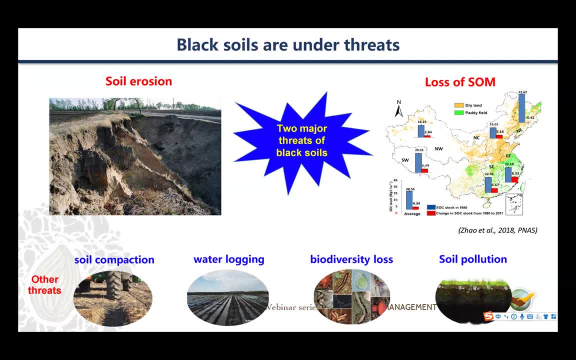 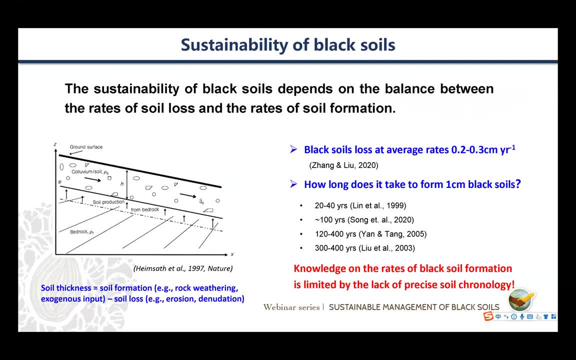 in specifically black soils. we have to know how much, how fast it is formed, Because the sustainability of black soils depends on the balance between the rate of soil loss and the rate of soil formation. Of course we know that soil formation rate is usually much lower than soil formation. 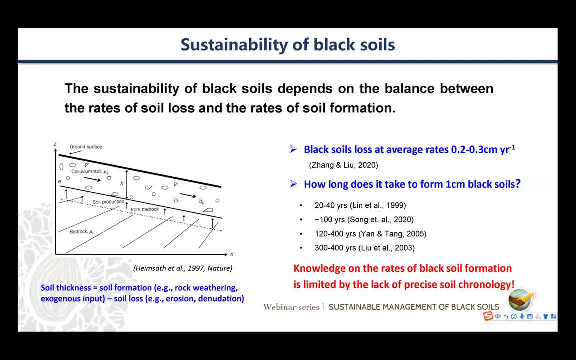 So there are various data on the formation of black soils, including, for example, here I just give to several examples. For example, one say is 0.2 or 0.3 centimeters per year, which is for the loss is very. 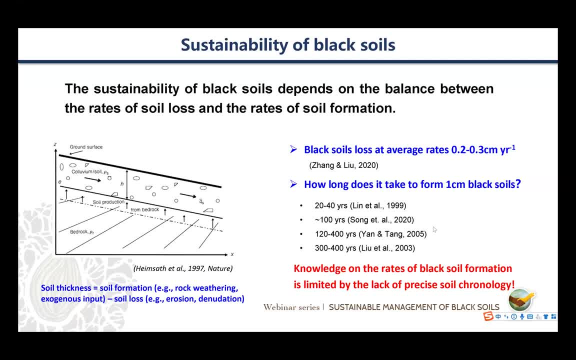 very fast but it takes very long time to form one centimeter black soils. But the data varied a lot. So some say 20 to 40 years, some say 100 years, some 120 or 400 years and some say 300 to 400 years. 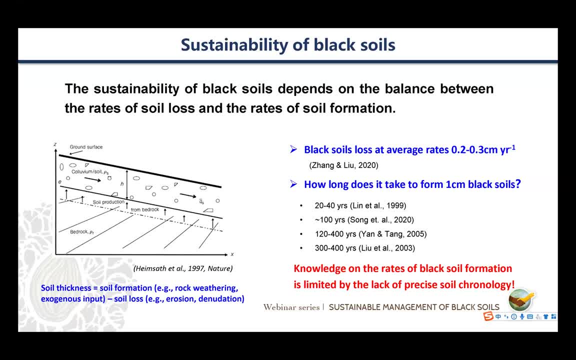 So this data? they are so complicated and they're so varied And actually, I have to tell, none of them has a real data or science based estimation They are coming from mostly a case or rough estimate. So we need really a serious study to know how much or how far. 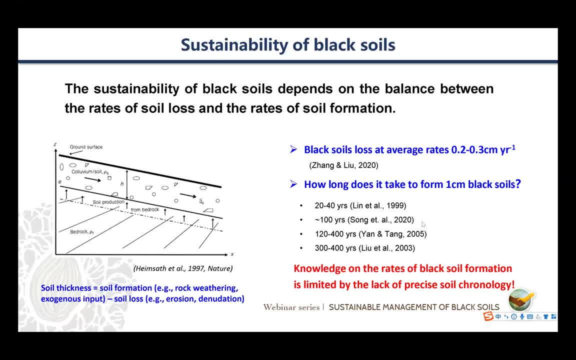 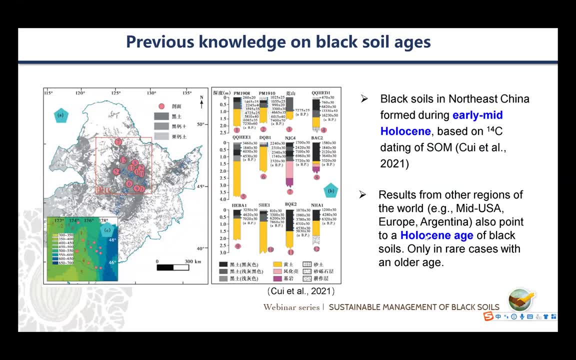 how fast soil this soil is formed. There are serious studies on the formation time of black soils, For example, this study from, also from China. they collected many piece in Northeast China. They dated the soil carbon using carbon 14 technology. 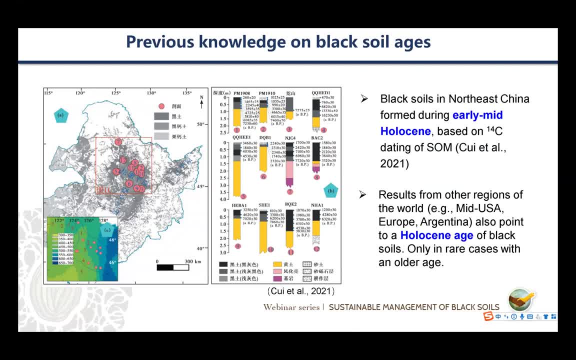 So the result is this: this soil started to form at Holocene age. It's about eight, So after after Holocene that means younger than 10,000 years. So mostly they are from 8,000 to 7,000 or 6,000.. 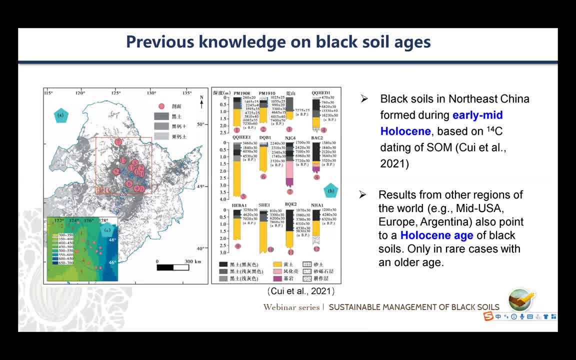 During this period of time. this, however, this also is in consistent with studies from other parts of the world, from such as the middle USA, European, Argentina. They also point to this Holocene age of black soil, So this is a. 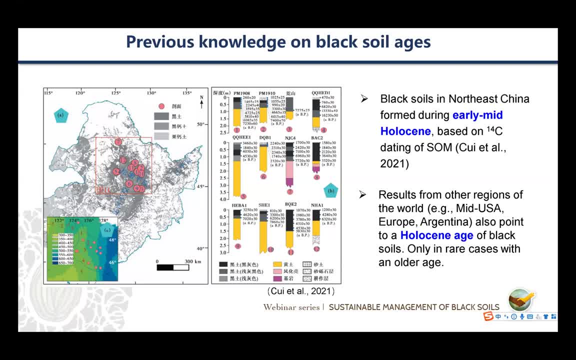 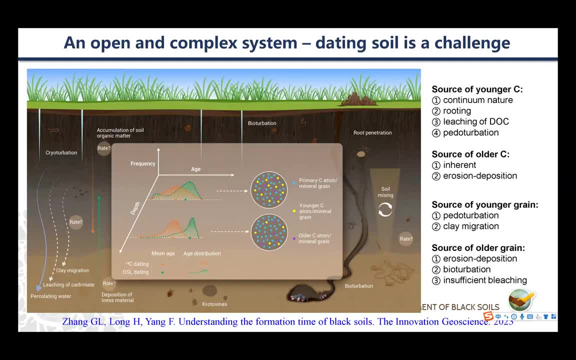 if this is the case, we have to understand the age of carbon 14.. What does this carbon 14 date mean? So, but we have to know the carbon in this soil, in actually in all soil, is rejuvenated after it is a formation. 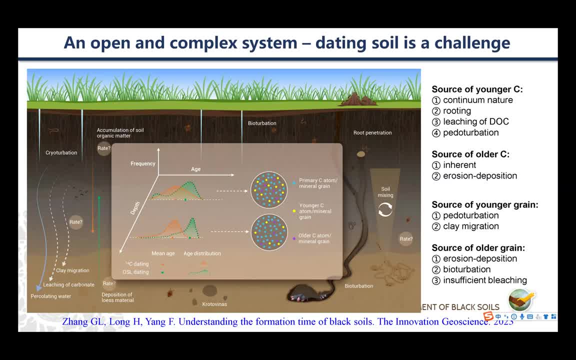 because they are complicated: mixing process of soil, organic matter, including leaching root, rooting, turbation, bioturbation by either small animals or either by termite or all kinds of these activities. So recently we present a framework for dating soil using carbon 14 and OSL technology. 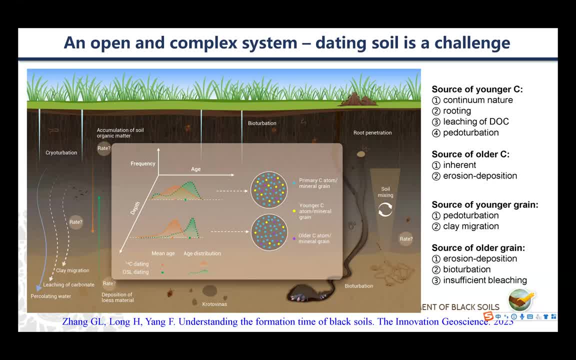 So, because the source of carbon can be different, can be from and the, the, all, the, the, the young, young carbon, new carbon can be transported from a surface by route to the, to deep soils And also. 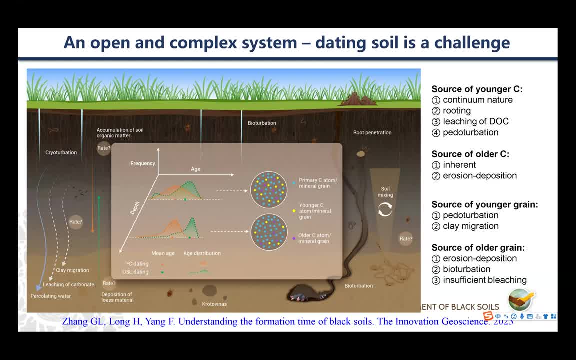 yes, the carbon altimus. they are inherited from all sources, So there is a. this is actually the age of soil. carbon is a spectrum, It's not a one data. It's a distribution of all kinds of age And similarly. 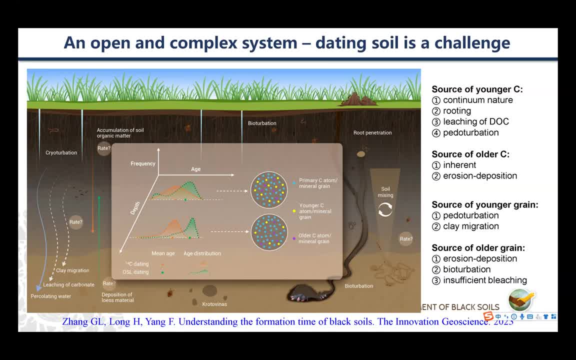 the grain, small grains, of either quartz or fed spire. they also have a distribution, a distribution of age, because they also have different sources. So unless we use very single, single grain or single carbon technology, we could not solve this. 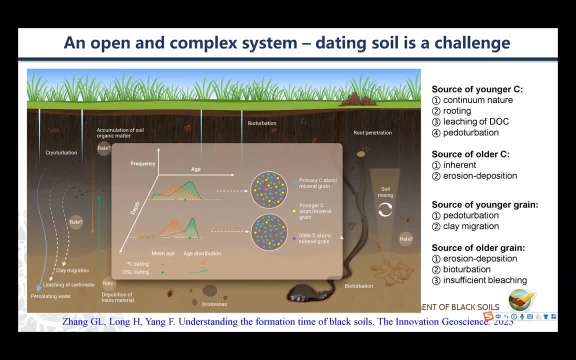 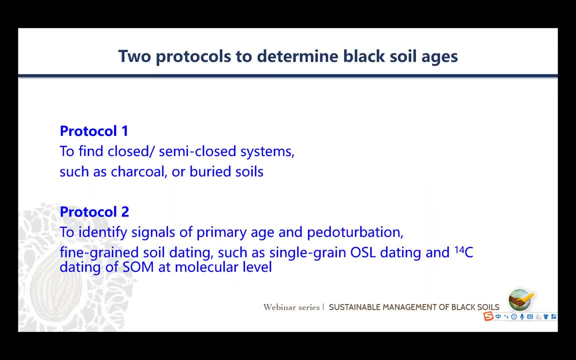 the distribution problem. This is the case. We have to have some new technologies. So if we want to understand that the soil starting starting age of black soil, we have to, we have to put them in these two protocols. protocols. 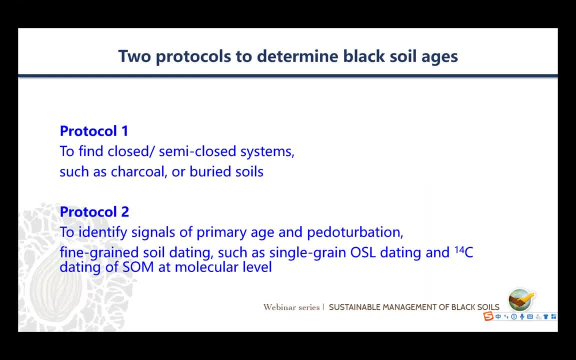 Once we need to find a closed, a semi-closed system so that the age of this carbonate is fixed. It's not a changing ways of soil formation. Then, second, we tried we can try to identify signals of primary age and perturbation using fine. 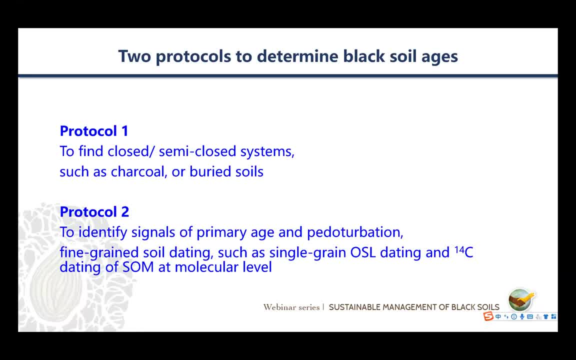 grain soil dating, such as single grain OSL dating and 14, carbon 14 dating at a molecular level, which by now, by the way, is now possible. Two days ago there was a report on this, on this technology. 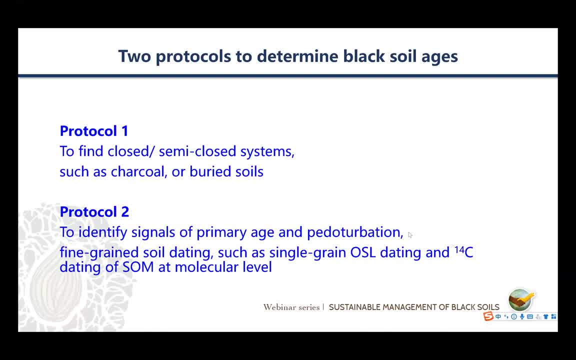 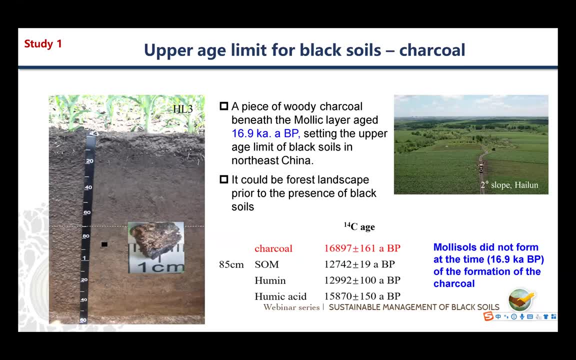 Well, given these hypothesis, we need to find the right location to to start this. Fortunately, we, after extensive survey, we in North East China. we investigated many soil profiles. In one profile we found a piece of a wooded charcoal. 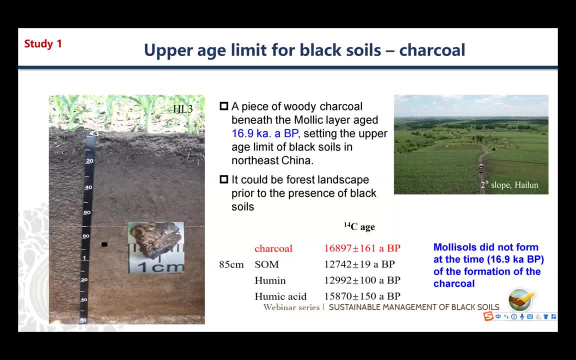 which is beneath the molecule layer And we dated this charcoal: It is about 60,, 16,000,, more than 16,000 years before present And and it it is buried below the molecule layer. So we can harvest is the formation of this black soil is. 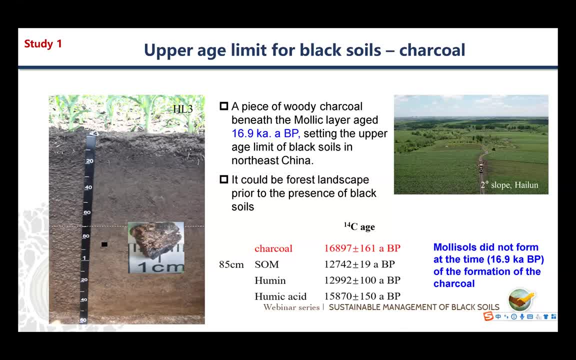 after this time And we also dated the carbon 14 age, The. the age can be from soil, organic matter in bark samples or we separated humic or humic acid. So we found that humic acid, carbon 14, is a little bit older than the bark soils. 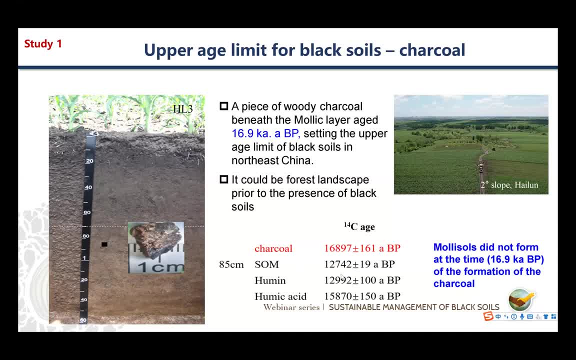 which means if we have to use carbon 14 age, we better separate this soil organic matter into different components And then we can use the old part. We need to testify this in more cases. We still need to do that in the future. 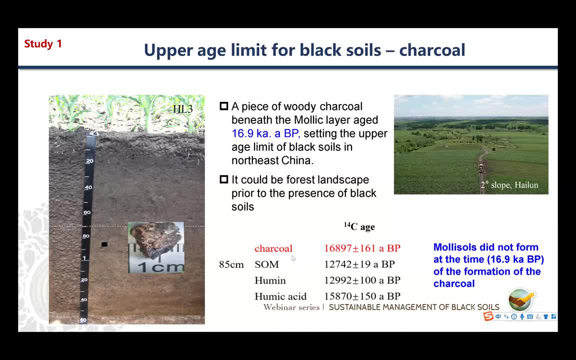 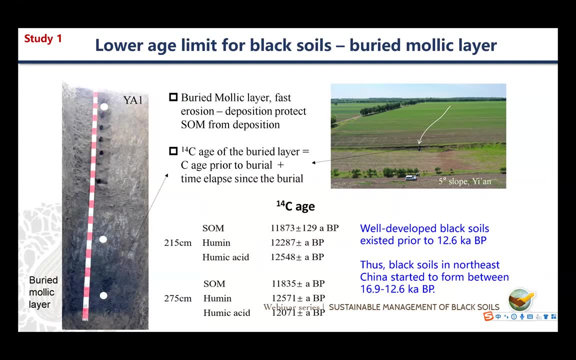 So this is the first we defined as the upper age limit. It's about 17,000 years. This is well. in another place, or actually in several other places, we found that we found that buried molecule layer, black layers- 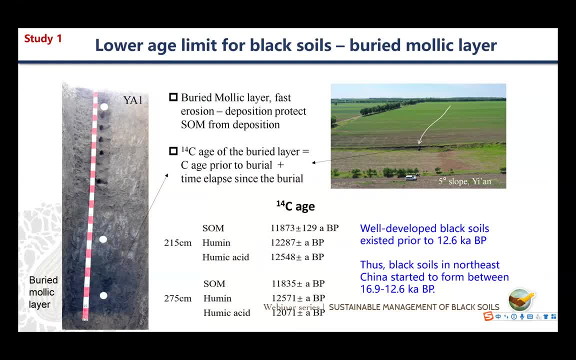 That is, they formed in a different is in a previous stage, which is buried by the current service soil because of a deposition, a certain erosion and deposition, And we we we sampled the buried soils in two depths: One is 215 centimeter. 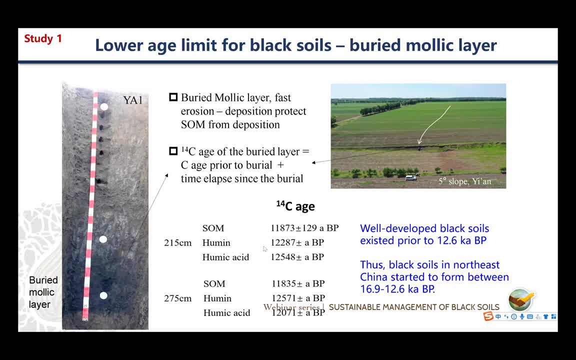 another 270 centimeter, And we did the carbon 14, which is about 12,, 12,000 years ago, And that means in this area the black soils was formed before that, before that. So that is by combining the 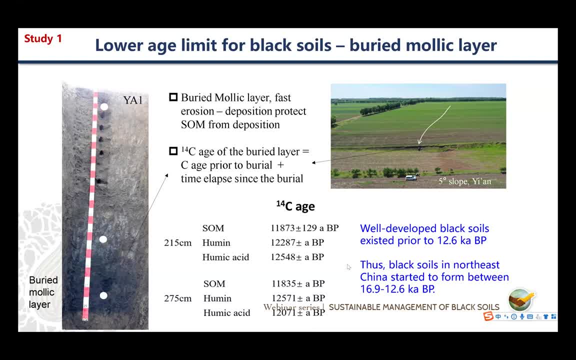 the previous slide. we, we can, we can say in Northeast China, black is black. soils started to form. started to form between 16.9 to 12.6, before present, This is to our knowledge, is the. 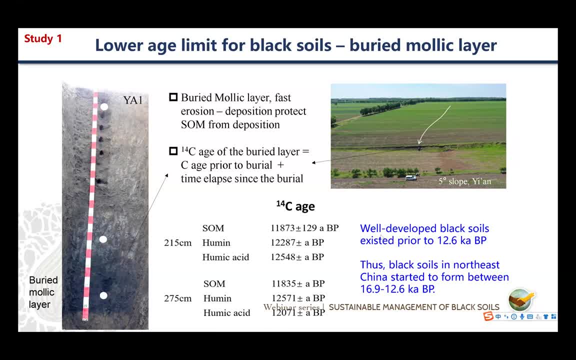 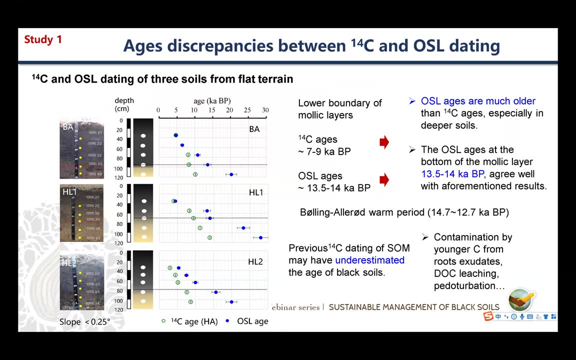 is the first solid evidence to show the very initial initial formation time of black soil in this region. Well, we also studied several other soil, soil soil profiles and we found that there are discrepancies between carbon 14 and OSL dating. 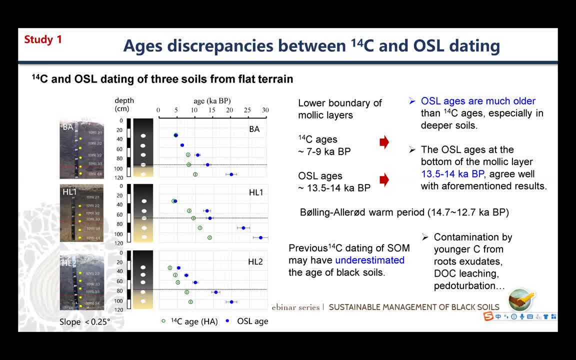 OSL dating is used to date the age of the parent material. So it's not for the, for the organic carbon. We see discrepancies, as you may see in all those profiles: the, the blue point, which is OSL date. 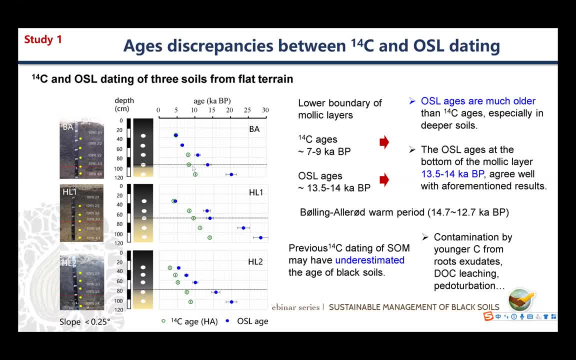 and the green point is organic date. There are also there. there is always a discrepancy between these two age Well and the OSL age always older than carbon 14 age And then OSL age at the bottom of the black layer. 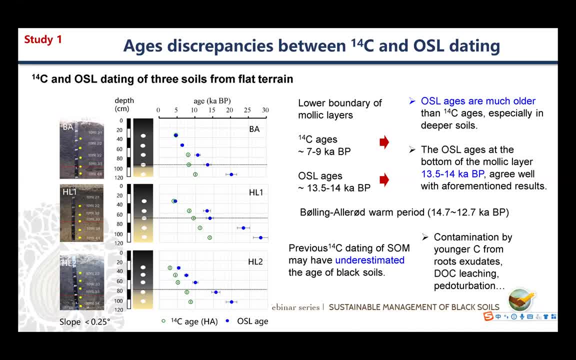 the old molecule layer normally is 13.5 to 14 ka, which means the deposition of parent, parent material started at this, at this time. So so this, by using this, this data, we have established a kind of framework for the. 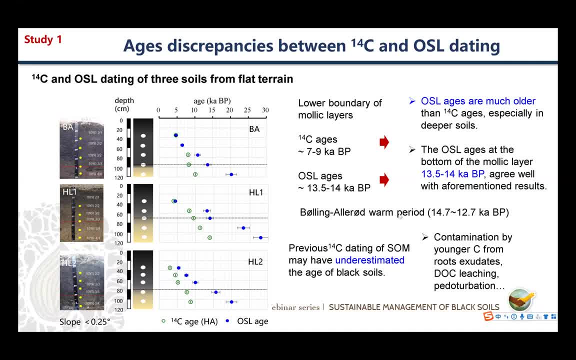 to understand the formation time of black soils in northeast China And we compared this kind of study with with very few studies from other parts of of the world And- and they are actually- then this study is really scale in. 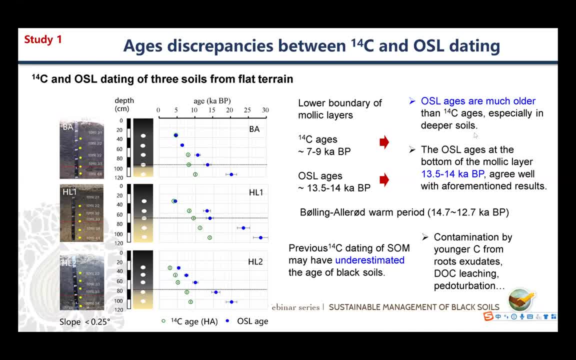 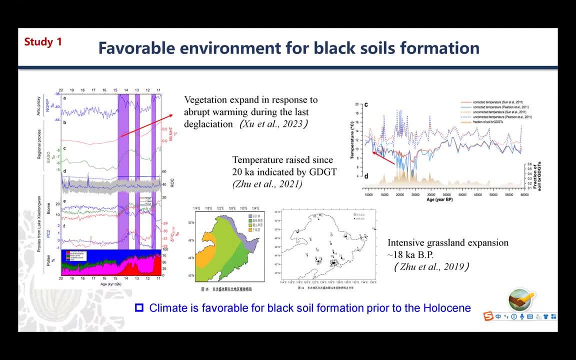 scales in in currently, And this period is in geologic term, is between Boolean and Elorot warm period It's it is 14.7 to 12.7 ka before present. So and we 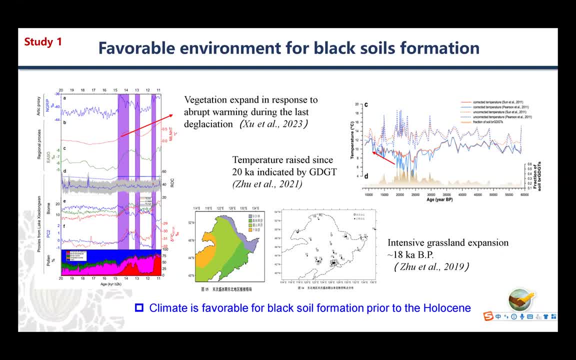 we have evidence from contemporary geology of this area. There are several, many other studies, many geological studies, contemporary geology studies in this area And it is to show that during this time, after 20 ka, the temperature in this region rests. 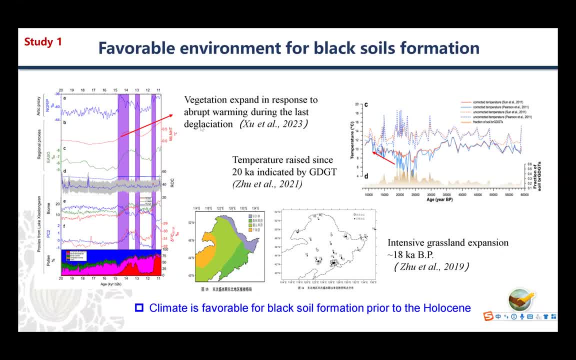 gradually And the vegetation started to to form and responded to the warming and it does last after the deglation. So so, and also there are studies show that after during 18 ka, before present, there was a grassland expansion in this area. 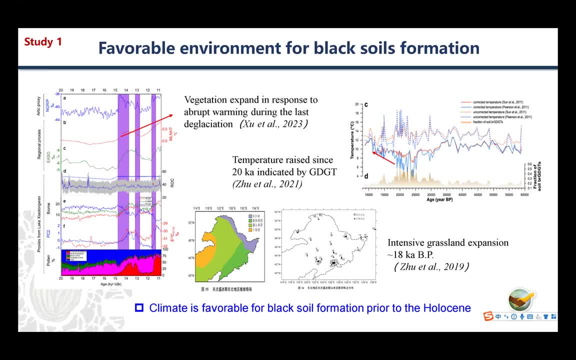 according to the, the biological, the, the, the botanic, botanic history study. So that means climate is favorable for black soil formation prior to the Holocene And the the formation of of black soil is much earlier. 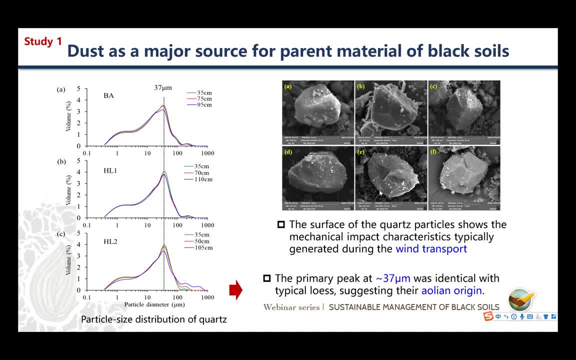 than Holocene time. So we have also studied the parent materials of this area. the area It's. basically it is loose loose. We. we see there, there, there. particle size. distribution of the of of quartz. 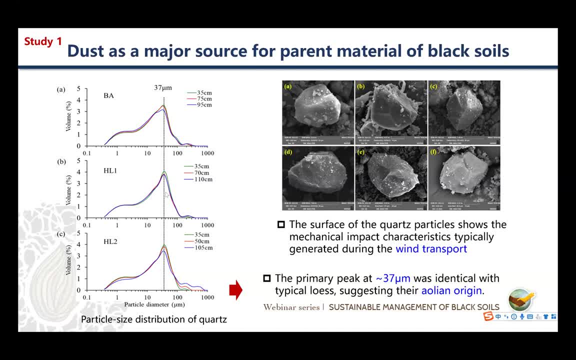 And I see there we we have in most in different profiles we have always the peak, a peak around 70,, 37,, 37,, 37,, seven meter. So this is a typical loose deposition And 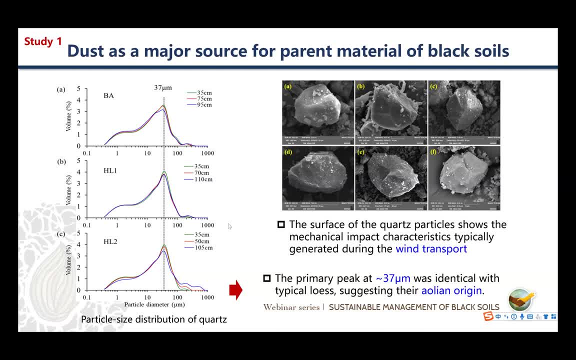 and it is formed by, of course, by wind transportation. So so this is we. we, we show the the deposition of the loose as material, material basis of black soil, And by calculating the 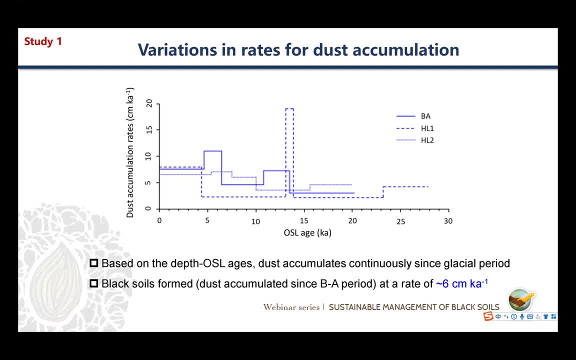 edge difference and the depth difference we can. We can calculate that the black soil in this area has an average rate of about six centimeters per thousand years, which is well. at least it's science-based data on the formation rate of this area. 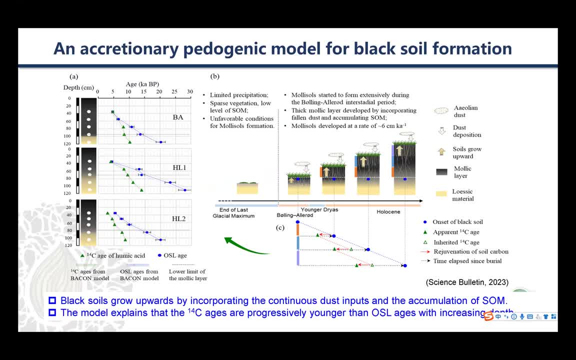 Well, as mentioned earlier, the buildup of black soil is an accretionary model, So that means the soil is built up and meanwhile the organic matter started to form. And because of time limit I have to go a little bit quick. 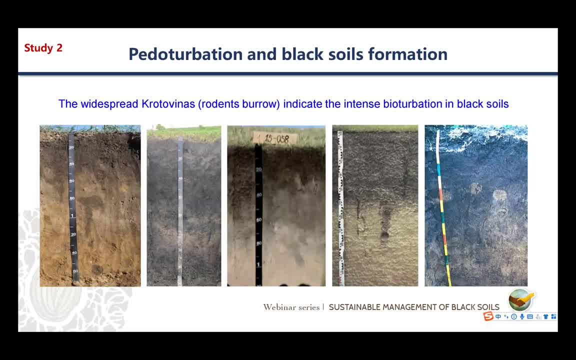 So there is another study we focused. We focused on the bioturbation process or pedoturbation process, because in black soil we have widespread cortovenous, which is a relics of rotten burrow. So there we see these pockets of either black or white materials, which is a mixture of soil materials from another soil layer. 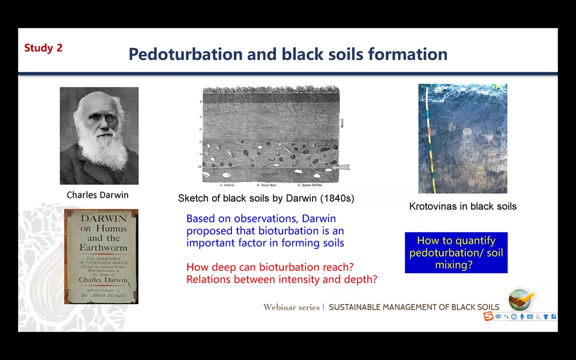 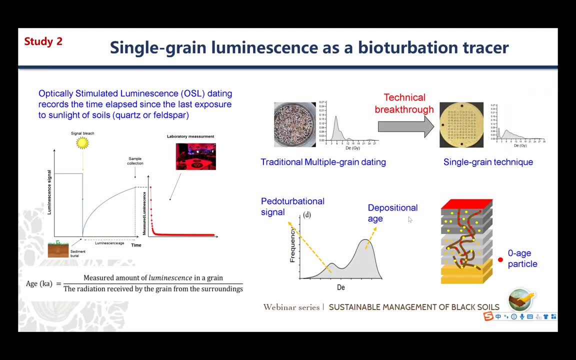 So this is a long note. This is the oldest evidence, as we can trace back to Darwin, Charles Darwin. He showed the sketch of bioturbation almost two centuries ago. So how can we determine, how can we calculate the rate or the ratio of mixed genes? 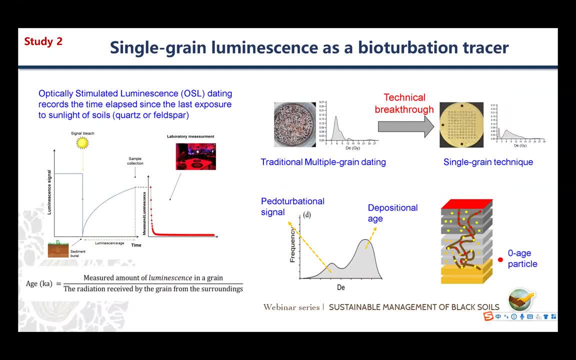 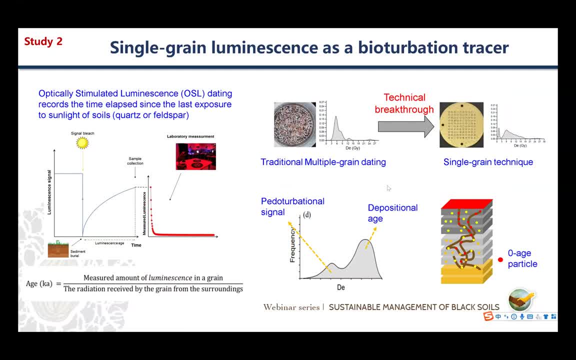 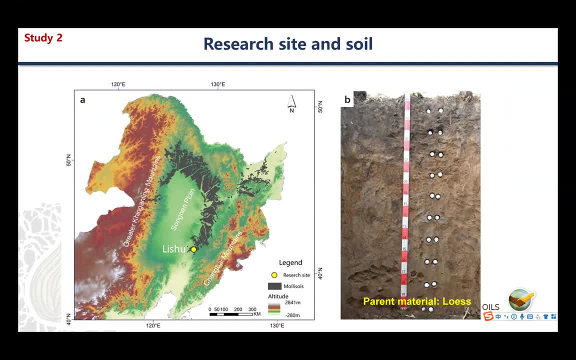 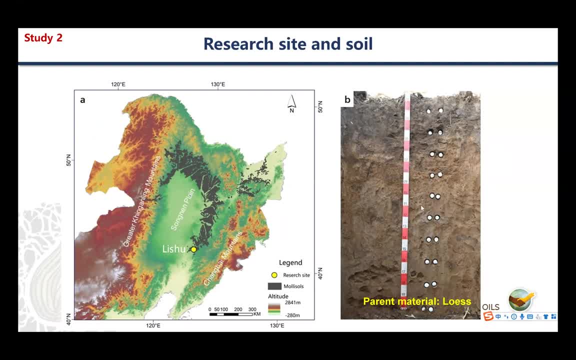 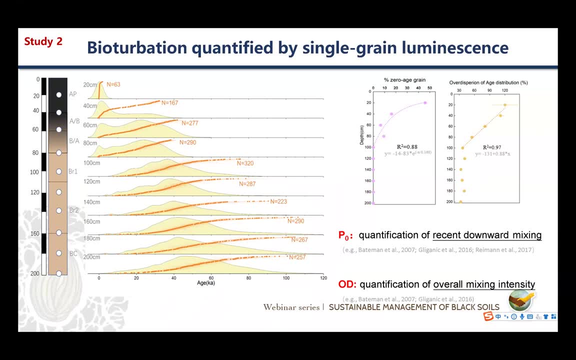 This is the southern boundary of black soils in China. So we sampled the horizontal soil of soils, And for each soil we separate 600 grains, either quad-grain or fed-spot grains, And then for each horizon we got 300, almost 300 age data. 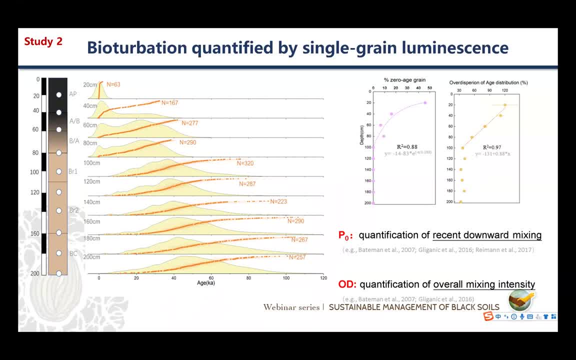 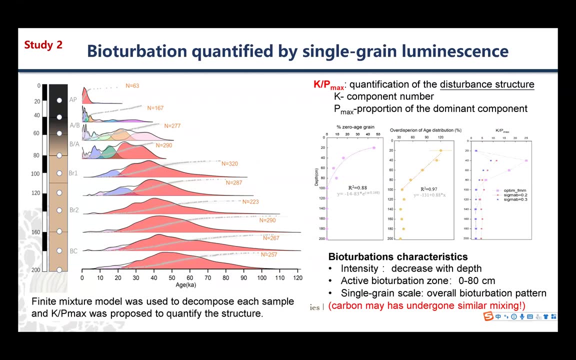 and which we can make a distribution of age of these grains. And by using finite mixture model, we can decompose each sample And we, by establishing indicate K over P max, which can show the disturbance structure, disturbance ratio of horizons. 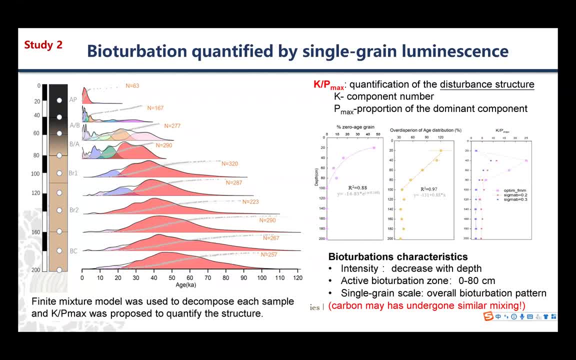 And in general we see the intensity of bioturbation decreases with depth And the active bioturbation zone is, for example, in the surface, 80 centimeter, and below that we had really no bioturbation or very little bioturbation. 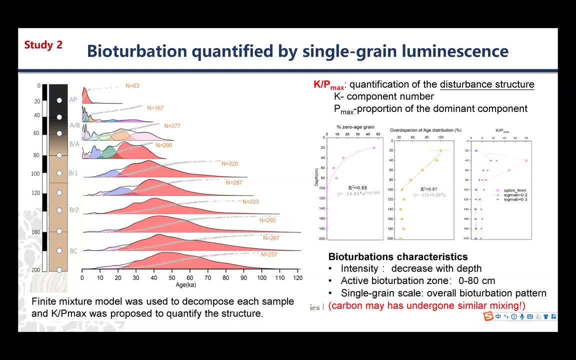 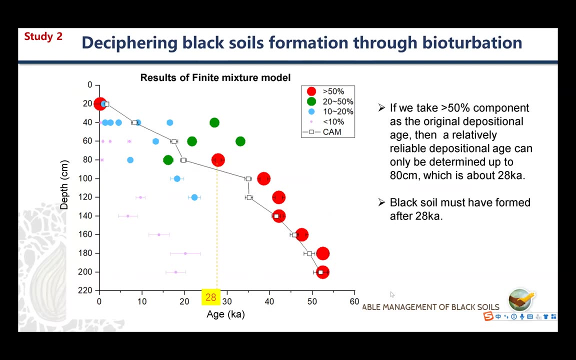 Actually, it has no current bioturbation. We can quantify it for each layer. above that, how much soil material is mixed with bioturbation? This is the very well new data and I use very cutting-edge technology to show this- and we we, if we give a criteria of fixed 50%. 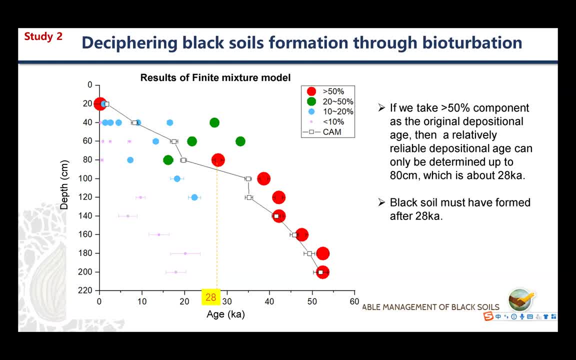 of original soil particles as a, as a, as a threshold, we can again see that over the surface, in the surface 80 centimeter, we have really a mixture of different sources of material materials, which again means the bitubation process is so strong and below that most of the soil material is from the one source, from one. 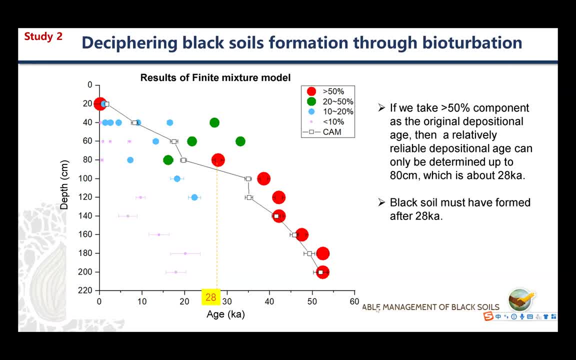 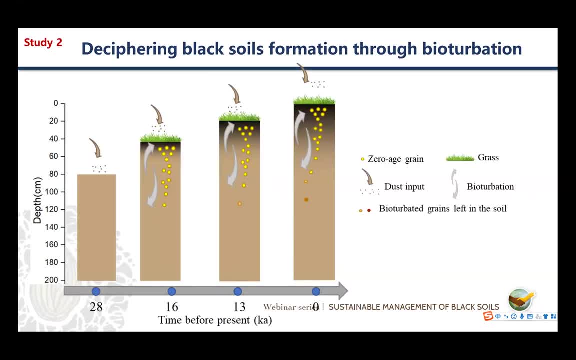 source, that means the little bitubation process occurred in these layers. so, to put them together, our study has shown that have shown that the formation model of blood soils in this region, First after the degradation period, with the advent of grass and the plant, 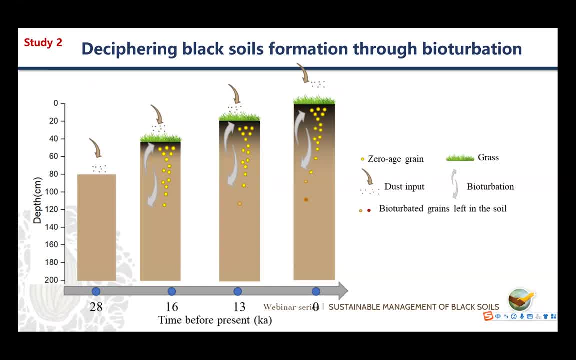 the soil, organic carbon started to accumulate. But in the meantime the dust accumulation continues and the soil has built up and the age of the carbon keeps older at the bottom. But with the regeneration process its value is always younger than the dust deposition age. So that is all the 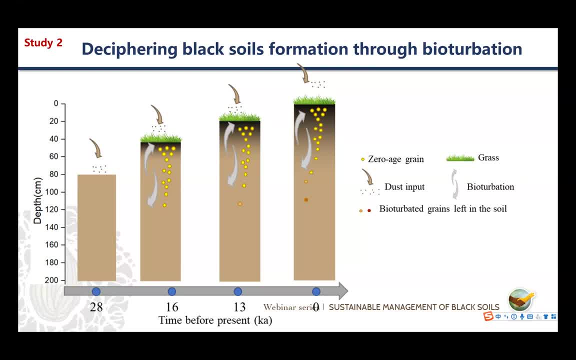 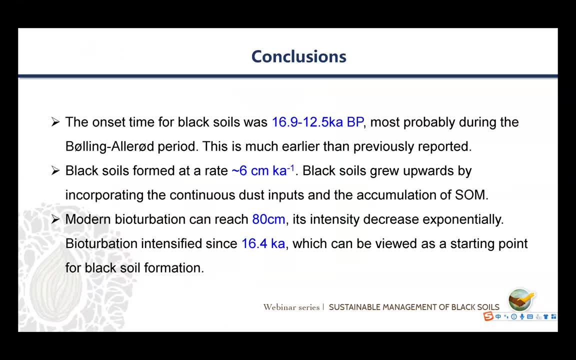 data we have just shown. To conclude, the onset time of black soil in North China is between this period, most probably during the BA period. This is much earlier than previously reported. The formation rate is about six centimeters for thousands of years. The modern biotubation 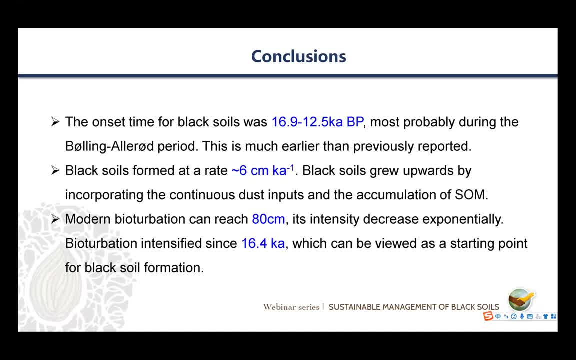 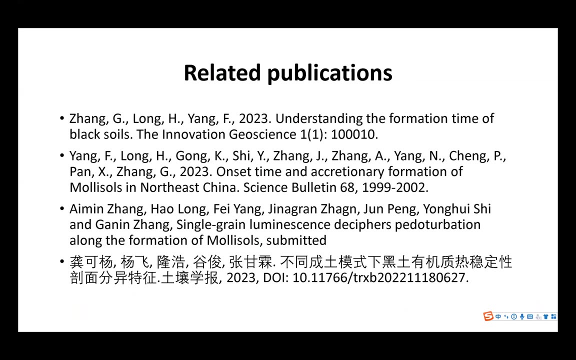 can reach up to 80 centimeters and its intensity decreases exponentially with the depths. So the biotubation intensifies since that period and which can be viewed as a starting point for the formation of black soils. So we have several publications to support this presentation in the innovation geoscience science bulletin and one. 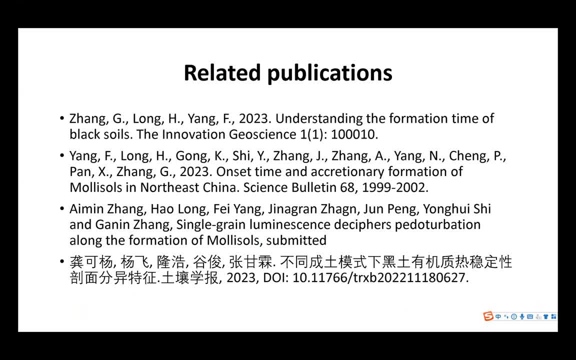 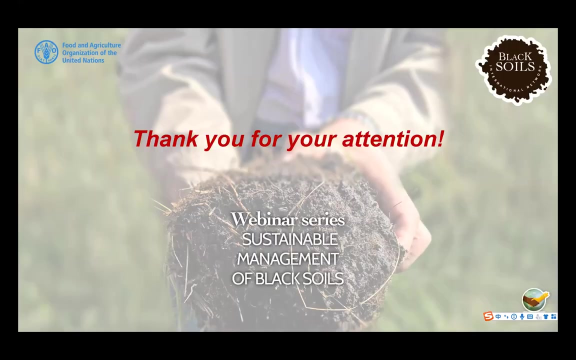 submitted to a very prominent journal on the OSL dating. So my colleagues Dr Long, Dr Yang and others also joined this study. For this I conclude my talk and thank you for your attention, Thank you. Thank you very much, Professor Zhang. Thank you very much for your. 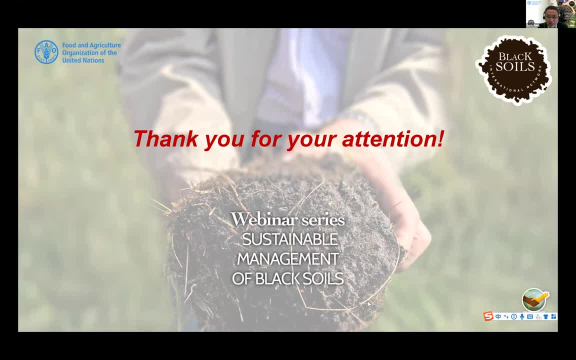 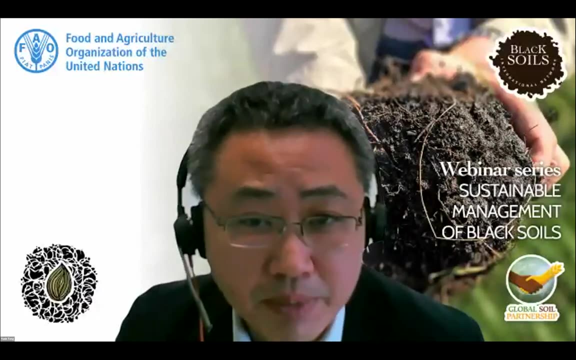 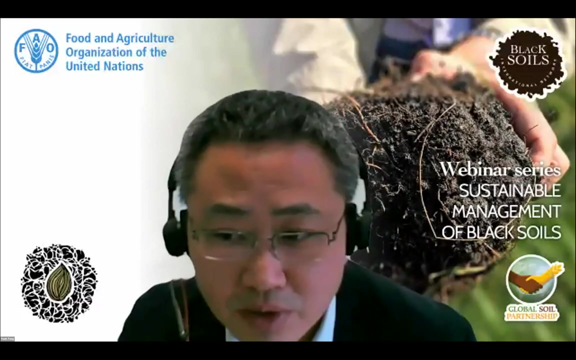 informative presentation. You explained to us how to formulate black soils and we know from your presentation. I also improved my knowledge about black soils. For example, to formulate black soil six centimeters will cost one thousand years, So it's so difficult to have black soils. 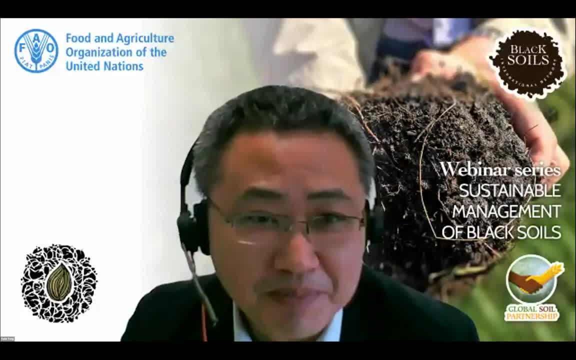 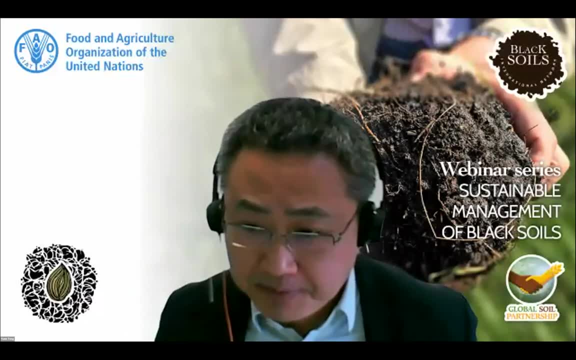 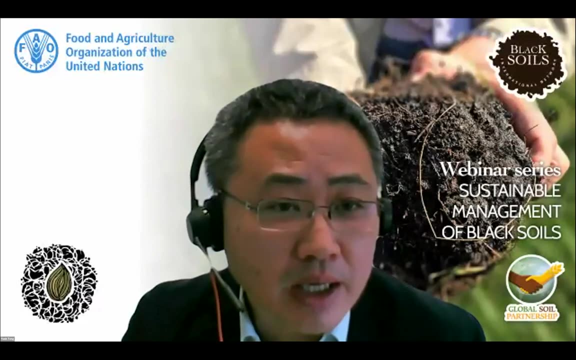 and for our human being. we are so easy to degradate black soil, So we must protect black soil and we learn a lot from your presentation and a lot of participants. the audience asked about the sharing of presentation, So we will upload the presentations of this webinar on our website So you can go to our 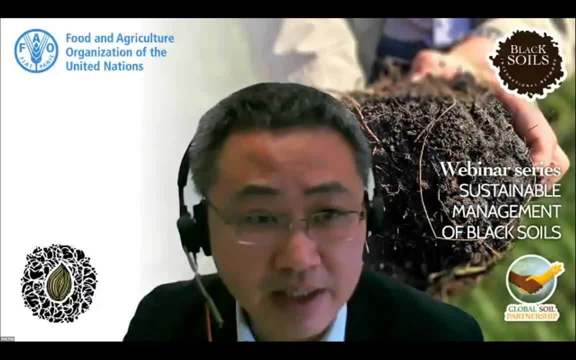 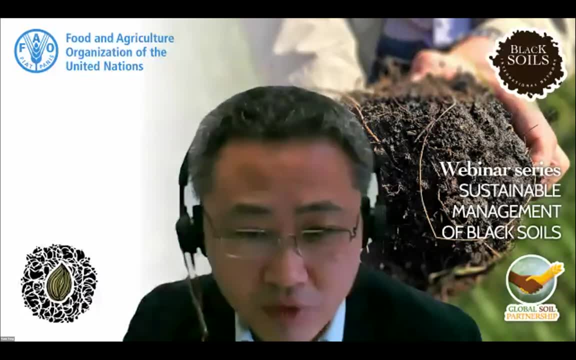 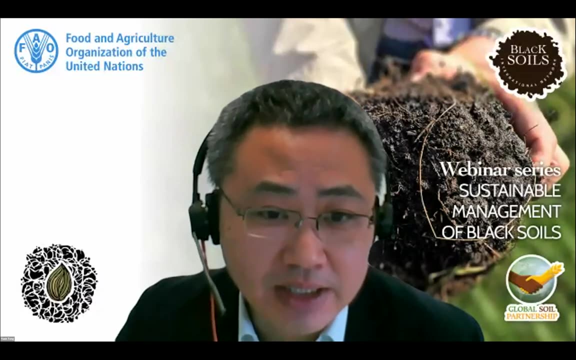 website to review the presentation, because I think we need some time to digest the knowledge from Professor Zhang. thank you very much, professor zhang, and without the further ado, uh, now i would like to invite the second technical presentation from professor jen tushong from china agriculture university. 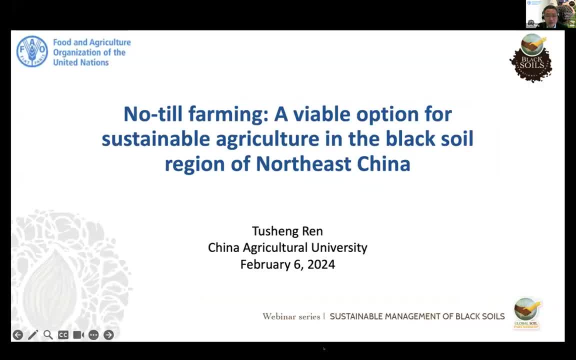 professor yen, the floor is yours, please. thank you very much. hello, dr tony. can you see my screen? yes, very clear. thank you please. okay, thank you very much. hello friends and colleagues. it's really a pleasure to be here to uh share some of my views on the black soil in china. this time i have been working in black soil. 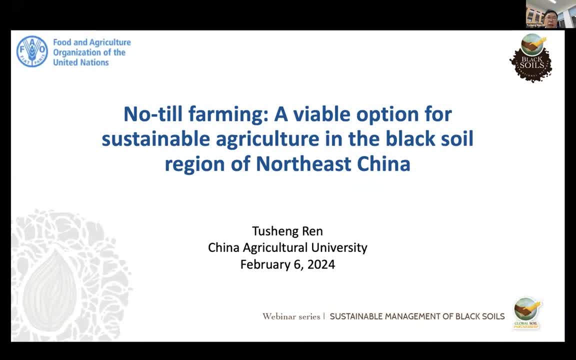 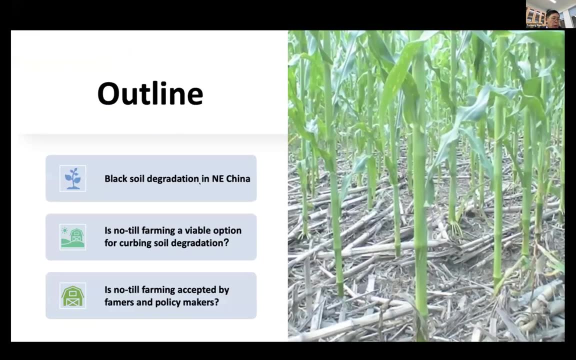 regions for the last 16 years. so today i want to show what i have learned there and about the technology of no-till farming for sustainable agriculture in this region. i will briefly introduce the status and drivers of black soil degradation and then present some of the results for our long-term no-till farming studies. 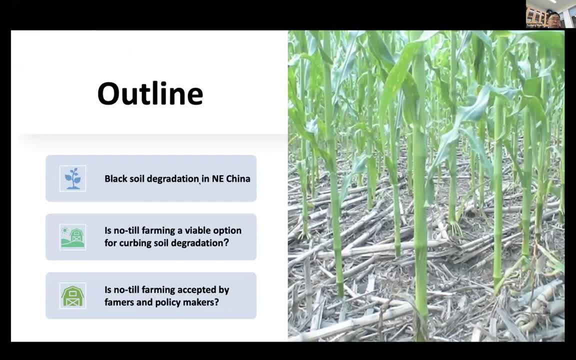 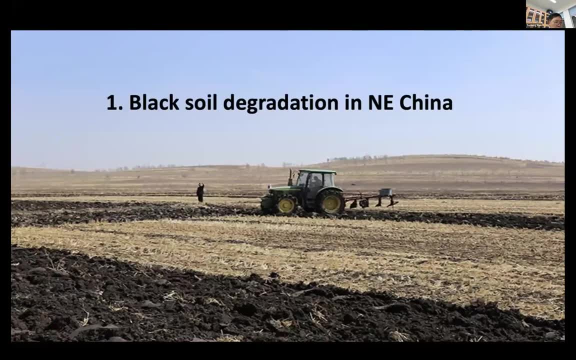 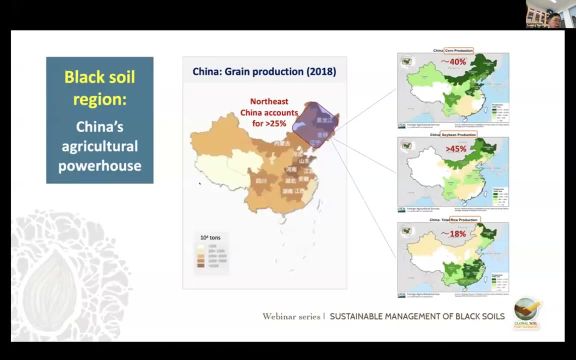 and finally show the responses of farmers and policy makers to the no-till farming system. first, let us have a look about the problems with black soil and how the crisis occurred. as has been introduced by the chair, the black soil region of north china is one of the most important cornerstones for china's food security in 2018. 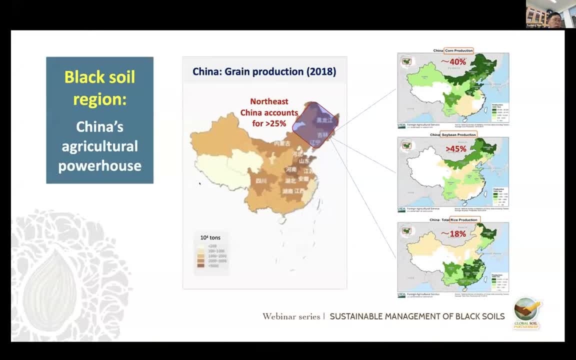 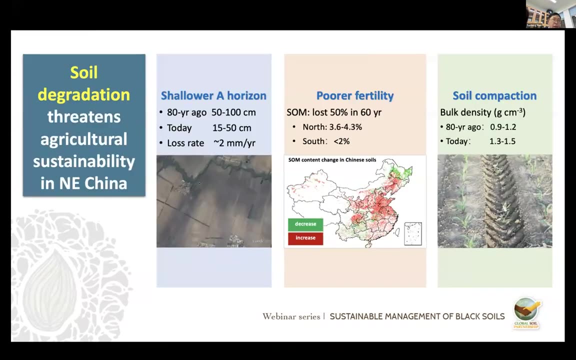 it produced more than a quarter of china's national grain. that includes about the 40 percent of corn, more than 45 percent of soybean and 18 percent of rice. however, over the past 50 years, the black soil has been threatened by the intensive farming systems. 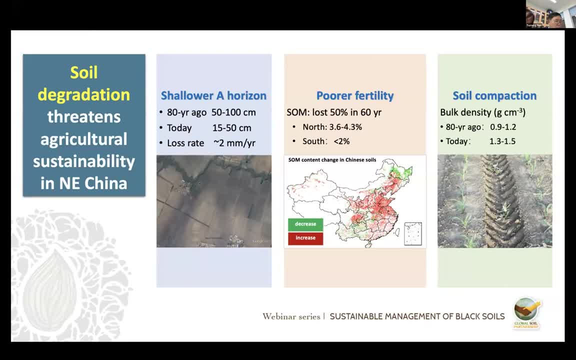 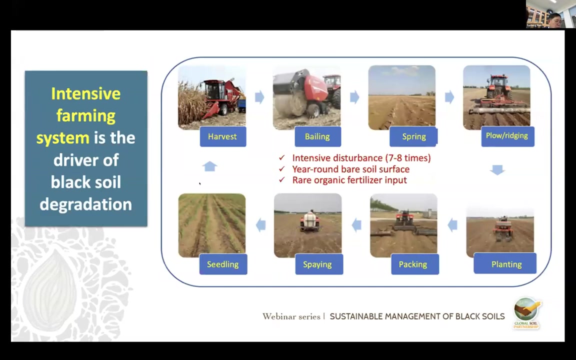 currently the top black soil layer is being lost and reached about two millimeters a year, and about 50 percent of the soil government has been lost and some soil compaction is now becoming a key constraint for crop production in this region. so this is a description of the current 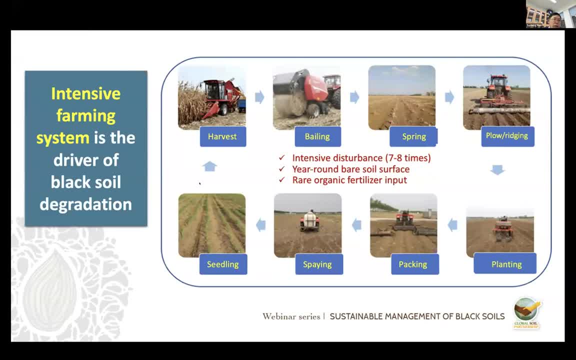 intensive farming system. uh, as you can see here, that crop, uh literature is brought or taken off from the field, leaving a bare soil- service in hui guanxiang year. and also the soil are killed several times, which leaves a loose surface layer. and during tillage times, uh, the soil aggregates were destroyed and the soil organic matter was decomposed. so 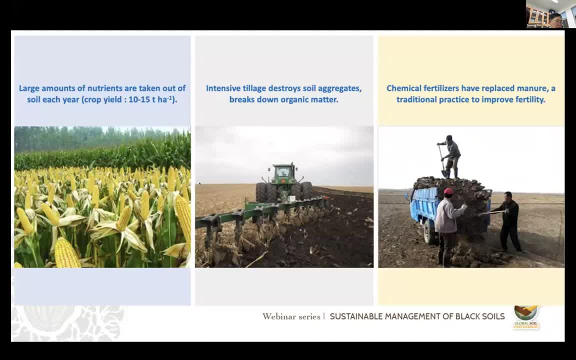 that's really a little degradation. at the same time, each year, you know, after crop harvest, a lot of the soil nutrients have been taken away from the soil. another thing that the traditional practice uh applies a lot of manures in soil, but today farmers have replaced the manure with chemical. 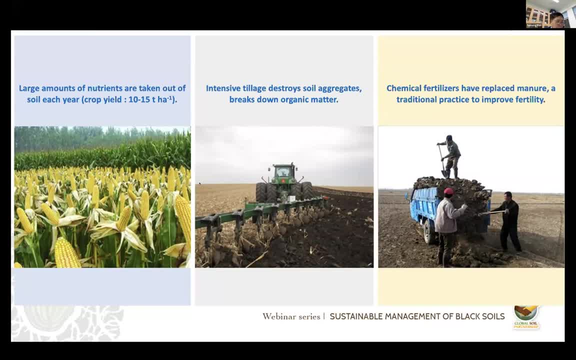 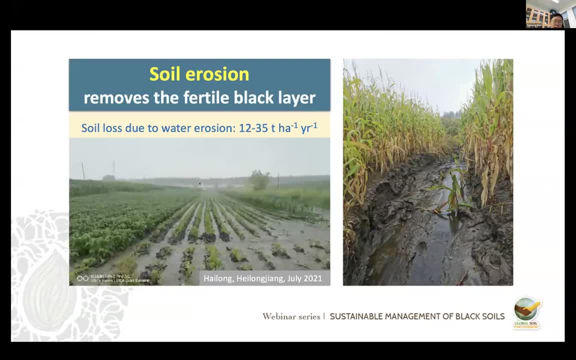 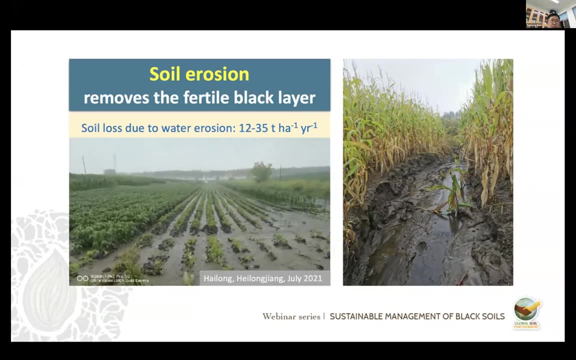 food and iron, so that's uh makes a lot of difference. so, as a route, the severe soil water erosion occurs in the summer, as you can see here. this was uh recorded by my uh friend in helenja province. you can see that. you know uh they have uh. 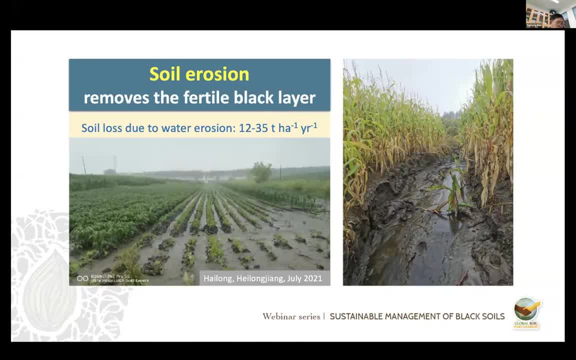 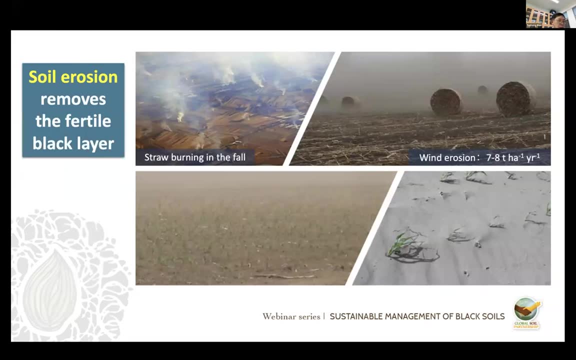 estimated that. you know you're in the sloping areas. black soil had lots of uh loss, uh as high as 12 to 35 tons per hectare a year, and also the uh because of the bear and loose tower soil. dust storms strikes the region several times in spring. 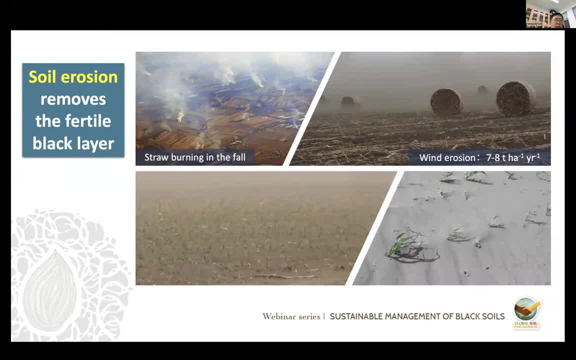 on average, the soil loss due to wind erosion is around seven to eight tons per hectare per year. so it is quite often that wind also hurts or even kills the young plants in spring and early summer, some periods, as you can see here. well, a lot of plants have been killed here. 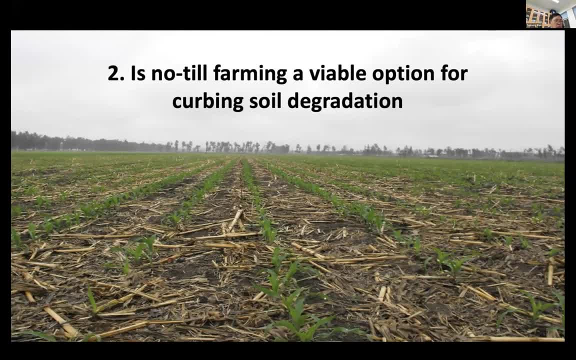 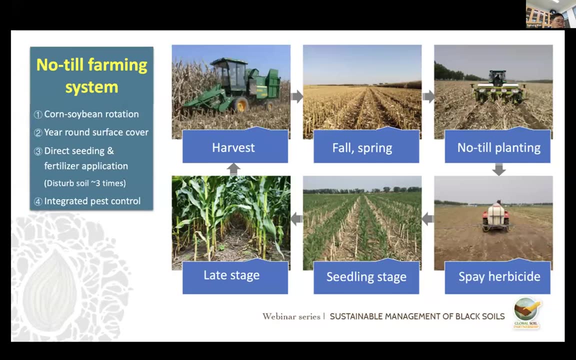 so, uh, 16 years next. i want to show you that the no-till farming is very effective in covering the region and enhance agricultural sustainability in this region. 16 years ago, we started to introduce no-till farming in north china. so, compared to the traditional farming system, the new system- 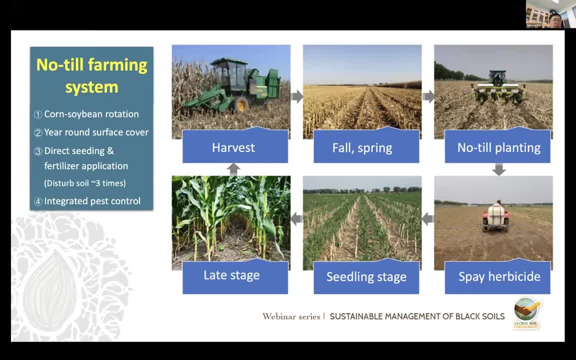 makes some changes in the farming practice. let's include the crop rotation, year-round surface cover with crop relative and during seeding and finally they integrate the past control. so in this system the soil disturbance is reduced from seven to eight times to three times and the soil is protected with crop relative uh year-round and a large amount. 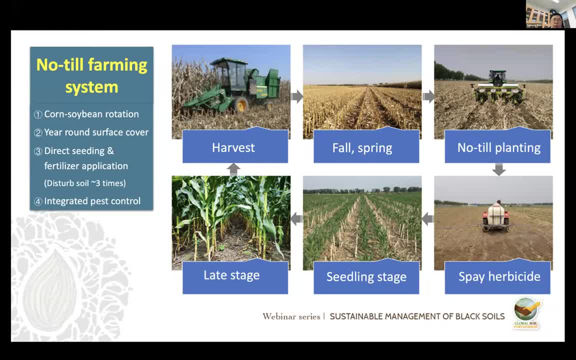 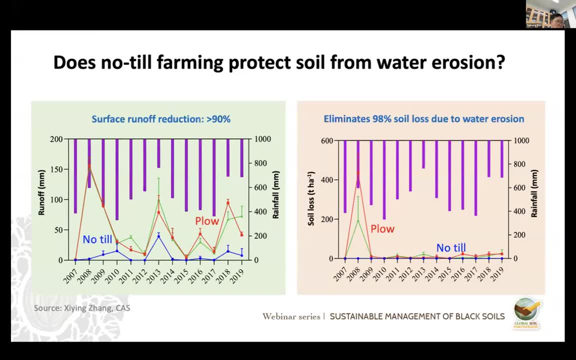 of organic material materials is retained to the soil. so this is our no-till farming system. uh, in next few slides i will show how effective the no-till farming system in covering the soil in black soil region of north china. first let's have a look of the uh? uh reduction of the soil. 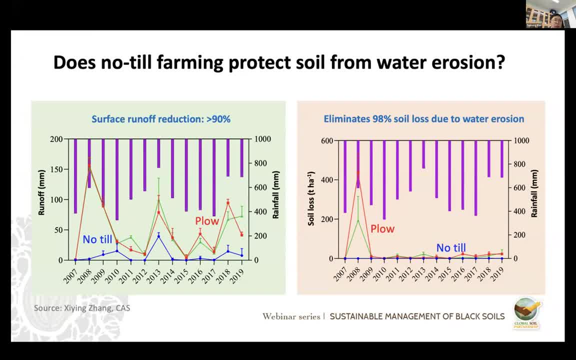 or water erosion. uh, this is a long-term study from my uh friend, uh from the chinese economy of sciences. uh, uh, they showed that you know uh, if you have the no-till farming system applied in uh in the field, uh surface draft can be reduced by ninety percent. ninety percent and uh a soil loss. 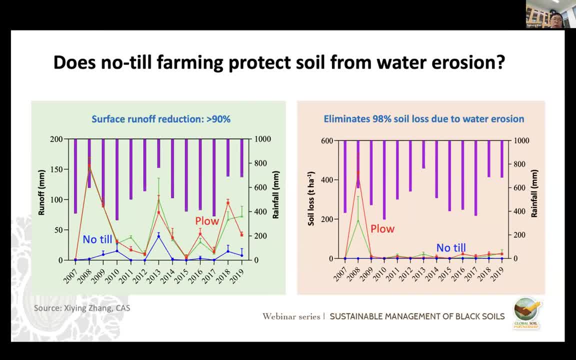 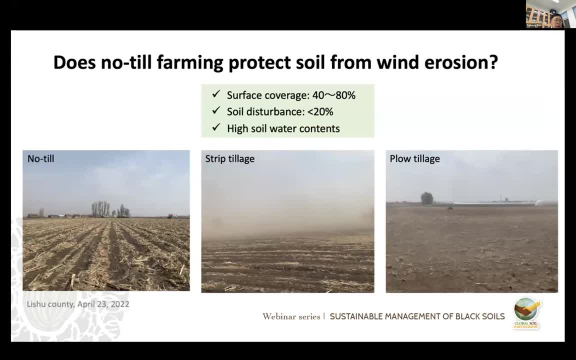 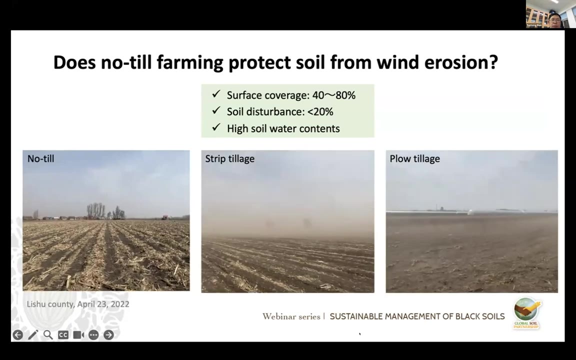 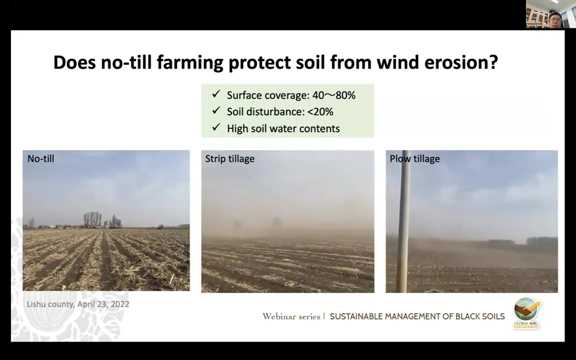 is almost eliminated, you know, due to the uh crop recovery and less disturbance uh. at the same time, uh uh, the soil only doesn't use reduced uh significantly. here i want to show you some of the uh radius we recorded in the field. so this video was the compromise students. you know they called it in two years ago. you can see that. 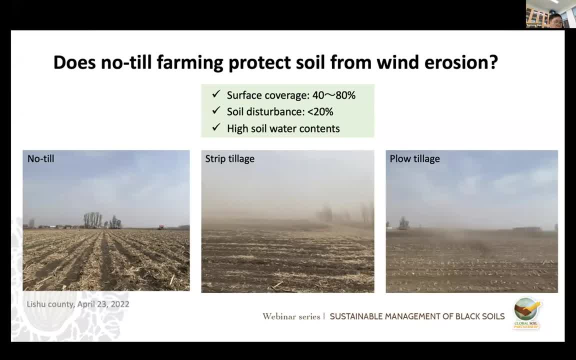 on the same field conditions, only yours in no-till plots, was reduced significantly because of the value cover and let's start the traverse- and also it has a higher water content. so the uh surface coverage: if you have a over 30 percent of surface cover, the surface cover is slightly higher than the. 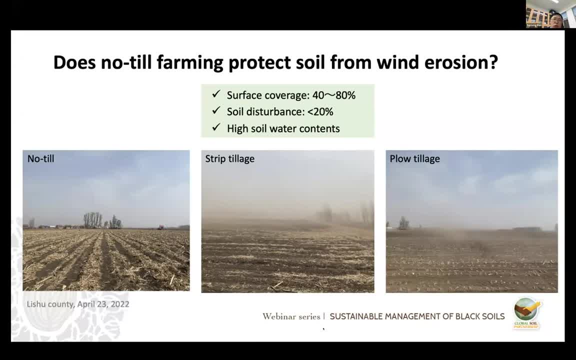 surface cover of the soil so it has a higher water content. so the uh surface coverage, if you have uh over 30 percent of surface cover, if you have over 30 percent of surface cover, So the wind can be reduced very effectively. This is my field: plots. 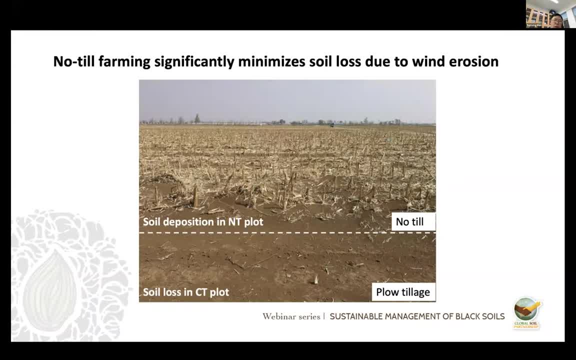 About. this has been done over 15 years. You can see that after 10 years okay, the no-till plots, the soil high surface is about five to 10 centimeters higher than the plotted plots because the wind had blown the soil to the no-till plots. 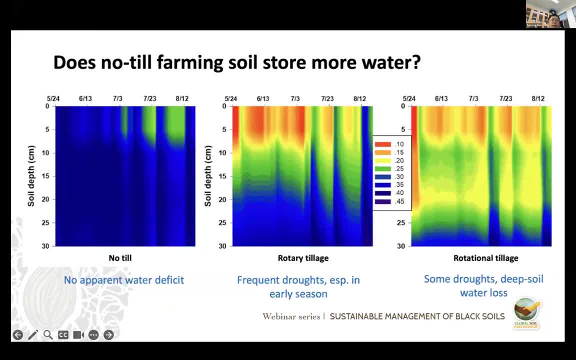 and the soil is deposited there. Sperm drought is often deletes core planting in much of the black soil region of China. So, on the no-till systems, this is not a problem anymore, because you can see here that the no-till plots. 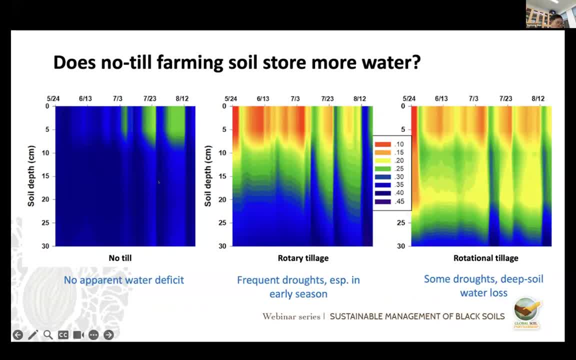 always have a higher water content and it's produced very favorable soil water conditions for planting. so there's no time to delay. But if you have a zotary tillage or zotational tillage, there always is a drought- delayed planting of coral. 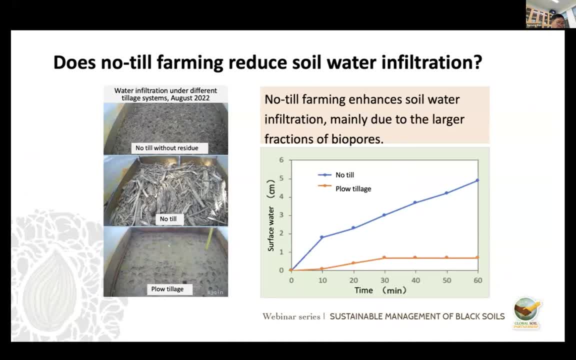 So in Northern China also, many people have been concerned about no-till farming because they are thinking that no-till farming will reduce soil water infiltration and soil water storage. Here, after 10 years of no-till farming, we can see that no-till farming did not reduce. 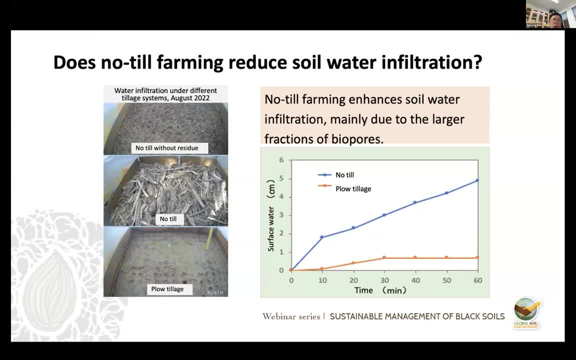 the soil water infiltration. But the problem is and has been that the director's and sector's- but actually the increase started apparently. So after about 60 minutes the surface water on the teal plots is about five millimeters high, but for no-teal plots it's only 0.7 centimeters. 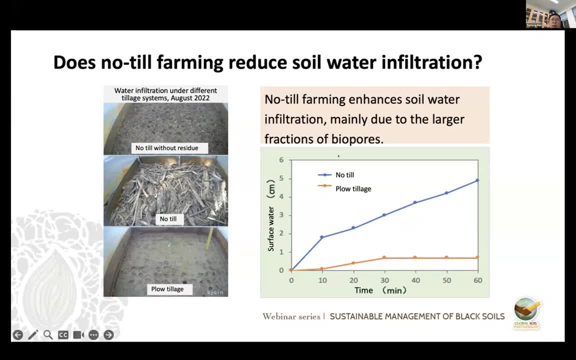 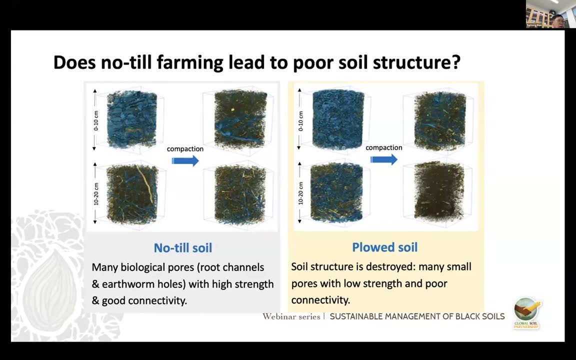 So the no-teal farming you can't solve water infusion, because the infusion rate is about seven times higher than the plot-heated plots. Also, we did some micro-seq studies about the soil structure. It showed that anti-plots have many biology pores. 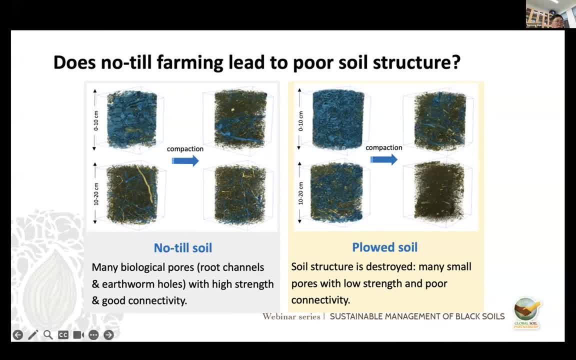 You can see that here anti-plots have a lot of biology pores And also after compaction the pores can still stand there, so they can resist the compaction. But for the plot-soil there's not many of the bio-pores and the micro-pores. 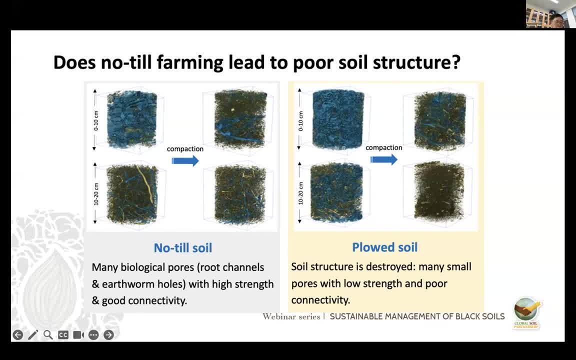 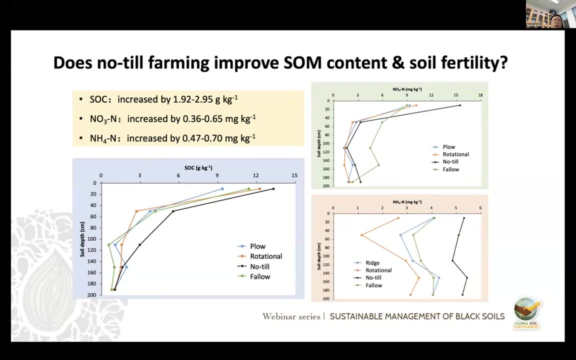 So after compaction a lot of pores have disappeared. So it's really that no-teal did not lead to poor soil structure, but it's an important soil structure. So another thing that if no-teal increases soil fertility- here I show you some results. 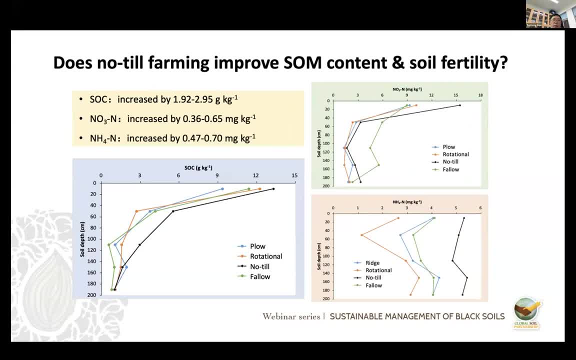 of this. This is a picture of our soil gathering carbon and also nitrate and ammonia. You can see that it's a black line. okay, The no-teal plots always have a higher soil gathering carbon in the soil profile and the nitrate is quite higher in the surface layer. 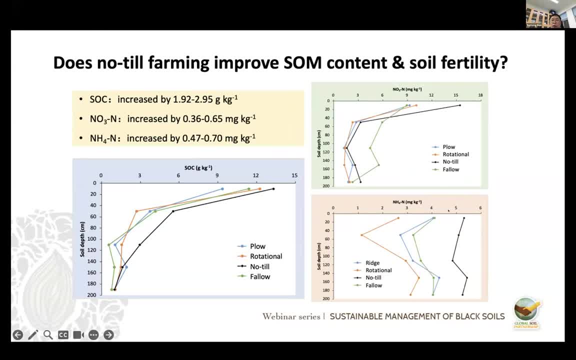 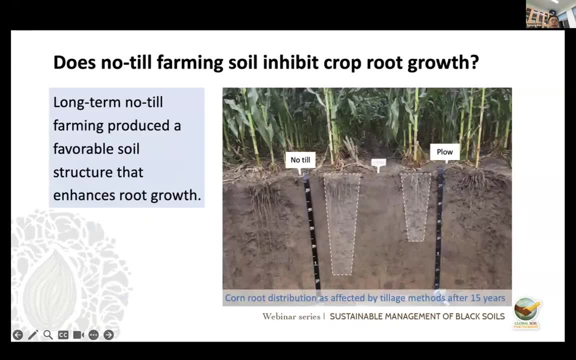 And ammonia is the most apparent change. you know, throughout the soil profile It always has a higher content of ammonia. So this slide shows the. So this is a picture from my colleagues from the Chinese Academy of Sciences. you know It shows that core root distribution in the soil profile. again after 15 years of no-teal. 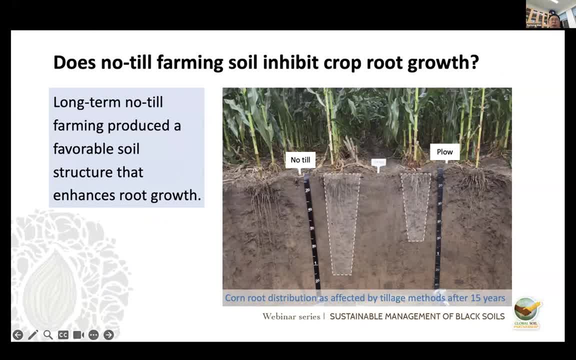 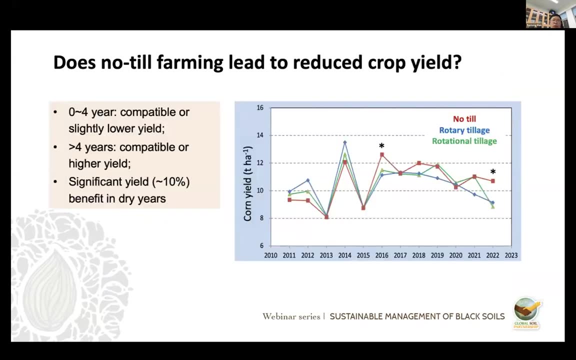 the crop root system is becoming deeper and also larger compared with the plot-teal system. So that means that no-teal farming really enhances the root development in the soil profile. So this slide shows the crop yield in my long-term studies, you know. 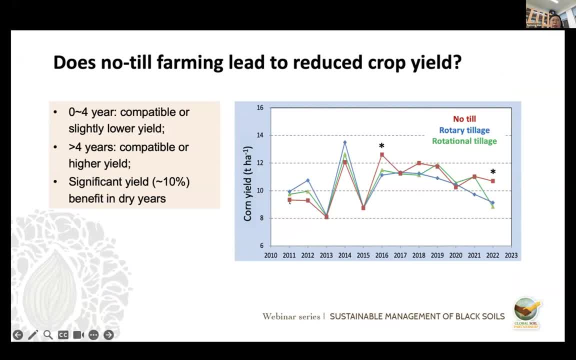 We started this experiment in 2011.. And over the last 12 years you can see that generally no-teal did not reduce the crop yield significantly. In the early few years, like four years or five years, there's some unstable yield. 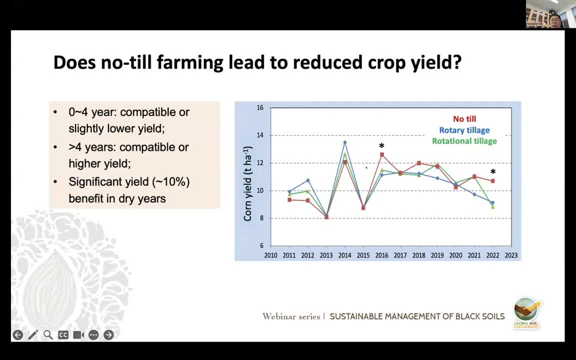 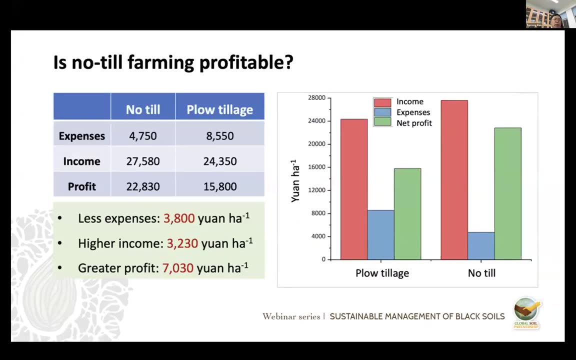 Sometimes higher, sometimes lower, But after about five years, no-teal, always have compatible or even higher crop yield than the conventional seeding system. So In two years the crop yield is significantly higher than the other systems. The other thing, that about the economic profit. so in terms of economics, because of the less 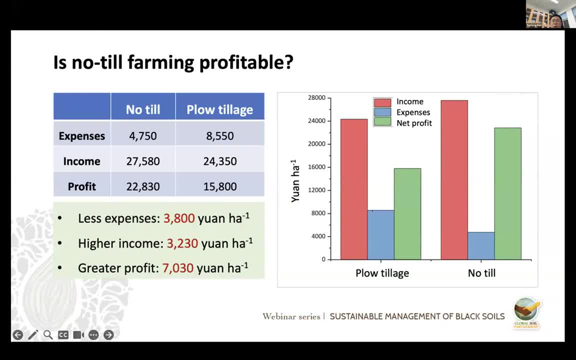 input here we have. okay, This is input in blue And this is income. you know, because you can see that no-teal have a higher income and less input, So the net profit is higher. Okay, We do some calculation in our field, okay. 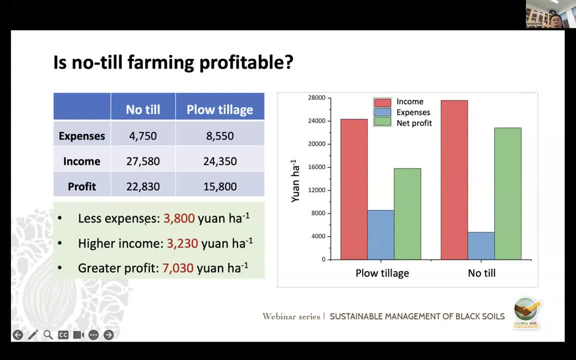 So the input is less than 3,800 yuan per hectare And the income is higher, 3,200 yuan higher, And so the net income of good profit is about 7,000 yuan per hectare, That's about 1,000 US dollars per hectare. 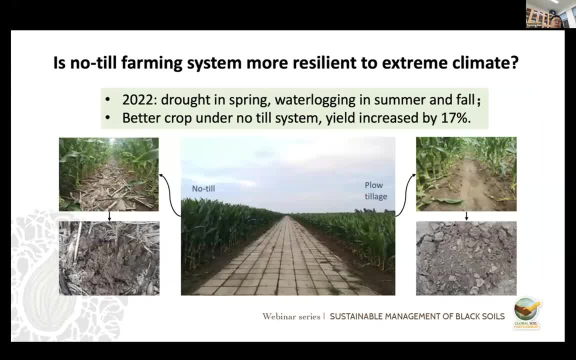 So it's really profitable for the farmers And also the no-teal crop system increased the resilience of the crop system In 2022,. we have a drought in the spring and two times of the rains in the summer and fall. On this extreme weather conditions, we got a very good crop yield in no-teal systems. 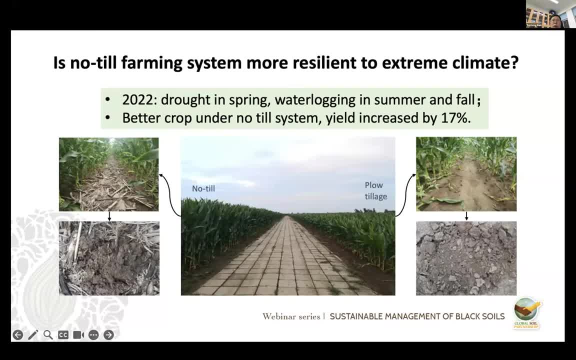 The crop yield is 70%, So we have a very good crop yield in no-teal systems. So we have a very good crop yield in no-teal systems. The crop yield is 70%, So we have a very good crop yield in no-teal systems. 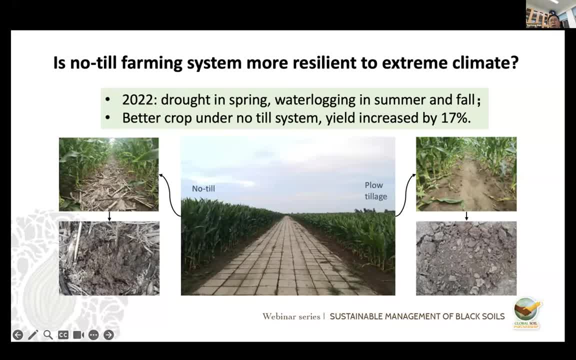 The crop yield is 70% higher than the plot yield systems. Actually, you can see from this picture here: this is our no-teal plots. This is the plot yield, plot-tilted plots, The crop: you can see the bottom cover, the color and also the height of crop of no-teal. 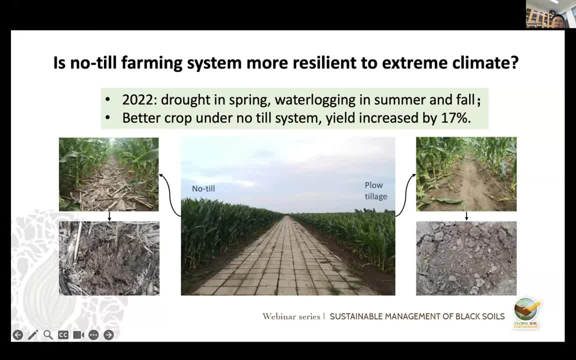 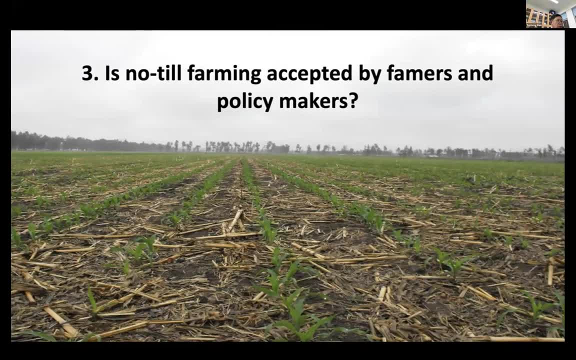 plots is higher than the plot-tilted plots, And also you can see the yellow leaves on the plot-tilted plots, So there's big difference here. Finally, I want to show you that I want to briefly introduce the. 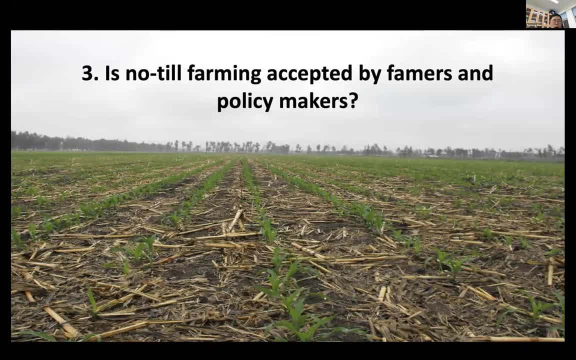 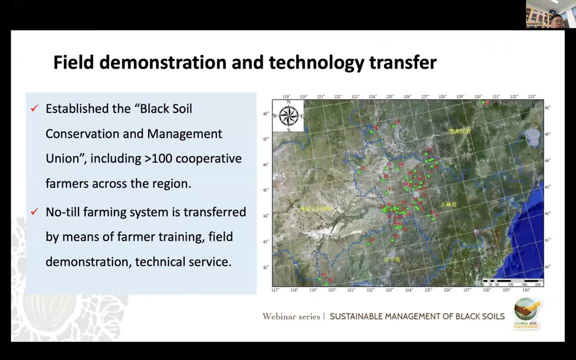 I want to introduce our outreach work on no-teal farming in Northeast China. Over the years we have established the Black Soil Conservation and Management Network in Northeast China. Currently we have more than 100 crop-teal farmers across the region. That means the farmer land is more than 100 hectares in this group. 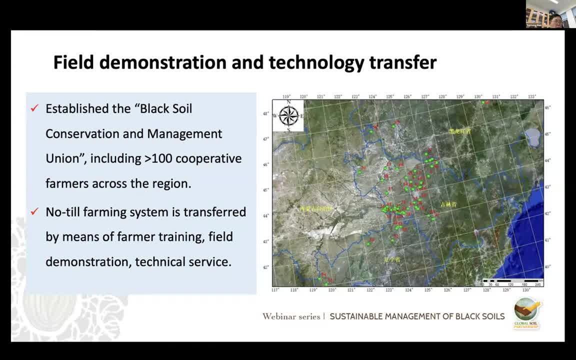 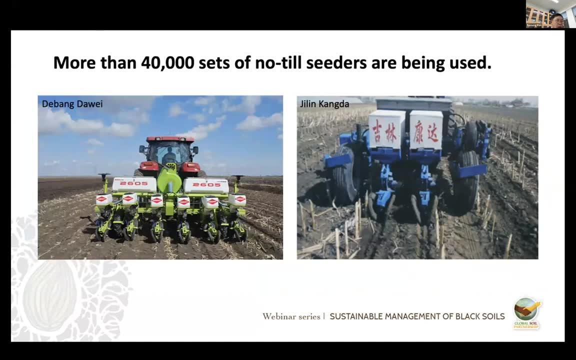 So we transfer the no-teal farming technology to the farmers by means of farm training and field demonstration and technical service. So this really enhances the intensity of the no-teal farming system in this region. I don't have an exact area about how much no-teal farming has been in this area, but 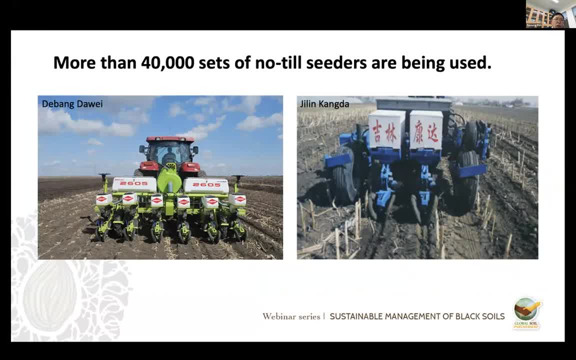 I know that we have sold more than 40,000 sets of no-teal seeders in this region. If we take a look at the number of no-teal seeders in this region, we have more than 40,000 sets of no-teal seeders in this region. 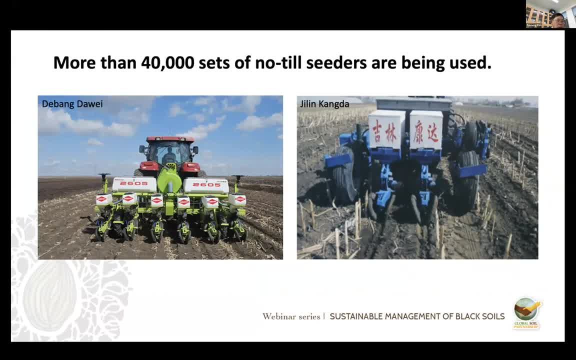 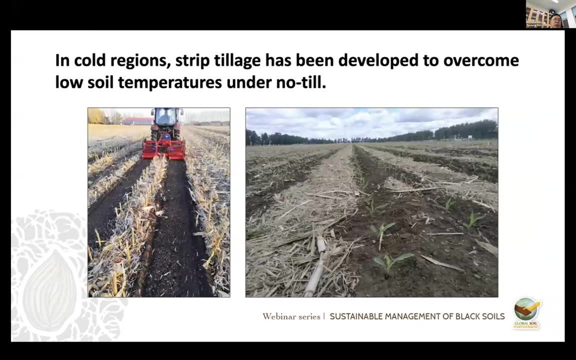 If we take 50 hectares per set and I think at the minimum we have about 2 million hectares of no-teal farmland. in Northeast China has been done In recent years. strip-tealage, which has about 50% of land, is no-teal-keeled here. 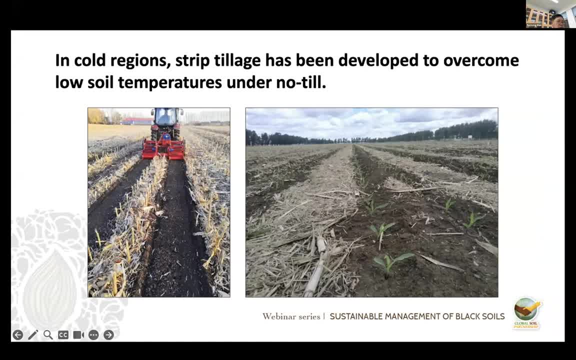 like this one, And the remaining 50 is anti-seed. Anti-seed has been widely accepted by the farmers in the north part of Northeast China, because in that area the soil temperature is a little bit low in the springtime, So the farmers use this technology to increase soil temperature, and so they can keep a very 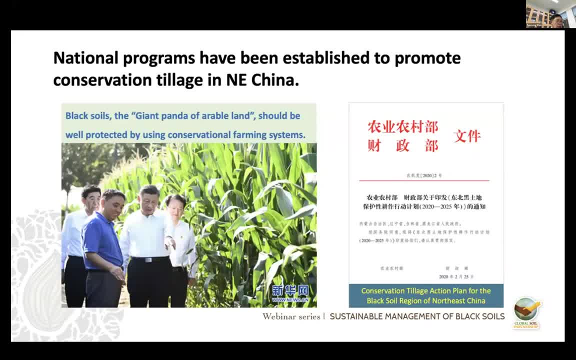 good crop yield. Our work has also drawn the attention of the governments at different levels. For example, in 2020, our President Xi, with our first set in Jilin province. he described the black soil as the giant pendant of arable land and he said that it should be well-protected. 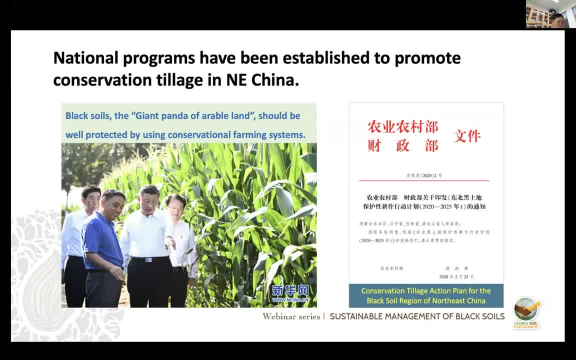 by using conservation farming systems. At the same time, the Ministry of Agriculture and Rural Affairs and the Ministry of Finance introduced the Conservation Technology Action Plan for the Black Soil Regions, And the Ministry of Agriculture and Rural Affairs and the Ministry of Finance introduced the Conservation Technology Action Plan for the Black Soil Regions. 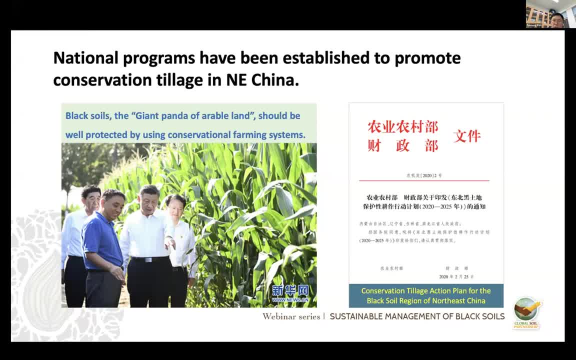 And the Ministry of Agriculture and Rural Affairs and the Ministry of Finance introduced the Conservation Technology Action Plan for the Black Soil Regions And they combined the types of soil control that we use in the region for our products in the North China Sea, which boosts the soil control of the Yilian region very quickly. 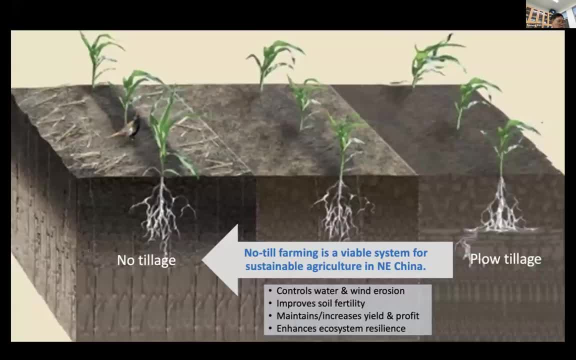 in the last few years. So, in conclusion, we believe that the industrial farming system is a viable system for sustainable agriculture in the North China Sea, because it effectively controls the water and wind erosion, improves the soil fertility and maintains or increases crop yield and profit. 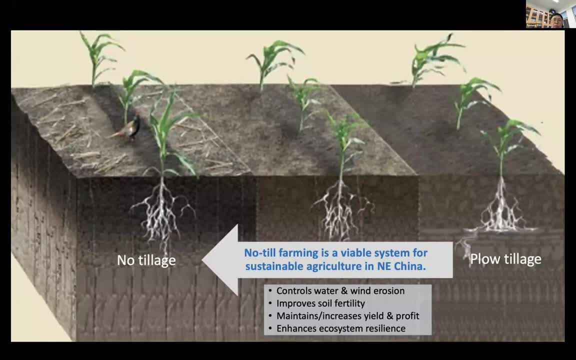 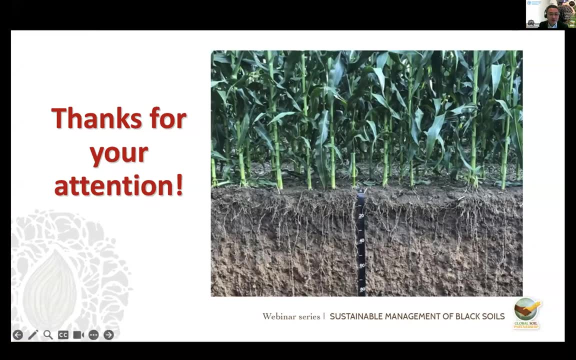 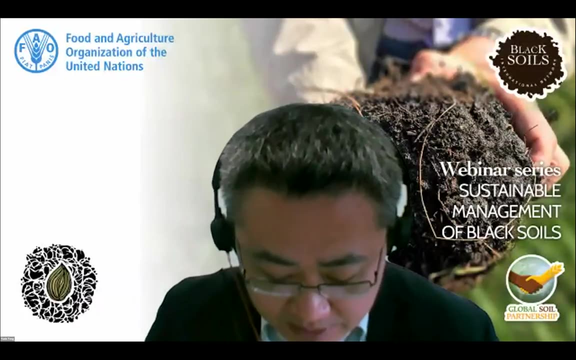 and also enhances the ecosystem ecosystem resilience. thank you for your attention. okay, i would like to ask you questions. thank you, professor ren. thank you very much for your presentation about the no tail farming system in northeast china, and your presentation uh introduced that the yield is very high there. 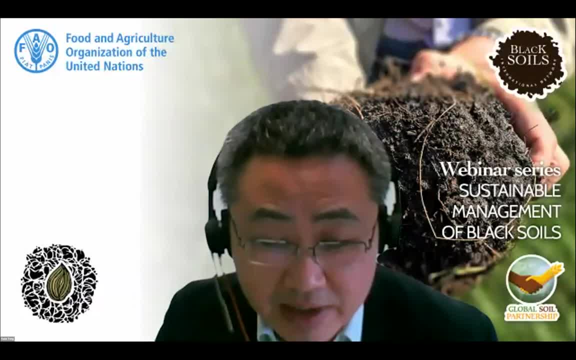 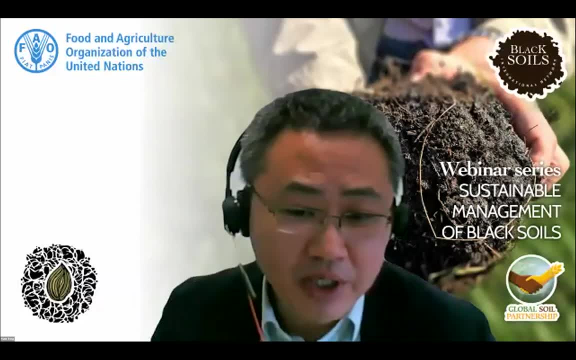 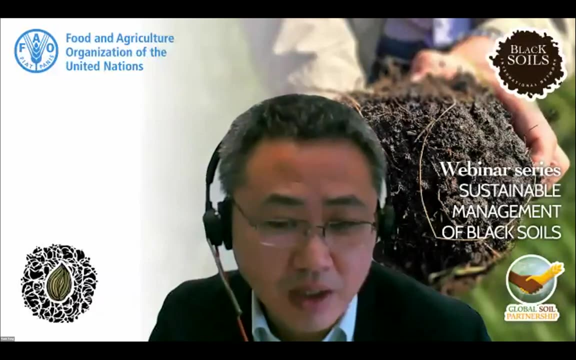 is a reach. the 10 to 15 10 factories and the no tail farming system can increase soil carbon, soil fertility and, i'd say, time- very important. these practices can also increase the benefit of farmers. that's always very important when we want to really recommend some good. 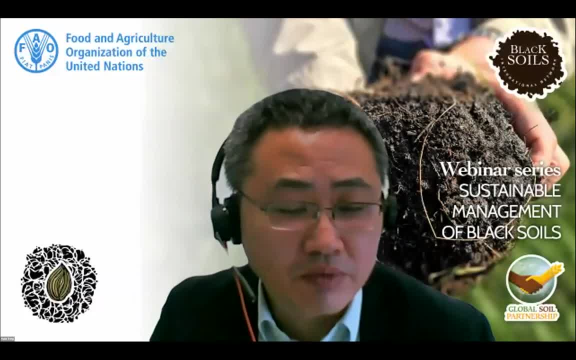 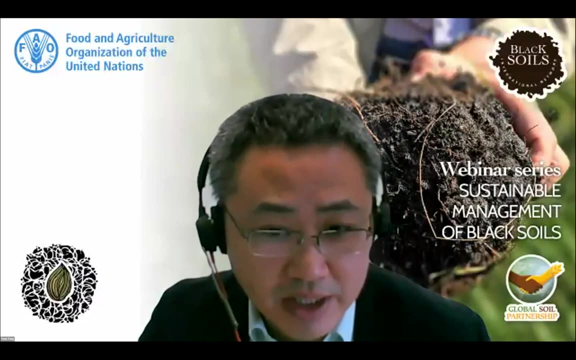 practices to to be used in the field. we must to consider the benefit of farmers. thank you very much. thank you very much for your presentation and, without further ado, now i would like to invite the third, third technical presentation from professor zhongjunjia from the northeast institute. 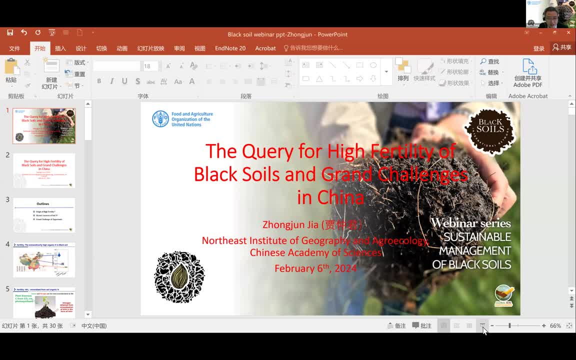 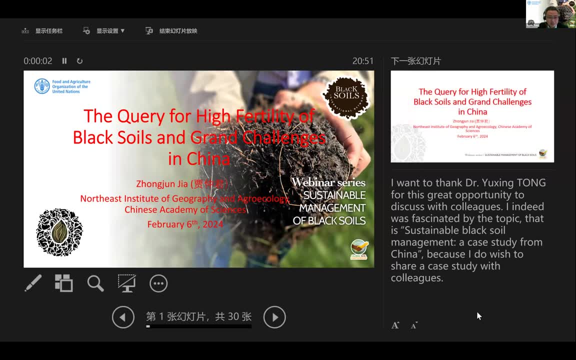 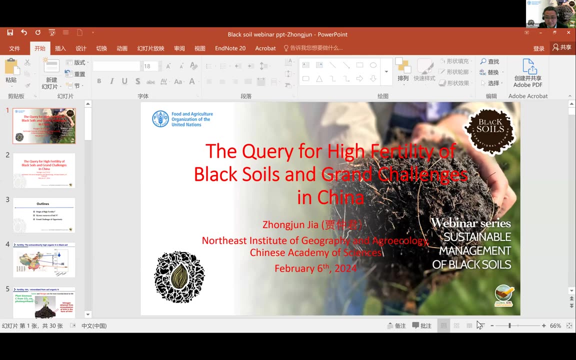 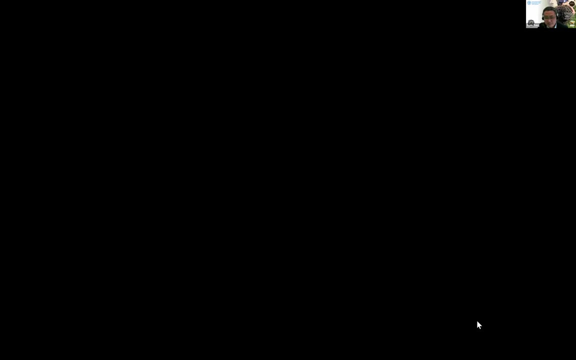 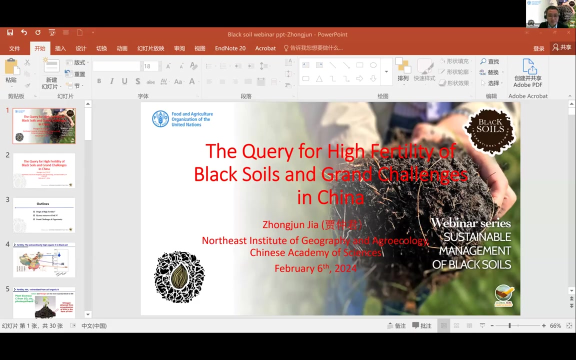 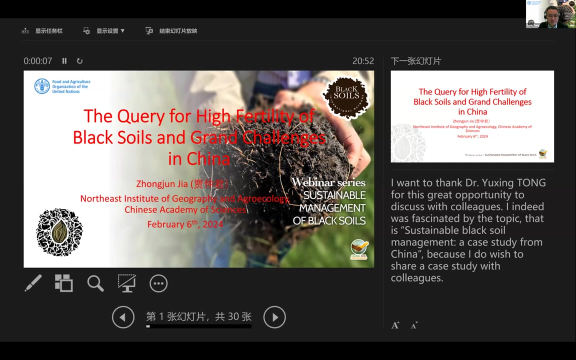 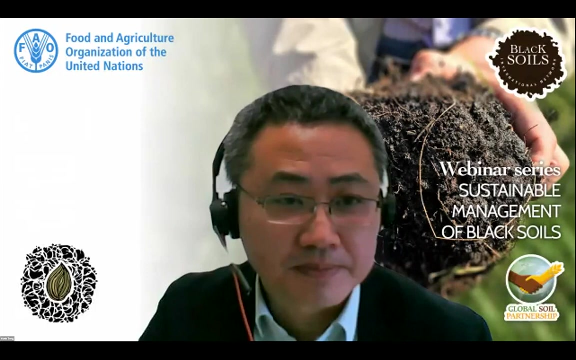 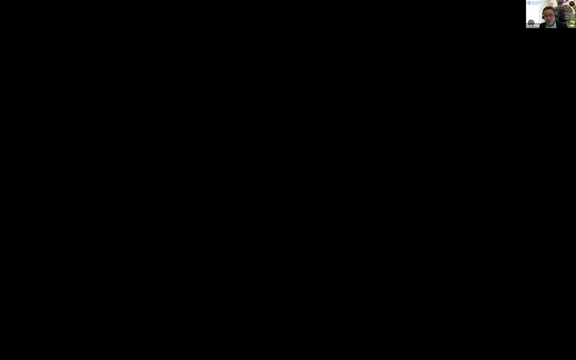 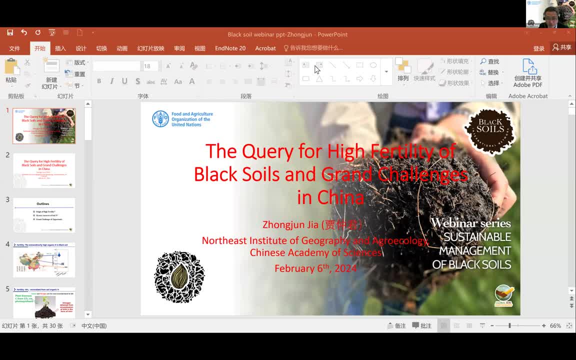 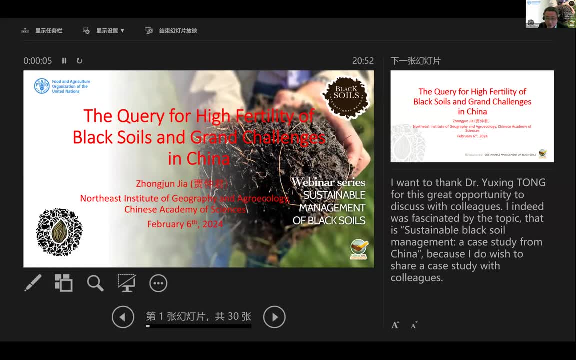 after the finish of the technical presentations, we will select question from the q and a in the zoom. then, uh, try to answer as many as possible of your questions during the discussion session of this webinar. thank you very much. please, uh, put your question in the q and a bottom and in of zoom and specifying which panelists you 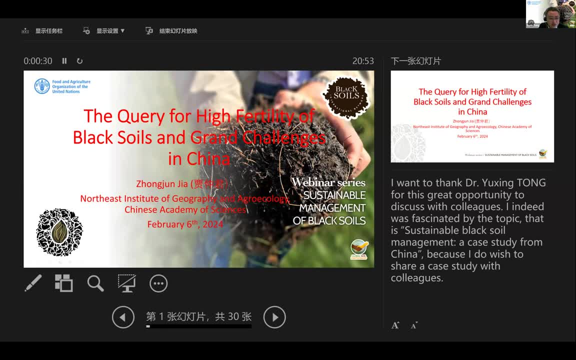 want to address the question to professor. yeah, we still see the grip format of the presentation that you have on the top right and we can see the grip format of the presentation. so i will just change it to the top right and we can see the grip format of the presentation. 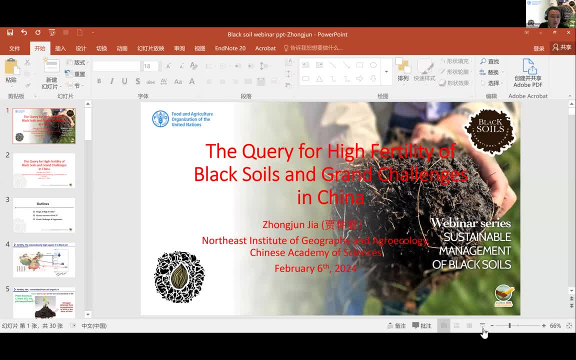 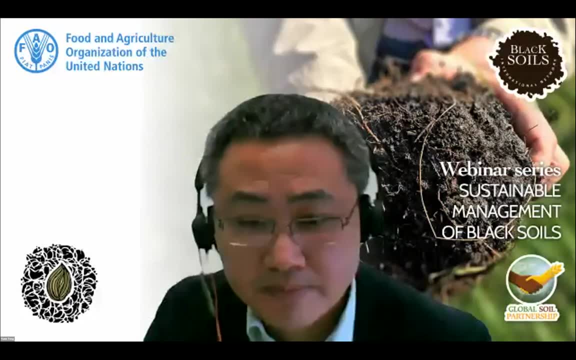 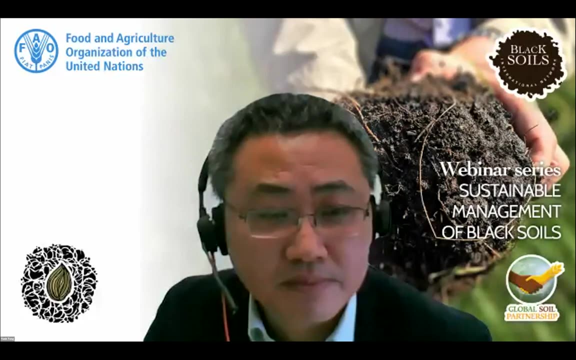 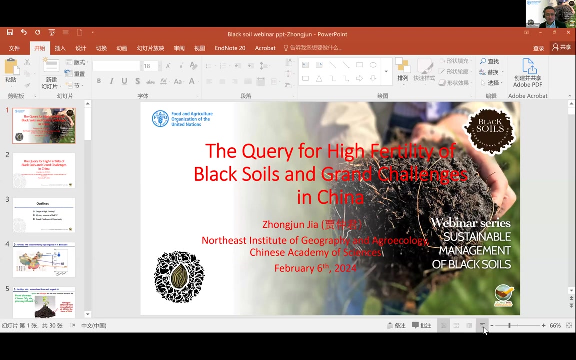 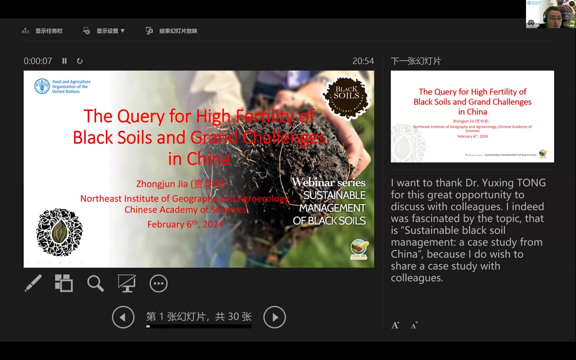 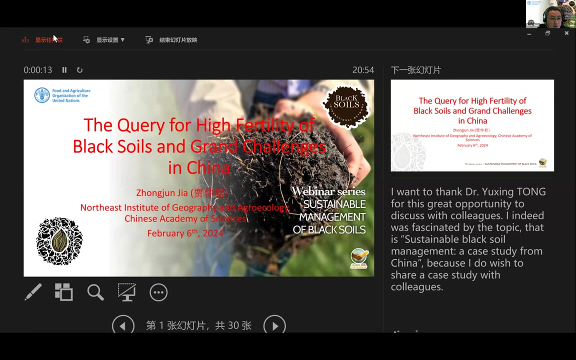 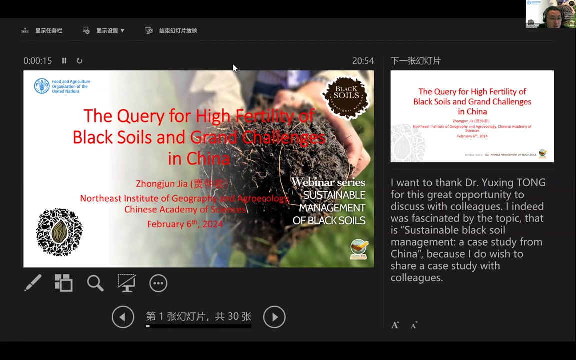 and we can use the in the same way to do the same thing. 贾老师上面有个显示设置, 左上角有个显示设置你点一下显示设置那个栏 右上角有个显示设置. 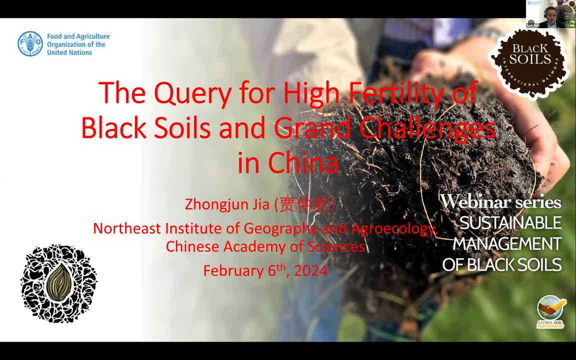 贾老师我们听不见您说话。. 贾老师我们听不见您说话。. 贾老师我们听不见您说话。. 贾老师我们听不见您说话。. 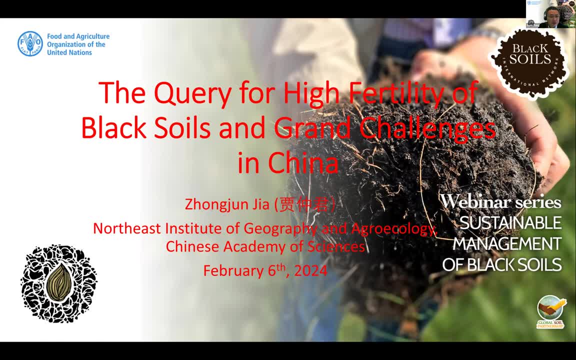 贾老师我们听不见您说话。. 贾老师我们听不见您说话。. 贾老师我们听不见您说话。. Hello, Professor Jia. 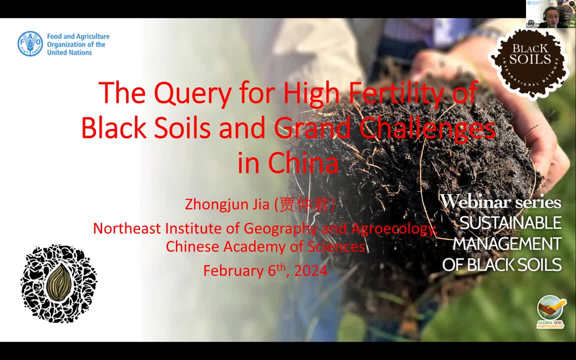 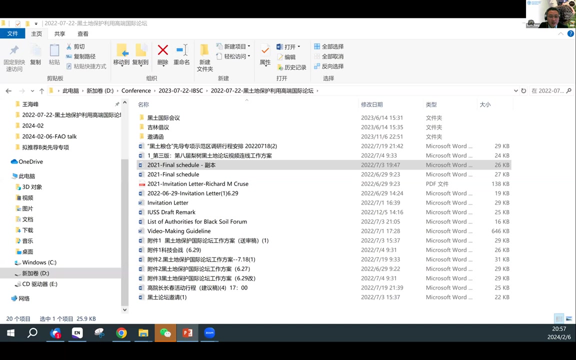 We cannot hear you. Hello, Professor Jia, We cannot hear you. We cannot hear you. I think there is some connection issues of Professor Jia. We cannot hear you. Sorry, we cannot know what happened to Professor Jia. Professor Jia, sorry, we cannot hear you. 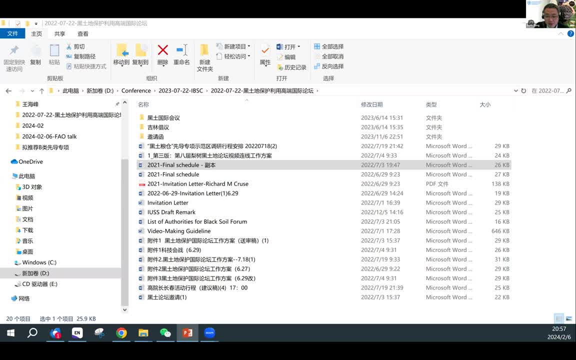 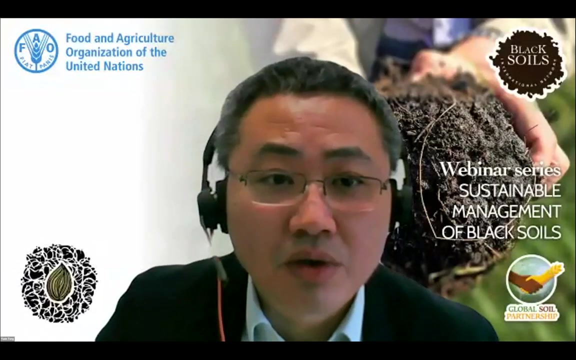 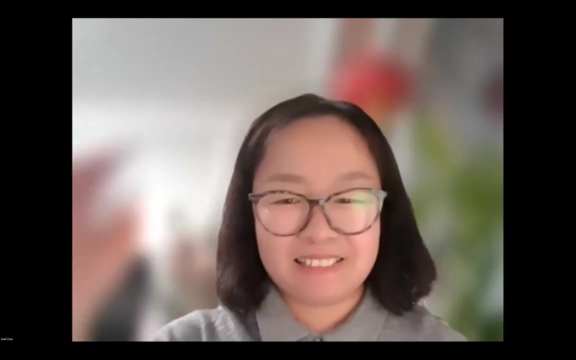 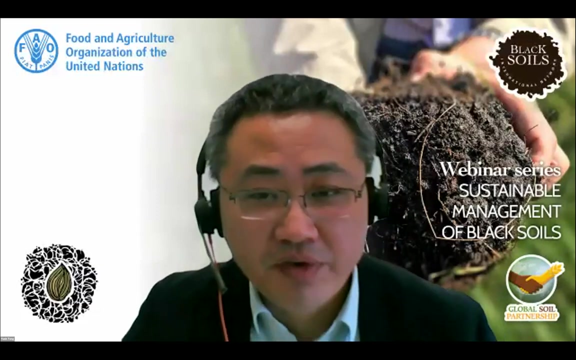 And So can you stop sharing the screen. So, Professor Chen Xue Li, Professor Chen, I think we can jump to Professor Chen, And we gave, We gave some time for Professor Jia to fix the internet problem. So, Professor Chen Xue Li, 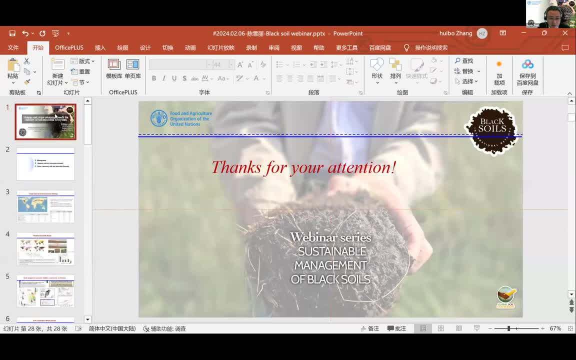 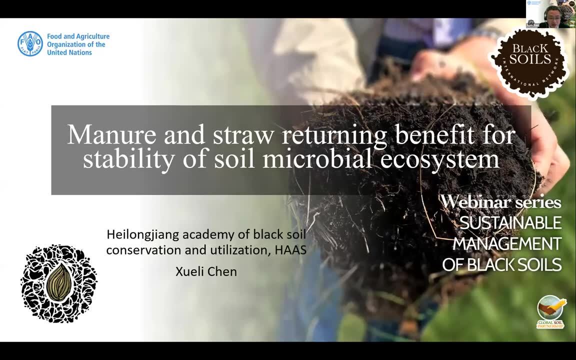 is come from Heilongjiang Academy of Agriculture Sciences And thank you very much. The floor is yours. Please give us the introduction and the information about the black soil management through manure straw returning In Northeast China. Please, The floor is yours. 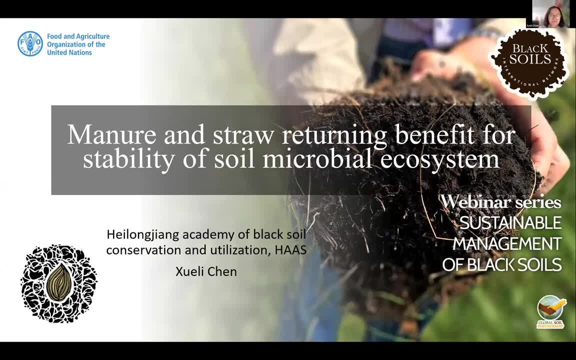 Thank you very much. Okay, Thank you. Good afternoon, Good evening And good morning Everybody. This is Xue Li Chen from Heilongjiang Academy of Agricultural Science. It is my honor, how this opportunity to share our work with all of you. 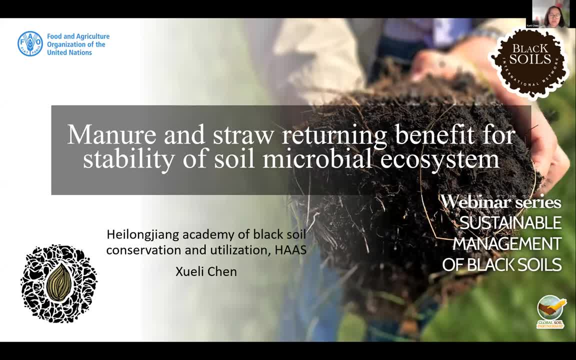 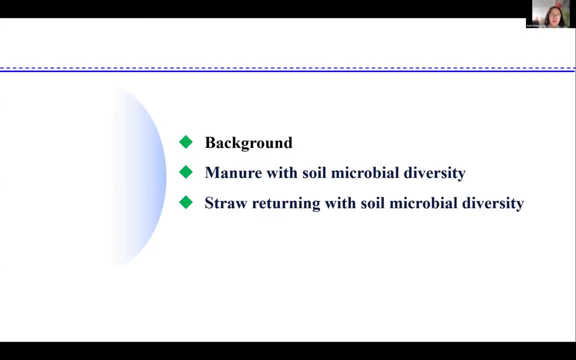 The title of my report is MANURE & STROLE: Returning Benefits for Stability of kerosene Mig염 into Soil by Euclidia. He did well with his entry, So please continue, Please continue. ecosystem, And I will give a report according to these three parts as: 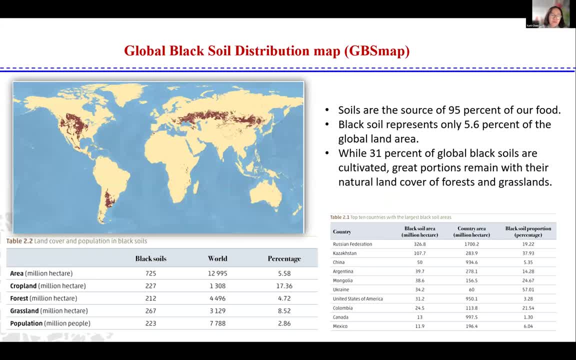 follow. As we know, soil make an important contribution for our life, including food production, air cleaning, pollution filter and so on. According to the statistic, that soil are the source of 95% of our food. while black soil is one important kinds of soil types, it repress only 5.6% of. 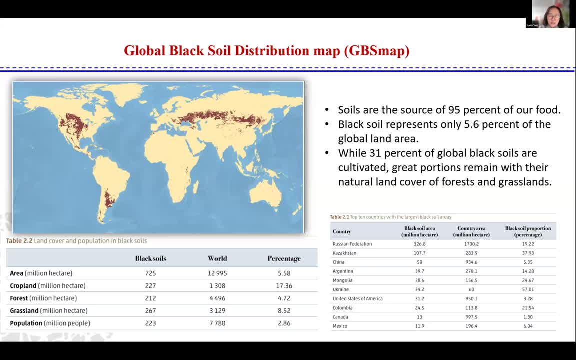 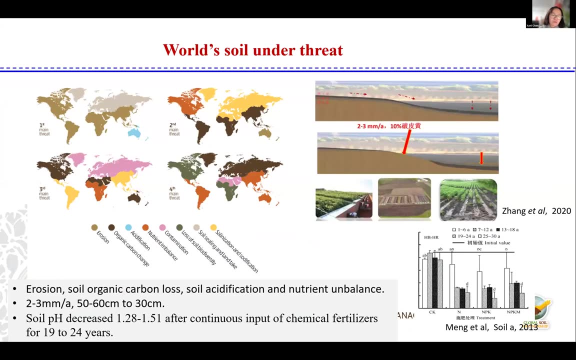 global land area. While 31% of global black soil are cultivated, great portions remain with their natural land cover of forests and grassland. Then the worst soils are under threat: Erosion, soil organic carbon loss, soil acidification and nutrients unbalance. 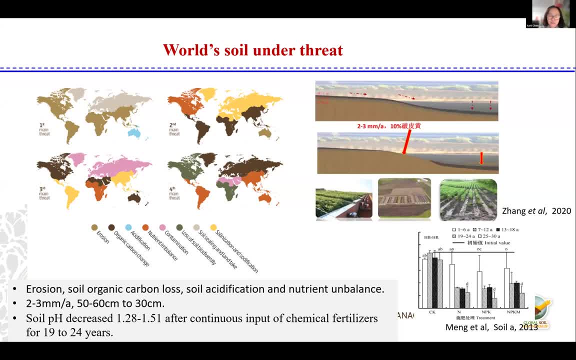 are four main soil problems, Also for black soil. according to the report, there are two to three millimeter soil loss in plough layer each year And the depths of plough layer decline from one to three millimeter soil loss. Soil pH decreased from 50 to 60 centimeter before reclamation to 30 centimeter. 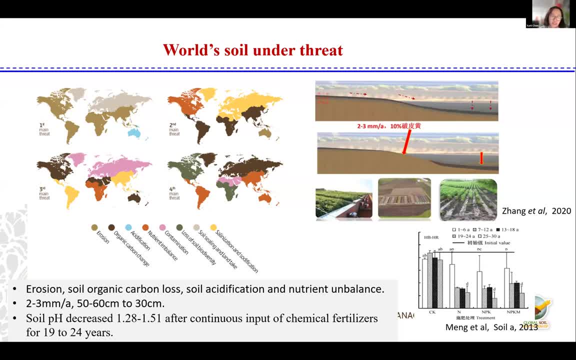 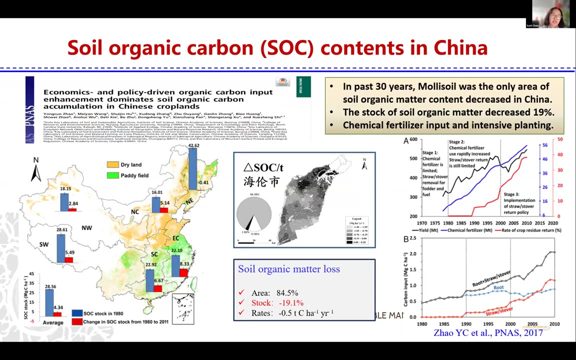 till now in China, Soil pH decreased 1.28 to 1.51 after continuous input of chemical fertilizer for 19 to 20 to 24 years. About soil organic matter of organic carbon content, there was a paper published on PNAS in 2017, which reported the soil organic carbon content in all over China in 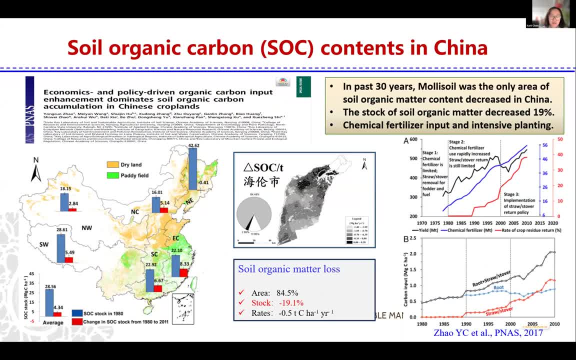 past 30 years. The results showed that molybdenum was the only area of soil organic matter content decreased in China. The stock of soil organic matter in China has decreased. The stock of soil organic matter in China has decreased. The stock of soil organic matter in China has decreased. 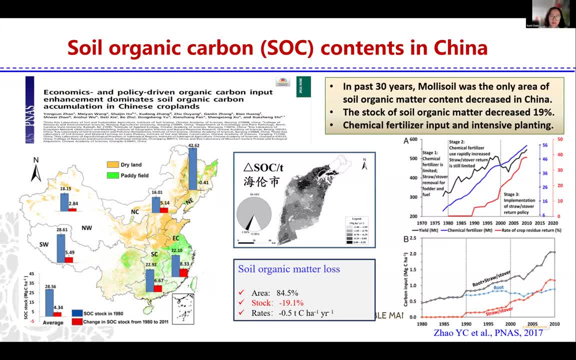 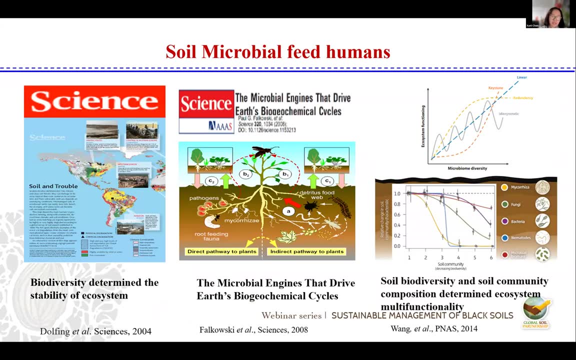 The stock of şeyi retainer in this area decreased 19%. The main reason was excessive chemical fertilizer input continuously and intensive planting. Soilizard пуq winco is a sensitive indicator of soil quality changing, which got more and more attention worldwide experts. 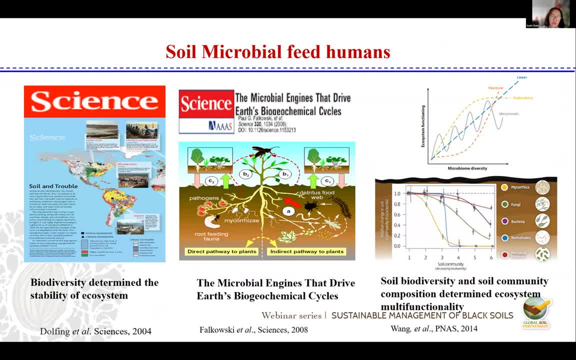 There were two papers published on science in 2004 and 2008 emphasized that biodiversity determined the stability of the ecosystem and the microbial energy that drives Earth's biogeochemical circles. And in 2014, there was a paper published on PNAS which further emphasized soil biodiversity. 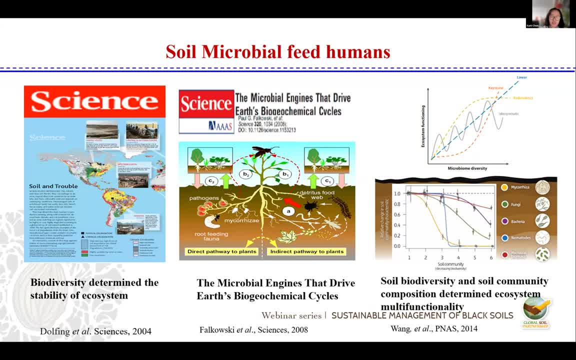 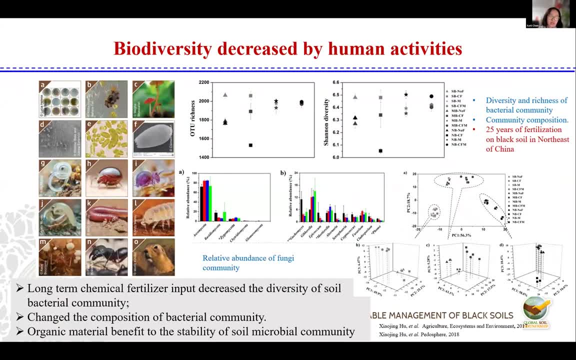 and soil community composition determined ecosystem multifunctionality With the development of agriculture, long-term chemical fertilizer input resulted in decreasing of diversity of soil microbial communities. changing of the composition of bacterial communities. Studies show that organic matter material application benefits the soil microbiology. 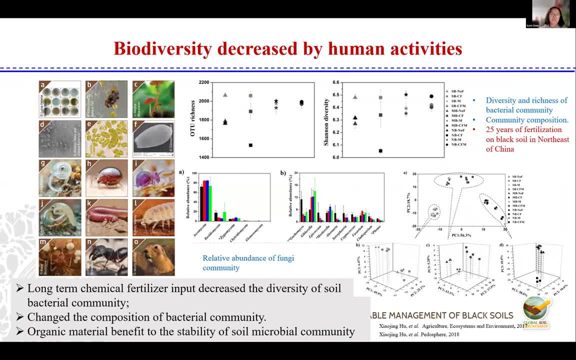 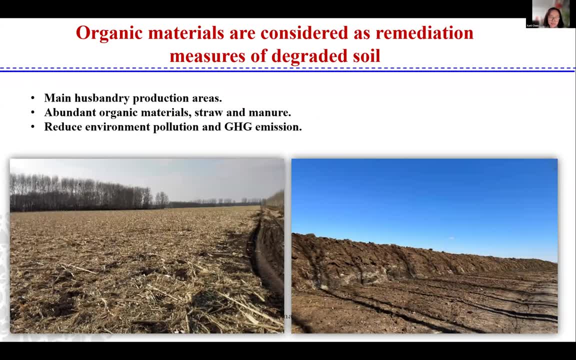 Actually, black soil areas are not only the food production basis, but also it is the main husbandry production areas. There are abundant organic materials, for example straw manure. Returning the straw and manure to the air balance also benefits to reduce environment pollution. 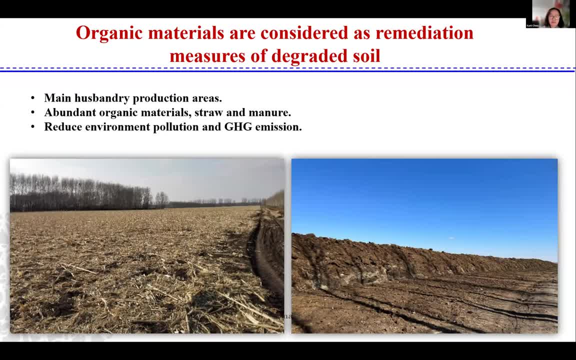 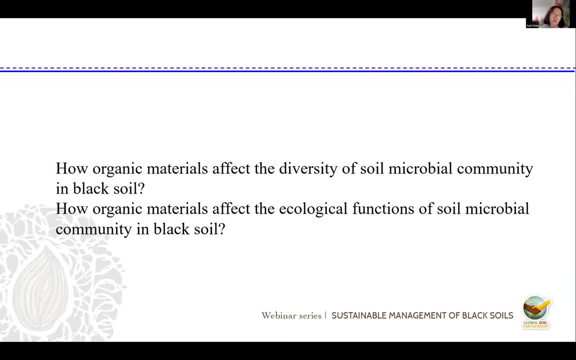 And greenhouse gas emissions. So this report. today I want to answer two questions based on the work of our team in past several years and the reference which published based on our long-term fertilization experiment in black soil. The first question is how organic materials affect soil. 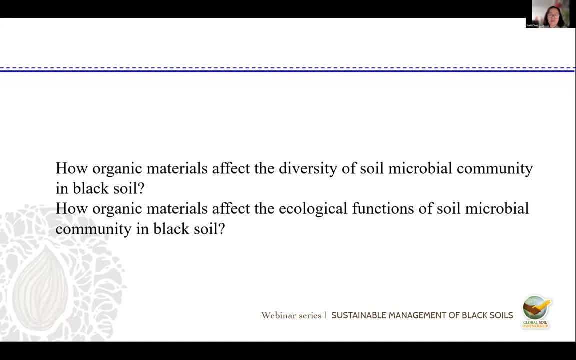 The second question is how organic materials affect soil. The third question is how organic materials affect soil. The fourth question is how organic materials affect soil. The fifth question is how organic materials affect the diversity of soil microbial community in black soil. And the second question is how organic materials affect the ecological functions of soil microbial. 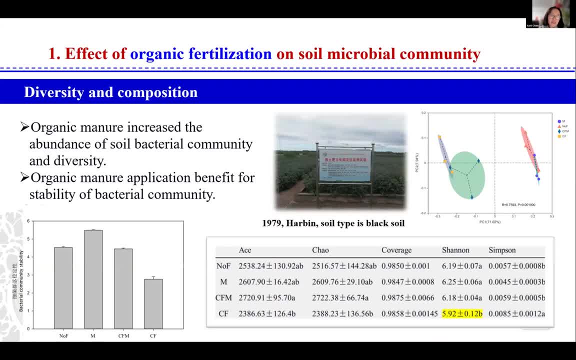 communities in black soil. The first question, I will give an introduction about the impact of organic fertilizer on soil microbial community. On the side of the impact of soil microbial community in black soil, of organic fertilization, of diversity and composition of soil microbial community. 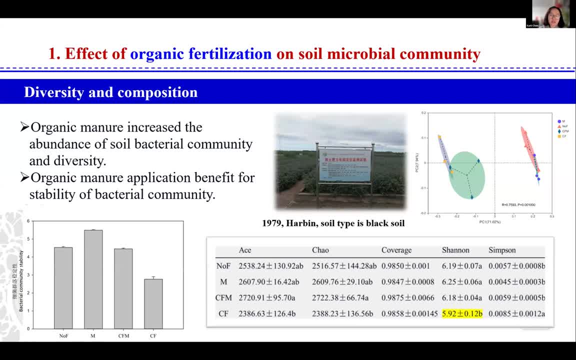 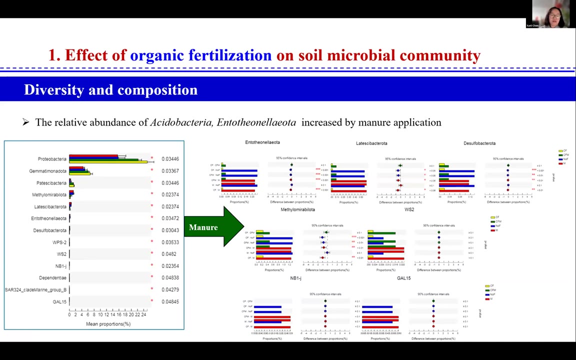 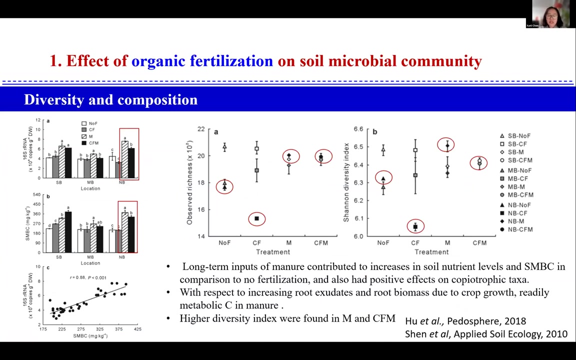 We found that organic manure application increased the abundance and diversity of soil bacterial community. Manure application benefit for stability of bacterial community. The relative abundance of phylum increased by manure application. The results confirmed by Dr Hu and Dr Shen in 2008 and 2010,. they found that long-term inputs 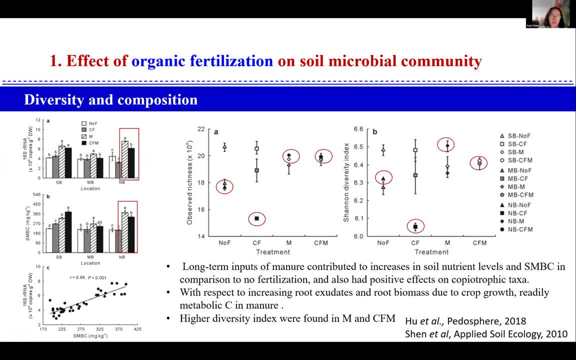 of manure contributed to increase in soil nutrient level and the soil microbiome, biomass carbon in compared to no fertilizer, no fertilization. and also how had a positive impact on copic trophic toxic With respect to increasing root exudates and root biomass. 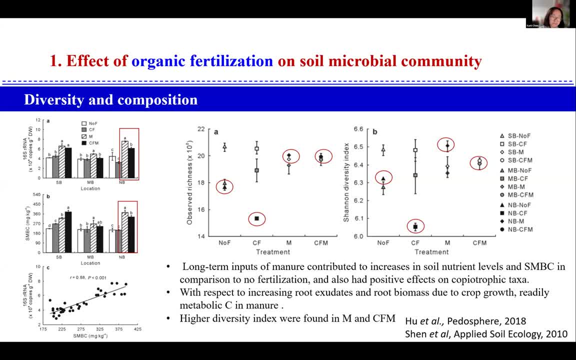 due to crop growth readily. a type biotic carbon in manure had a diversity index of manure And next look at a total carbon byving of phylon in material using organic fertilizer for better dairyанию and duglet, phytonutrients being found from Actually. 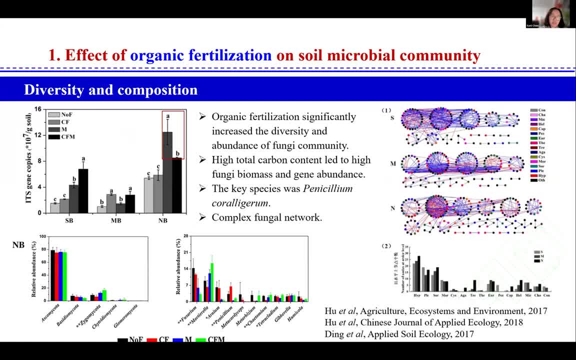 this found. organic fertilizers were found in manure and chemical fertilizer combined with manure or fungi community. They found organic fertilizer significantly increased the diversity and abundance. high total carbon content lead to high fungene biomass and gene abundance. The key species was Pythidine. 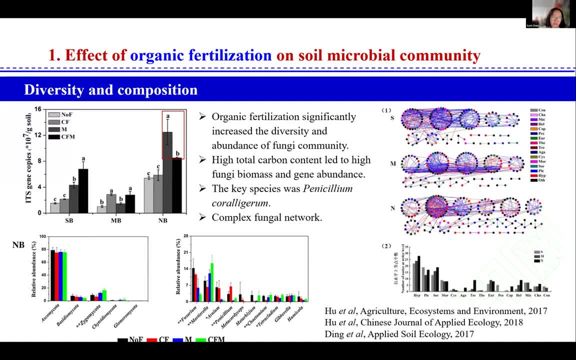 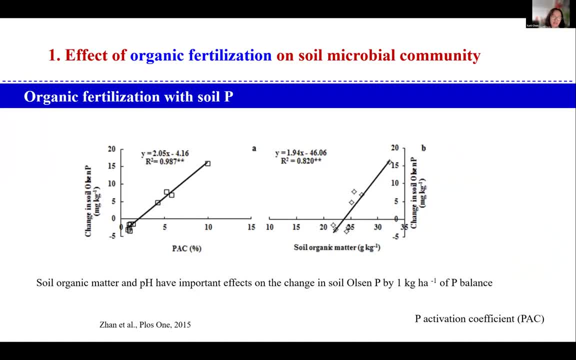 The fungene network in manure treatment showed more complex About the relationship of organic fertilization with soil. phosphorus, Soil organic matter and pH have important impact on the change in soil ozone. phosphorus by 1 km per hectare of phosphorus balance. 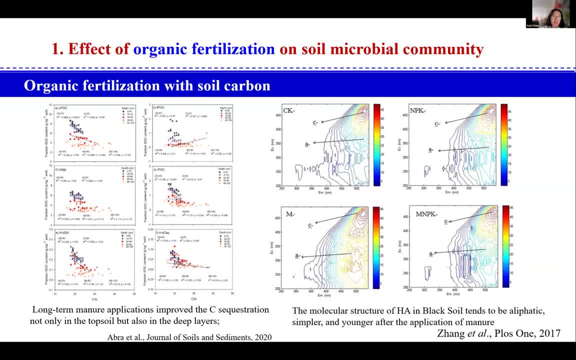 About the relationship of organic fertilization with soil. carbon showed that long term manure application improved the carbon sequence sequence with nutrition, not only in the top soil but also in the deep layers. The structure of the HA in black soil tends to be alphatic. 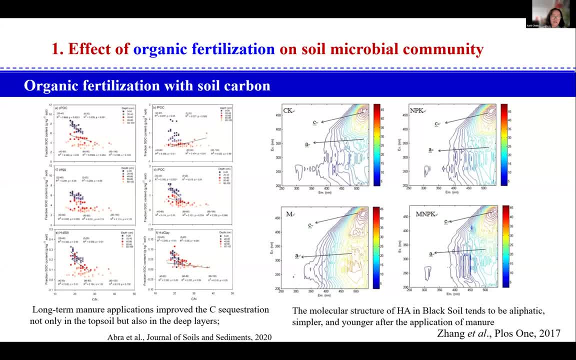 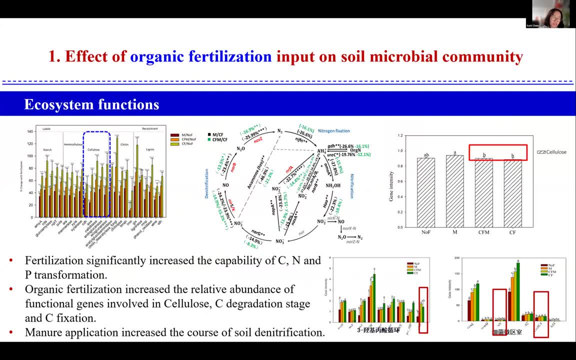 alphatic and the younger after the application of manure. Function of function genes diversity by geoshape. The results showed that the diversity of functional genes decreased by organic manure application. The composition of functional group in manure and chemical fertilizer combined with manure are similar. 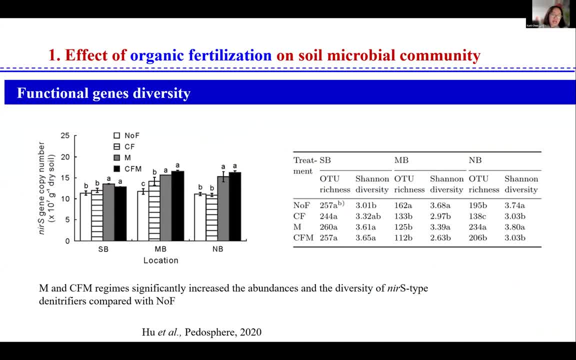 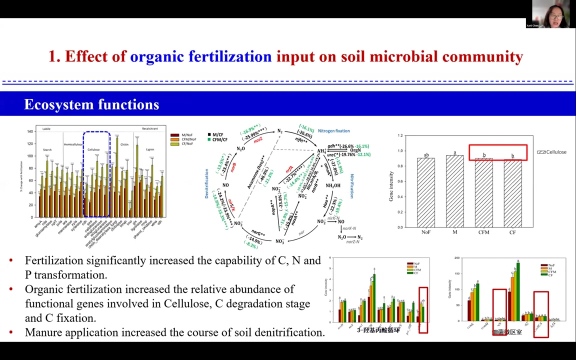 About the ecosystem functions. We found fertilizer significantly increased the capability of carbon nitrogen and phosphorus transformation. Organic fertilization increased the relative abundance of functional genes involved in the cellulose Carbon degradation stage and carbon fixation, And the manure application increased the cost of soil denitrification. 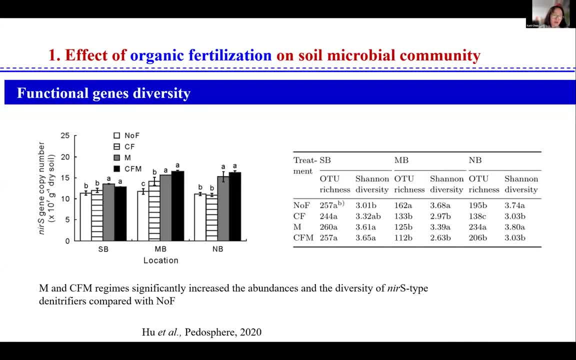 The results also were coincided with the study for Dr Hu in 2020.. She found the manure and chemical fertilizer combined with manure significantly increased the abundance of and the diversity of nurse ice type denitrification features, compared with no fertilization. 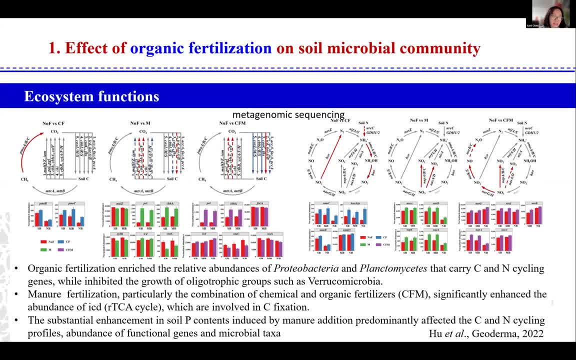 And organic fertilization enriched the relative protection and the plantar mysis that carried the carbon and nitrogen circle genes Well inhibited the growth of oligocrophic groups such as the varroa chemimicrobi. Manure fertilization, particularly the combined with the chemical and 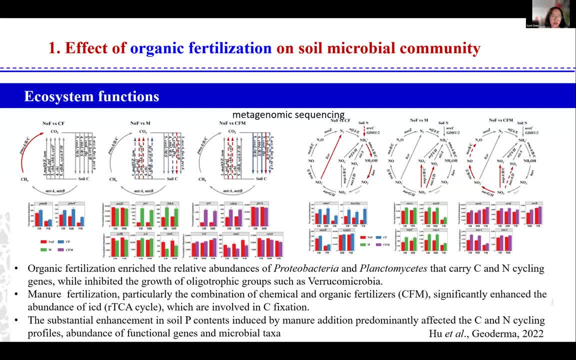 organic fertilizer Significantly enhanced the abundance of ice, which evolved in carbon fixation. The substantial enhancement in soil phosphorus contents induced by manure addition Predominantly affected the carbon and the nitrogen carbon circle profiles, Abundance of function, genes and microbial texts. 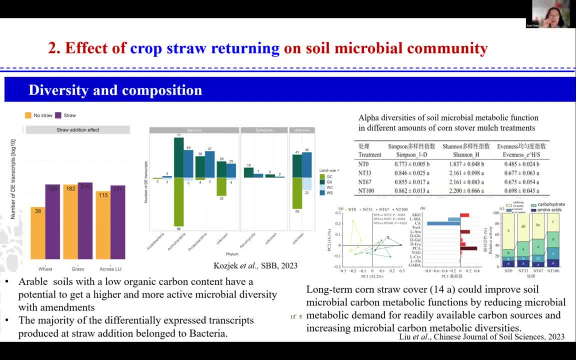 The second part about the impact of crop straw returning on soil microbial community, About the diversity and the composition of soil microbial community affected by straw returning showed that arable soil with low organic carbon content have a potential to get a higher and more active microbial diversity. with abandonment amendments. 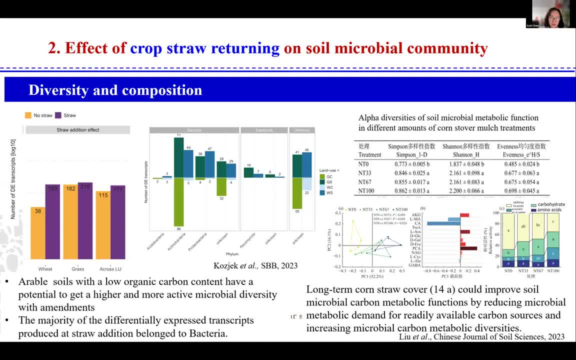 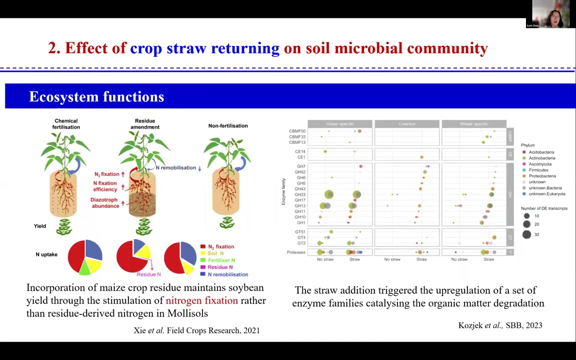 And the majority of differently expressed transfer transcripts produced at straw. addition belongs to bacterial And the long-term maize straw cover could improve soil microbial carbon metabolic functions By reducing microbial metabolic demands for readily available carbon source And increasing microbial carbon metabolic diversity. About the ecosystem functions of soil microbial affected by straw. 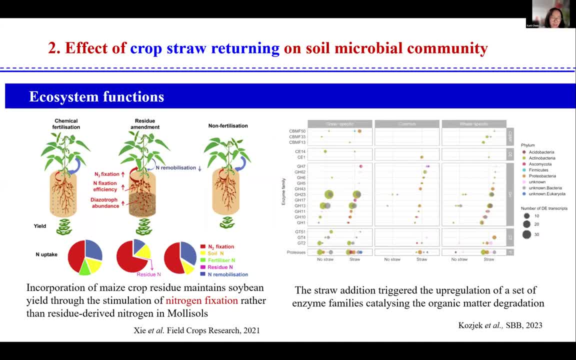 returning showed that incorporation of maize crop residue maintains the soybean yield through the stimulation of nitrogen fixation Rather than residue. derailed nitrogen in molysul And the straw addition triggered the operation of a set of families ley singed organic matter degradation. 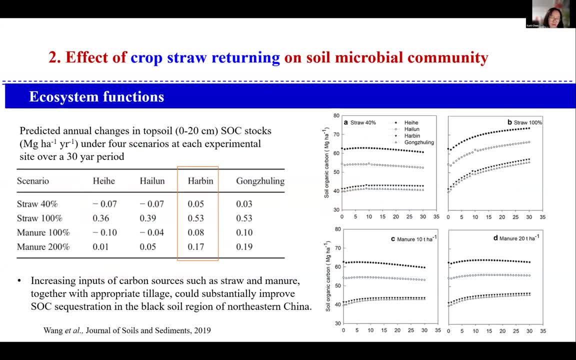 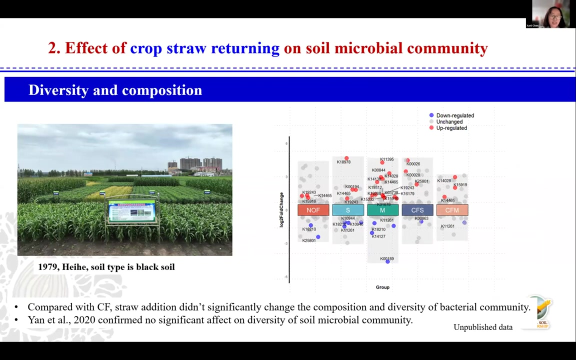 Increasing the input of carbon source that has the straw and manual together This probably carbon sequestration in the Black Soil region for Northeast China. Then these fundings are focused on the diversity of the soil bacterial community, carbon microbiota and the nitrogen fiction of straw returning separate. 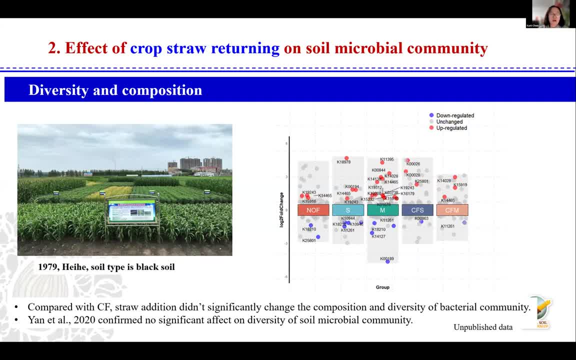 Our team analyzes the soil microbiota community composition and the function genes based on the continuous straw returning for 41 years In Heihe. this experiment is established in 2012.. Oh, I'm sorry, I don't think this picture is wrong, I think. 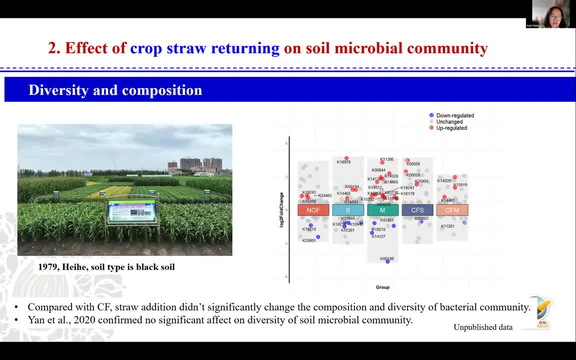 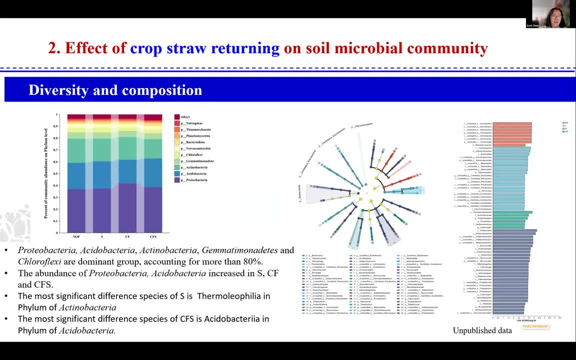 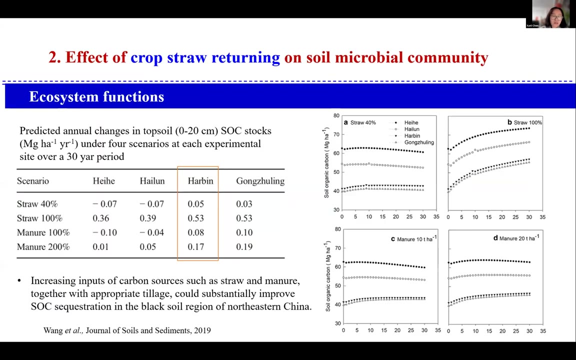 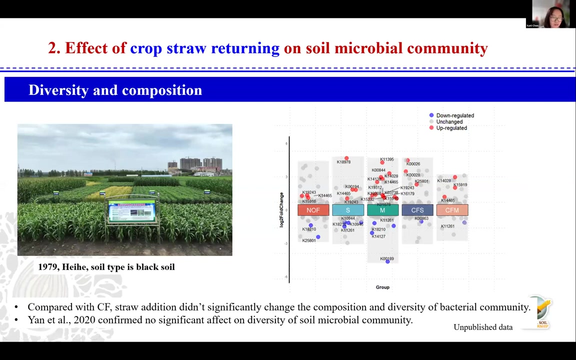 The rotation system is soybean and maize. The soil type is Black Soil. Compared with chemical fertilizer, the straw addition didn't significantly change the composition of the soil. The soil composition and the diversity here didn't change the composition and the diversity of bacterial, and the results coincided with Yang published in 2020.. 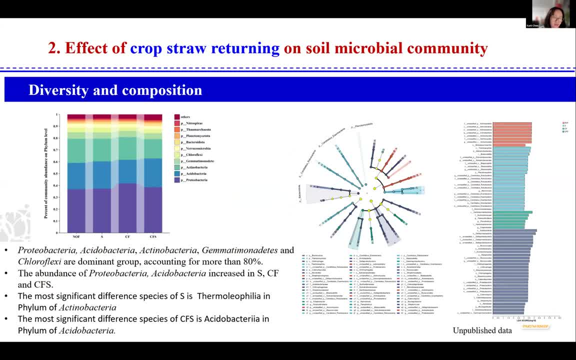 By identifying the NG note with the highest degree of network as a keynote note. it was found that the keynote of straw application alone's treatment is mainly due to the fifth gene related to cellulose decomposition, and the two general with the highest degree of positive correlation are belongs to the actin bacterial and the acid bacterial. 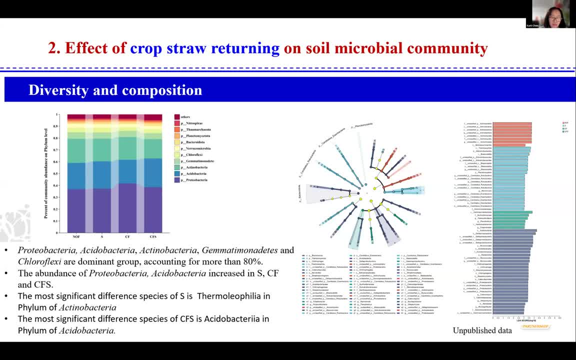 They are involved in primary decomposition of plant materials in soil and hold ability to degrade complex organic compounds in soil. The chemical fertilization is the micro gene associated with starch metabolism. Okay, Yes, and glycol degradation is a member of phylum acid bacterium. 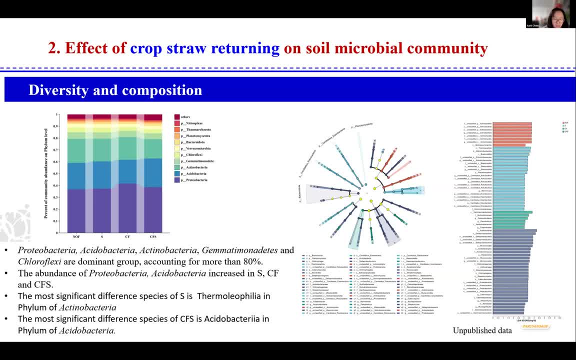 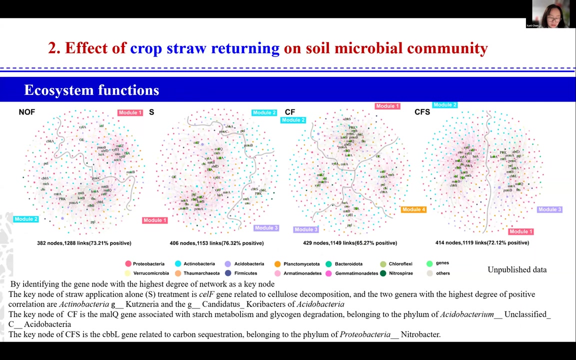 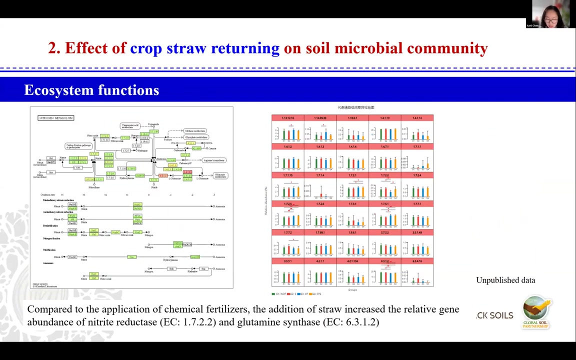 Chemical fertilizer combined with straw is the CBBL gene related to carbon sequestration. This gene belongs to a proteobacterium. It's the nitrified bacterium produce acidic substance to improve the alkaline soil. This, compared to the application application of chemical fertilizer. The addition of straw increased the relative gene abundance. 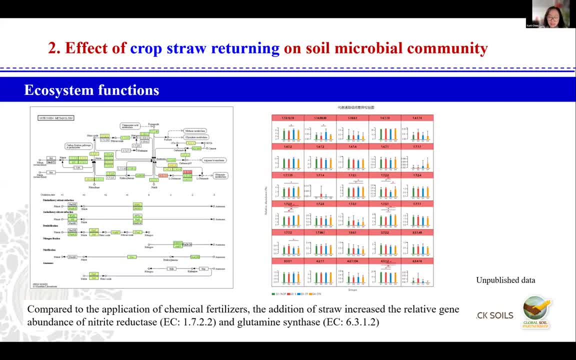 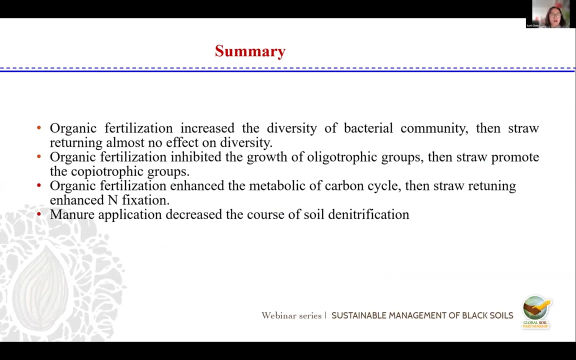 of nitrate, reducing the tax and the global system. I just reported the results we just got from the experiment, so it's an unpublished date. Overall, I gave a summary. Organic fertilization increased the diversity of bacterial community, then straw returning almost no effect on diversity of the bacterial community. 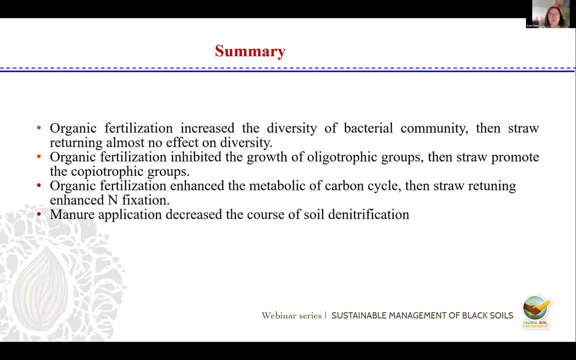 Organic fertilization inhibited the growth of oligotrophic groups, then straw promotes the compitrophic groups. Organic fertilization enhanced the metabolic metabolic of carbon circle, then straw returning enhanced the natural nitrogen fixing effect. Organic fertilization decreases the cost of soil denitrification. 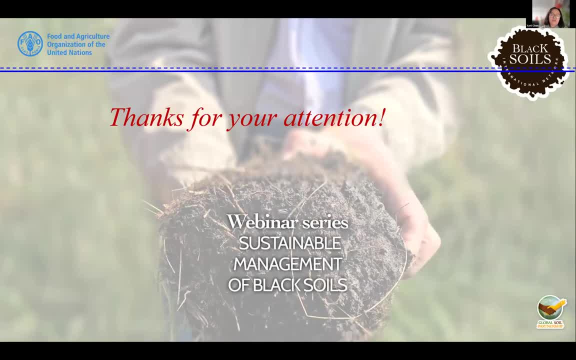 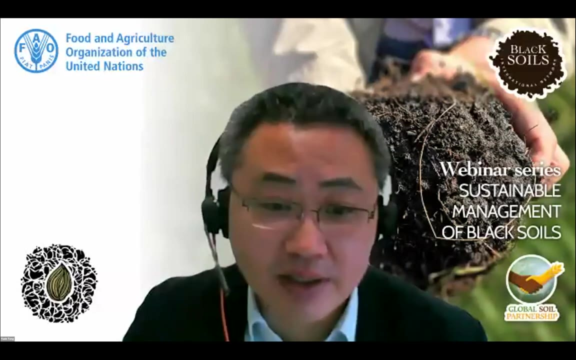 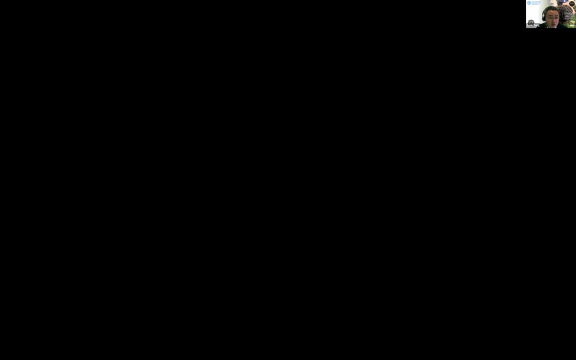 Ok, that's all my report. thank you for your attention. Thank you very much, Professor Chan, and thank you for your presentation regarding organic farming and the manure application for the black soils. and indeed, the manure application on organic farming system can also improve black soils and can also protect black soils at the same time. 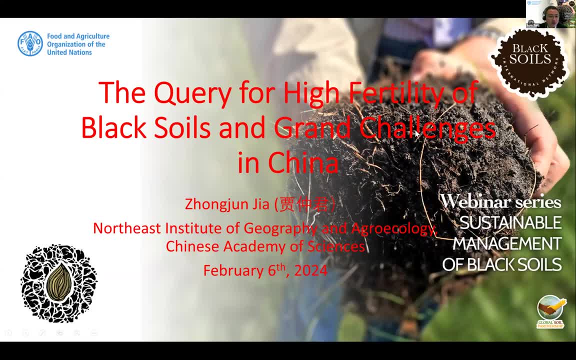 ensure the food security, ensure the yield. thank you very much, professor Chen. and now I would like glad to invite professor Jia to make his presentation. and professor Jia come from the Chinese academy of sciences and then the from the northeast institute of geographic and agroecology. professor Jia, the floor is yours. okay, thank you. yeah, yeah, yeah, loud and clear. 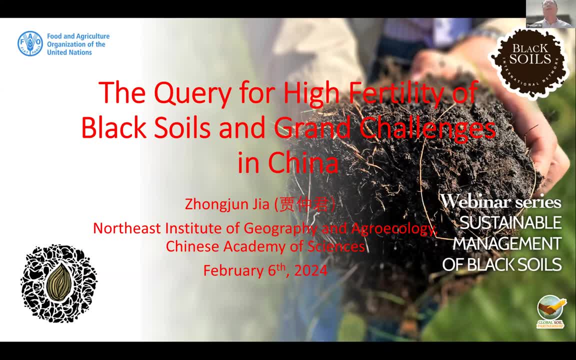 thank you, please go ahead. thank you very much. I'm so very sorry. I actually, we, indeed I indeed had a pre-tester for the presentation. I'm sorry. something is going wrong was going on at my side, so I would like to apologize for this inconvenience to all. 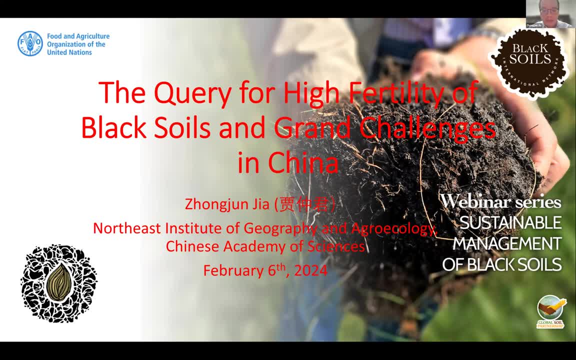 the audience audience. so I would like to start my talk by, first of all, thank you, Yu Xin, for this great opportunity to discuss this with the colleagues. I actually I was fascinated by this topic, that is, sustainable black soil management- a case study from China. so I mean, it's a case study. 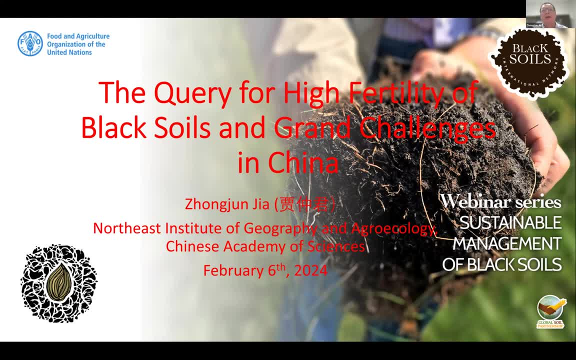 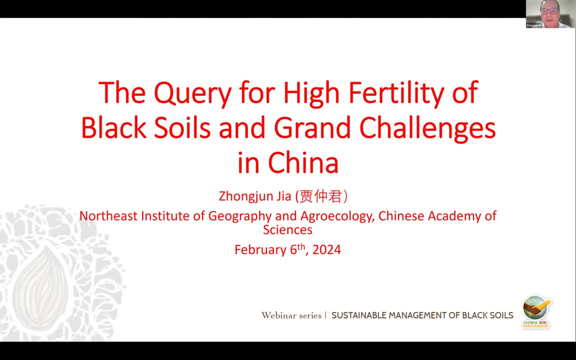 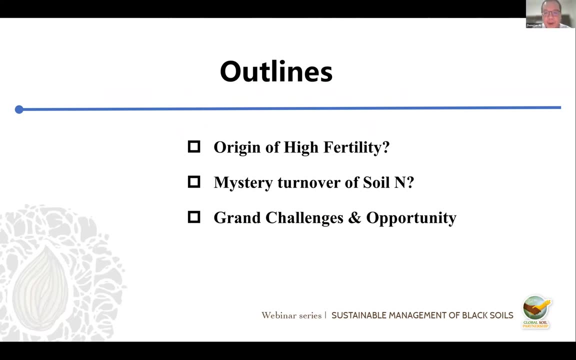 and because I do wish to share a case study with our colleagues. so the title of my talk is the query for highway fertility of black soil and underground challenges in China. so the alternance of my talk include includes three parts. the first, the whole black that have 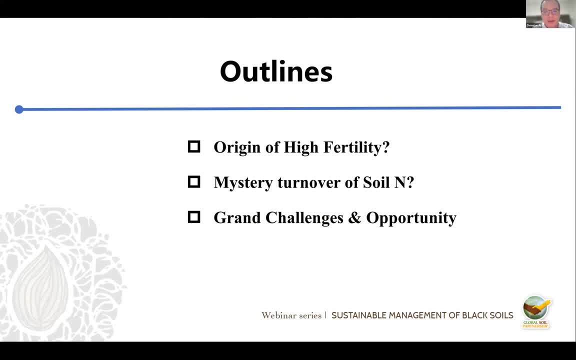 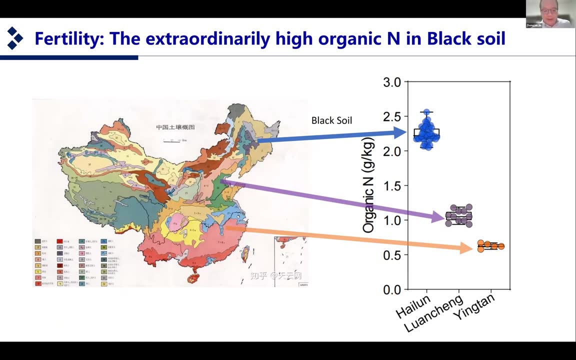 been for the reality of in black soil is originated under the mysterious turnover of soil, organic nitrogen and the final part is the ground challenge, challenge and opportunity. So, as we all know that black soil has extraordinarily high organic nitrogen in black soil, I would like to see this the origin of the high fertility. So you can see. 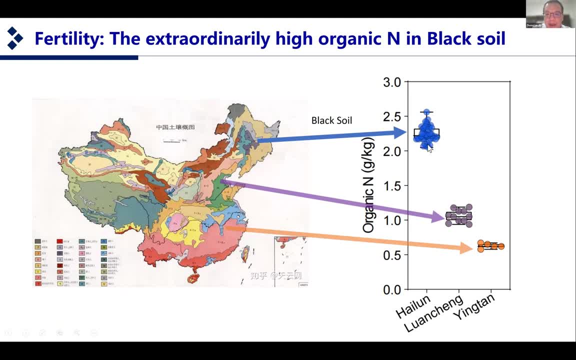 the black soil in China are mostly, maybe completely, located in northeastern China, which is a cold temperate region. As you can see, the black soil in northeastern China has the organic nitrogen which is two times higher than the loamy soil in the north China. 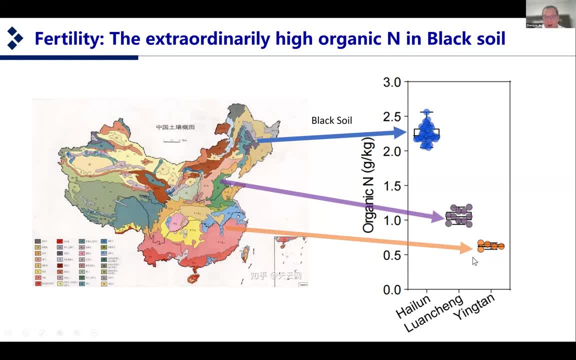 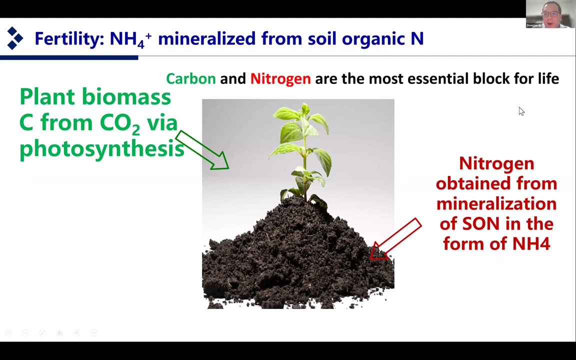 which is close to Beijing and four times higher than the red soil in southern China, southern part of the China, And we know that carbon and nitrogen are the most essential block for life, and ammonium and, historically speaking, ammonium is the key nitrogen source for plant and it must be. 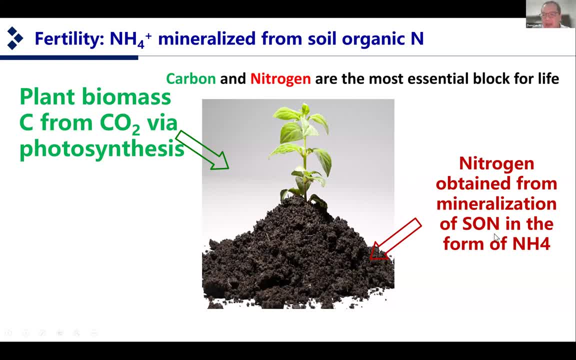 obtained from mineralization. In the meantime, the photosynthesis carbon serves as the key source of the plant biomass. carbon from what we know in the atmosphere, CO2, which is largely about 400 ppm in the atmosphere. So I would like to say the carbon source for plant growth is almost endless in the air. but 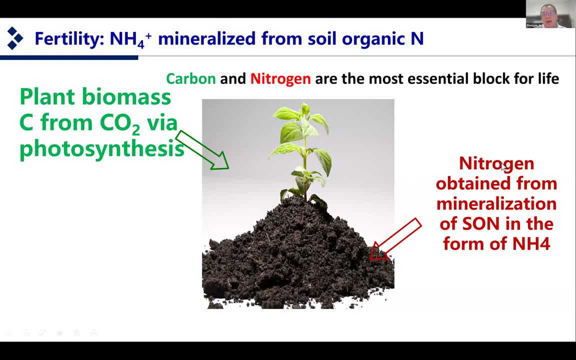 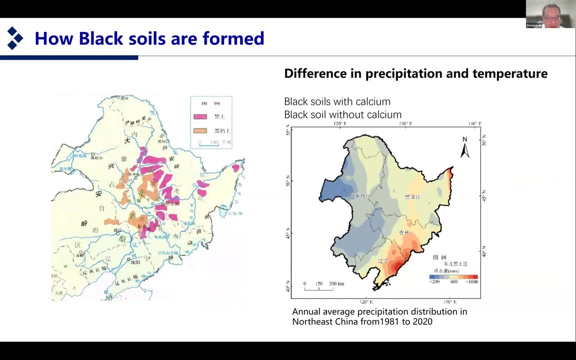 we know the nitrogen. the nitrogen in the air is not reactive nitrogen. It cannot be directly used by plant. So soil organic nitrogen is very important. So we know the black soil from Russia actually is widely accepted as the founding father of the soil's sense, like the dog child, Black soil in Russia we know has contains plant. 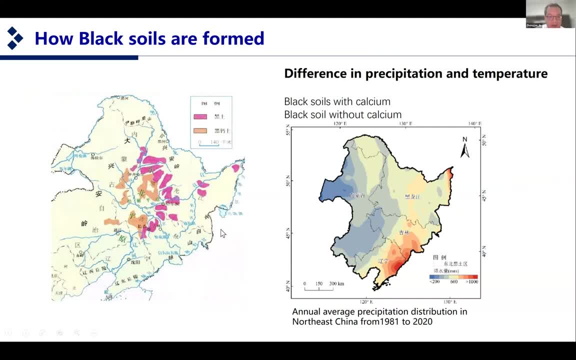 of the classing where it does not hold true. in china you can see the some black soil in china has has no calcium. in this region i mean this black soil in the bread color. it has no calcium or very little calcium, and the and the black soil with calcium is colored with a dark, dark brown. so 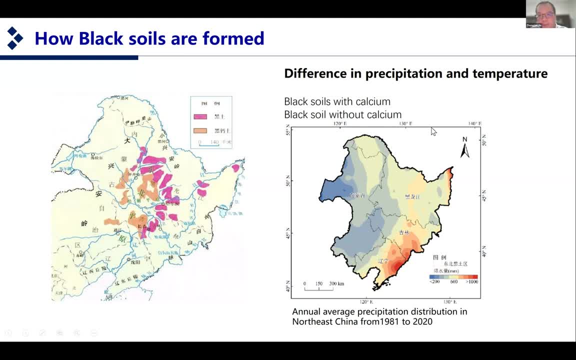 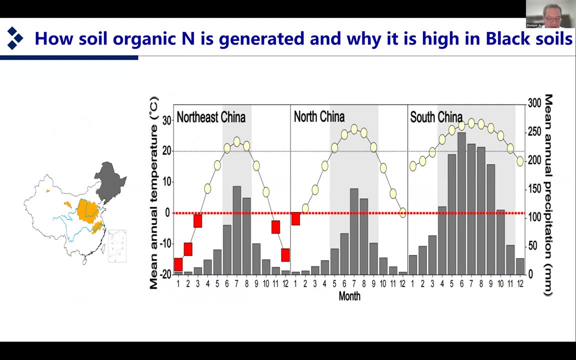 why this deep? there is a certain kind of difference. it is from the precipitation. you can see in this region there is a high precipitation so the calcium is elapsed from the black soil surface. so the question is why the soil organic nitrogen is high in the black soil and how it is generated. you can see in this figure. this is the map of 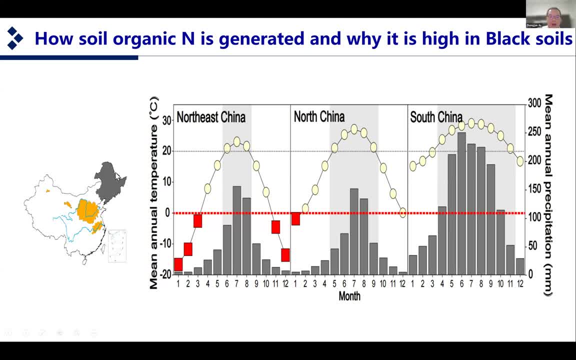 the channel. this is north east wind, ww, codult, fandel, China, where most black soil are located. This is the north China In Beijing. this is southern China. This is the brown soil, this is red soil, this is black soil. 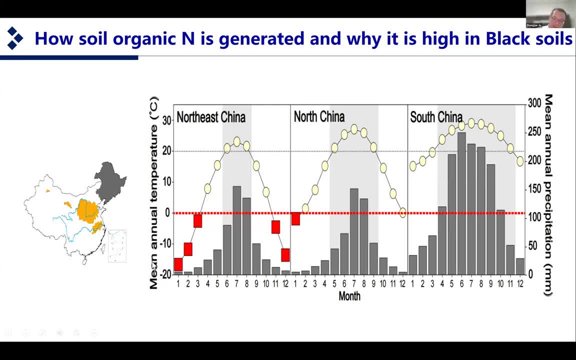 largely speaking in China. So this y-axis is the mean annual temperature. This left side, the red side, is the mean annual precipitation. So we can see clearly. so in northeastern China, most of the precipitation under the precipitation here, here is the temperature. hostile temperature could occur in summer. 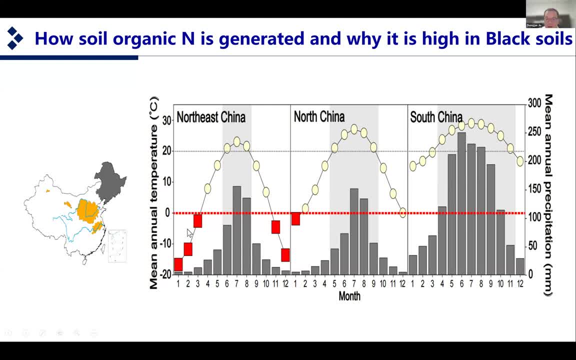 from June to August And for the rest of the year the temperature is almost, I mean, below 0 degree. but in southern China the situation is comparable, ض definition completely different. We can see, the temperature is way higher than the stone cells degree and over the year there are lots of the precipitation. 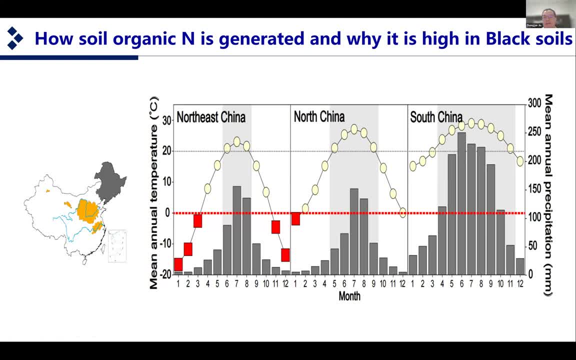 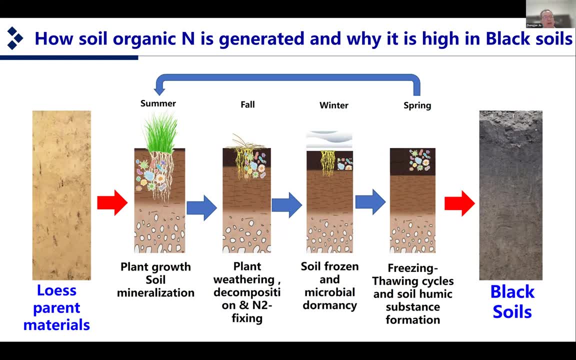 So the climate drives the formation of the black soil And then the loose soil is often, as Dr Prof Lin Zhang mentioned, loose soil is often considered as a parent material of black soil, and then in the summer the plant grows rapidly and the strong soil mineralization. 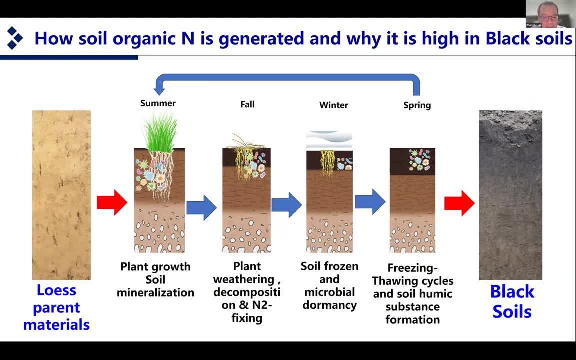 is going on because of the high microbe activity and the high temperature, But in the fall the plant litter and the residue started to be decomposed by organisms and the free living nitrogen fixer started to work, because the plant biomass usually lacks nitrogen. 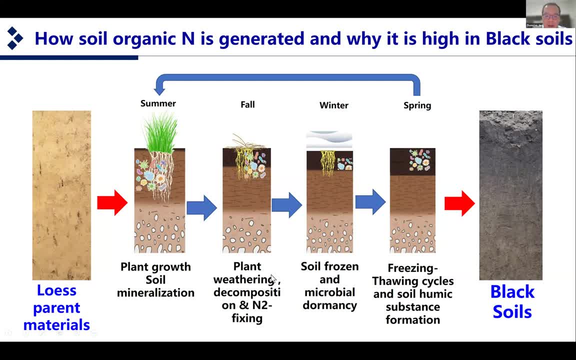 And this is a key source of the soil- organic nitrogen, ranging from the black soil. And in the winter, because the soil is frozen and the microorganisms come into the dormant for rest, and in spring, the repeated cycles of freezing and the thawing cycles start to work. 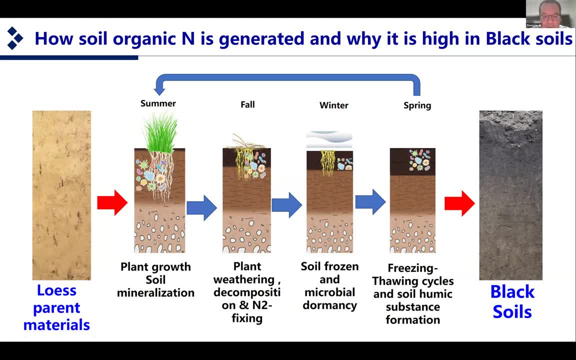 and the plant residues cannot be decomposed completely. Therefore the soil humic substance with high nitrogen is formed and the color is getting dark because of the incomplete decomposition and the formation of the black humic substance, as Prof Zhang mentioned before. 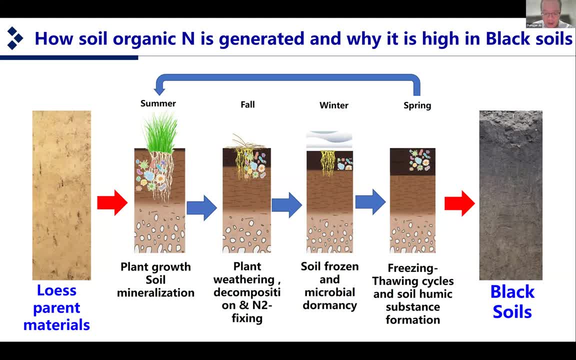 And, in summary, the high organic nitrogen depends on the two points. One point is that in the summer there is a large amount of plant biomass in the soil, And number two, this large amount of plant biomass cannot be completely decomposed under the cold, temperate climate in northeastern China. 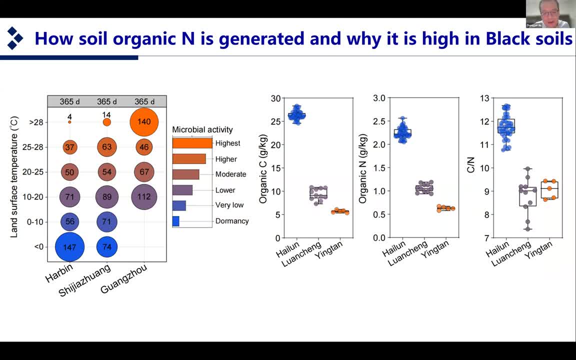 I also would like to show you specifically how black soil is formed, why soil nitrogen is high. You can see in this figure this is northeastern China. This is southern part of China. So one year has 365 days, So you can see almost half of the year. 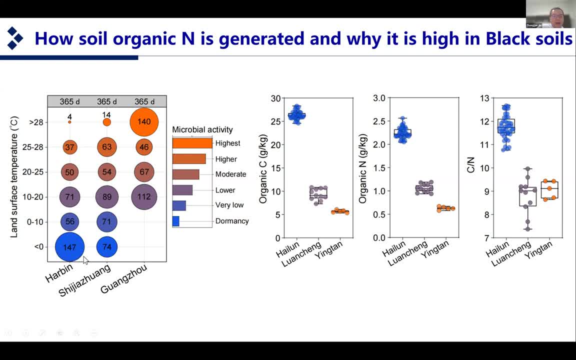 the temperature in northeastern China is below zero degree. So the organism is almost resting over there. It has nothing to do but rest. But also the other point: you can see, organic nitrogen is much higher in northeastern China than in southern China and north China. 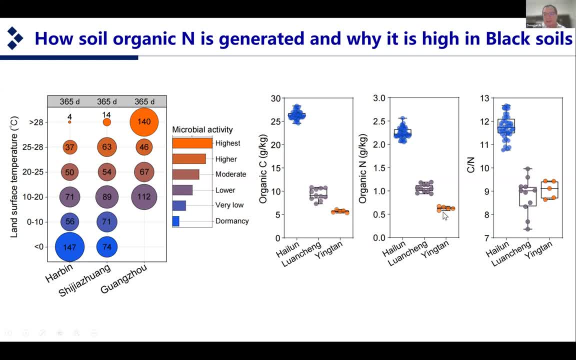 And organic nitrogen is also very high, as I said before. But it's interesting, I would like to have your attention. The carbon to nitrogen ratio is also very high in northeastern China. It means it has two implications. One implication: the black soil has very high organic carbon. 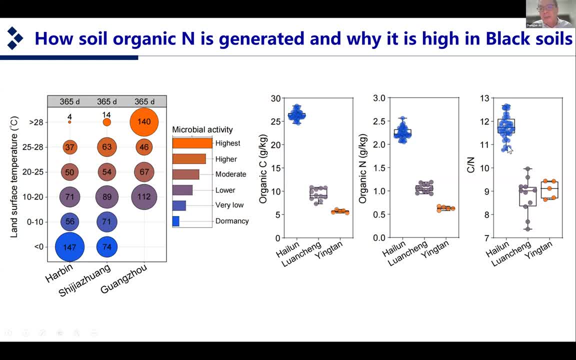 Therefore, even though nitrogen content is high, but the ratio is still low. So, as we know, the plant biomass has a carbon to nitrogen ratio normally more than 40. And the organism has a carbon to nitrogen ratio below 30. And the black soil has a carbon to nitrogen ratio around 12.. 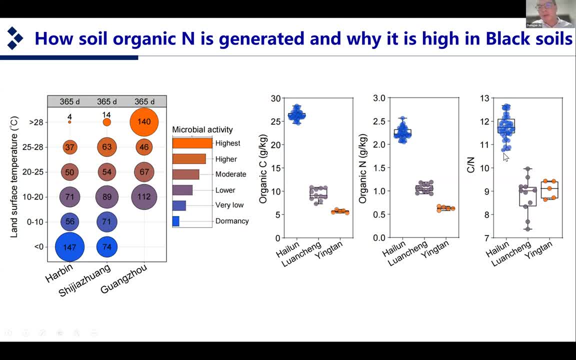 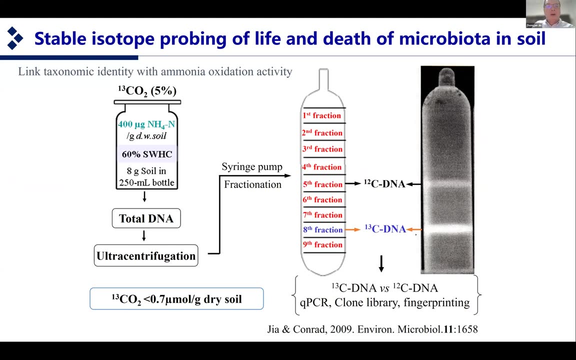 So the implication is that most soil organic nature is likely from the dead microorganism organism in the soil but not from the plant residue. So in this part I would like to say how we use stable isotope probing to probe the life and death of the microorganism in soil. 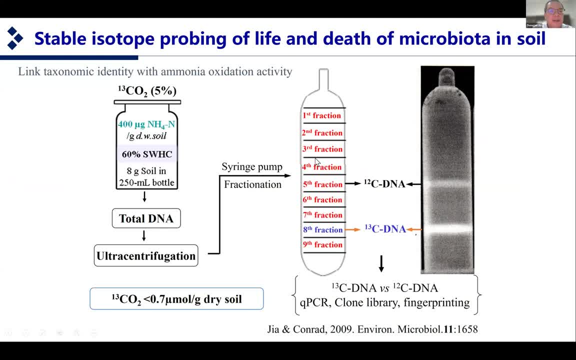 And then we can link the taxonomic identity of the touch of the microorganism with its functional activity. It's very simple: We just incubate the black soil with a labelled substrate, nitrogen-13-CO2.. And the microorganism in the soil 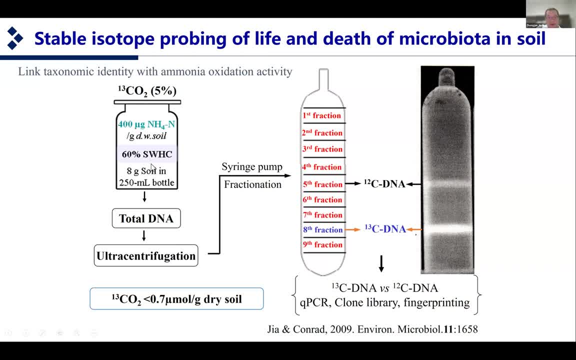 will assimilate the organism in the soil that assimilates. the labelled substrate would be getting labelled, I mean the DNA would be getting labelled. And then we are going to do the ultra-centrification. We can resolve the 13C DNA from 12 DNA. 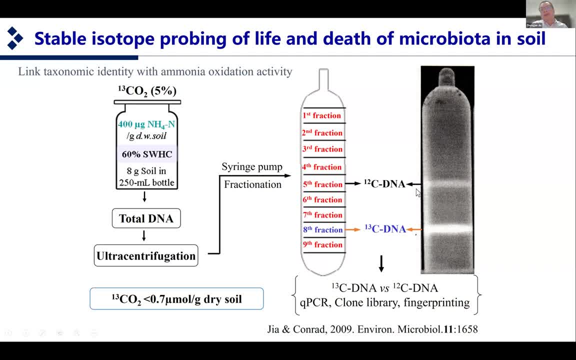 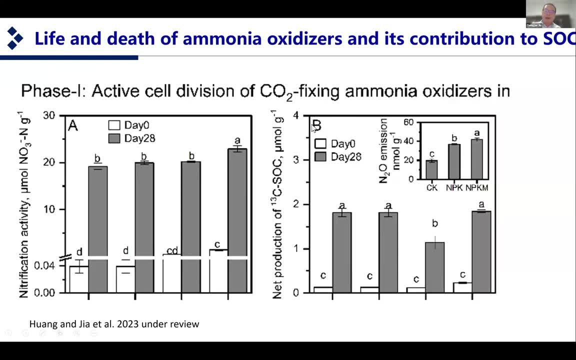 of the labelled microorganism that do not utilise the labelled substrate. So it's very clear. we have the two phases. The first phase is we incubate the soil with 13-CO2.. We can see we have a very strong or full soil. 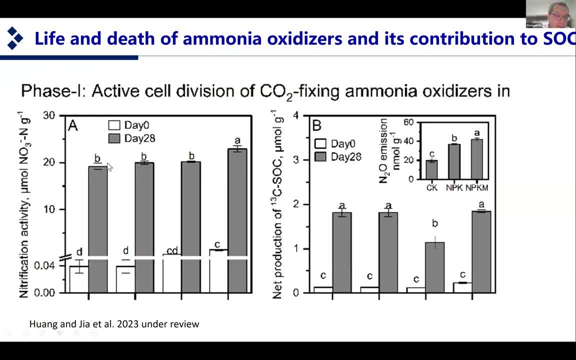 We have all soil, compared to the day zero. We have plenty of nitrate production. It implies strong nitrification activity. Correspondingly, you can see there is a strong nit production of 13C- labelled soil organic carbon, in this black soil. 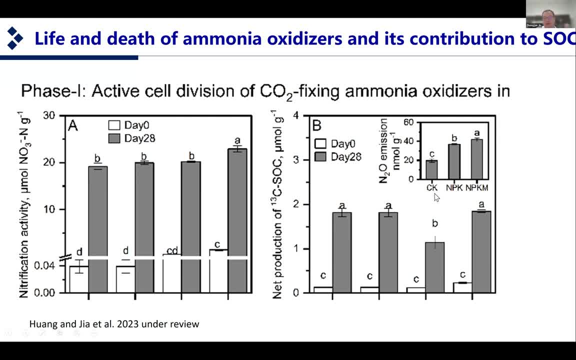 So the first soil that receives the first CK, soil that received no fertiliser, and the NPK means the soil that received the chemical fertiliser- chemical fertiliser for the last 30 years And this NPK M soil represents the black soil that received the chemical fertiliser. 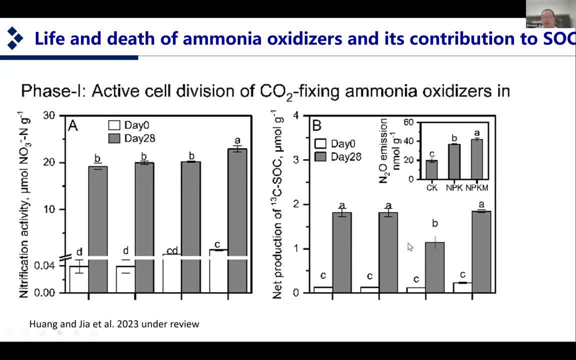 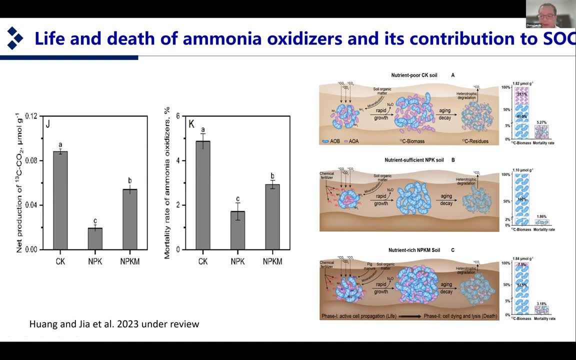 and manure. All of the soil has accumulated a large amount of the soil organic carbon. This carbon is actually from the CO2 fixing ammonia oxidiser. This is our first step. Our second step is because we know there is plenty of the newly. 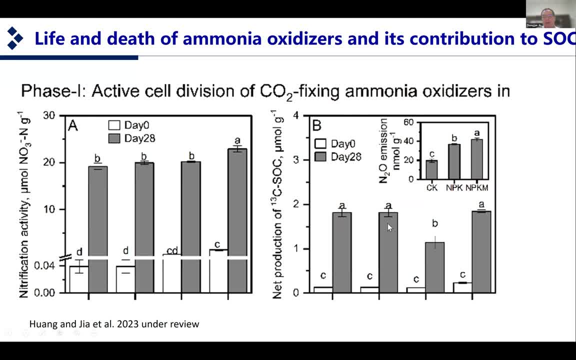 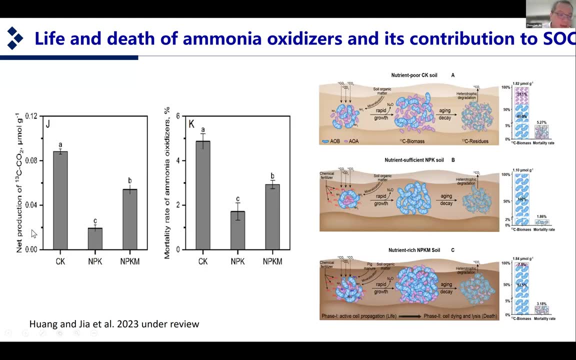 imported soil organic carbon. This carbon is from the newly generated CO2 fixing ammonia oxidiser. And then we incubate this newly generated ammonia oxidiser and you can see that if the microorganism is going to die, the organism will be decomposed. 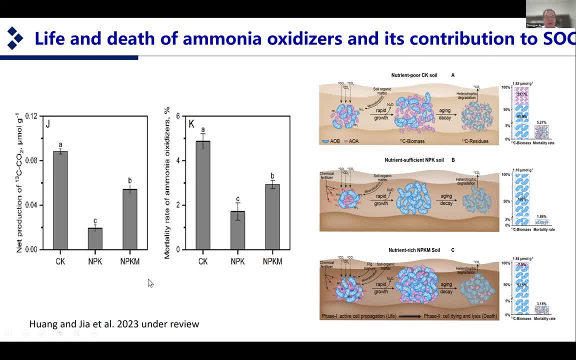 because of the 13C CO2.. We can see these three soils, all of these three soils have released a fraction of the 13C CO2 from the black soil. This is our result. It indicates there is a 5% of the newly generated. 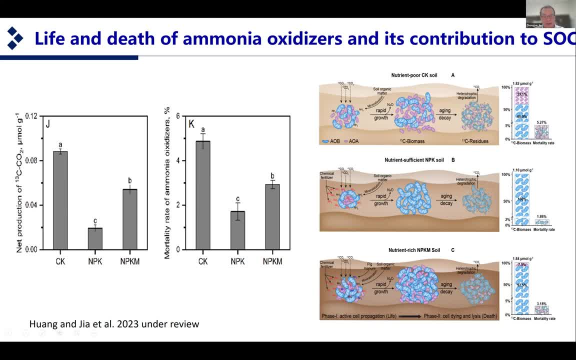 microorganism has died and it was completely decomposed to respect the 13C CO2 for the 3K soil, But for the NPK soil it's relatively fertile. There is only 1.8 or 1.9%. 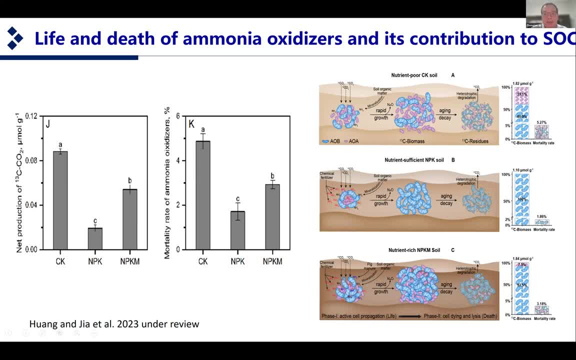 of the newly produced ammonia oxidiser microorganism is decomposed to 13C CO2.. It means it's dead. It is dead And for the soil with NPK manure soil it's up to 3.18% of the newly generated. 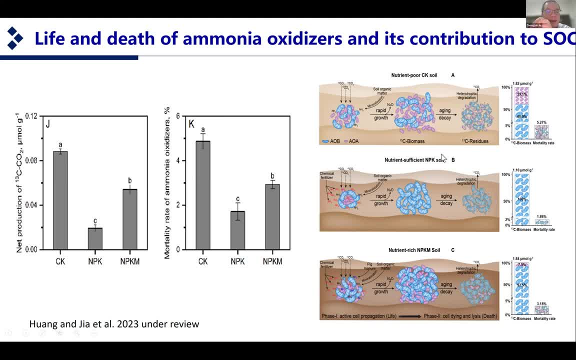 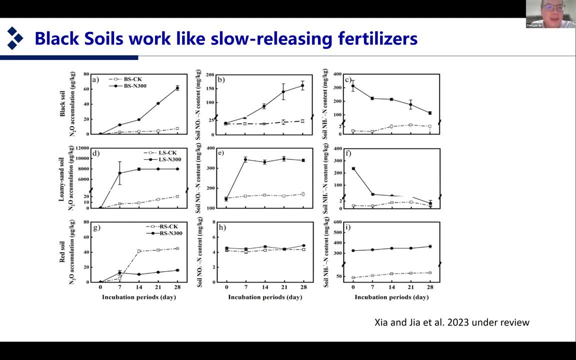 fresh ammonia oxidiser has been aging to death. So this is the other study I would like to show you- It's a case study- why the black soil is very important. It works like the slow releasing fertiliser. You can see, this is the black soil. 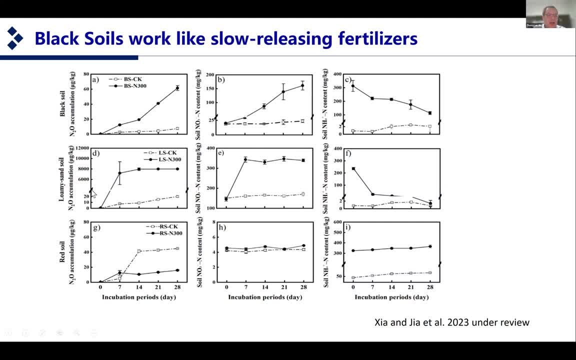 This is the loamy soil which is in North China, close to Beijing. This is the red soil in the south of China, So we added the 300 ppm ammonium- urea ammonium into this soil. So the CK means there is. 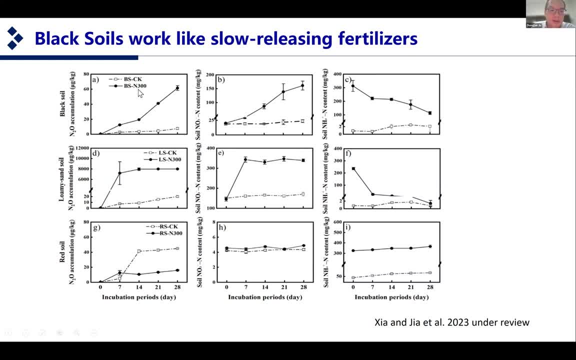 no addition of the ammonium, The 300, nitrogen 300 means 300 ppm ammonium. You can see, for this black soil the nitrate production is slowly going up, But for the loamy soil in North China, close to Beijing. 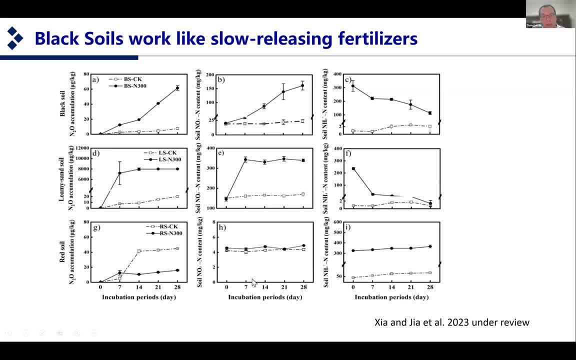 the nitrate production immediately goes to the peak for one week, seven days, And then it stays at the plateau. But for the red soil there's almost no ammonium transformation, So it means the ammonium in the black soil can be slowly released. 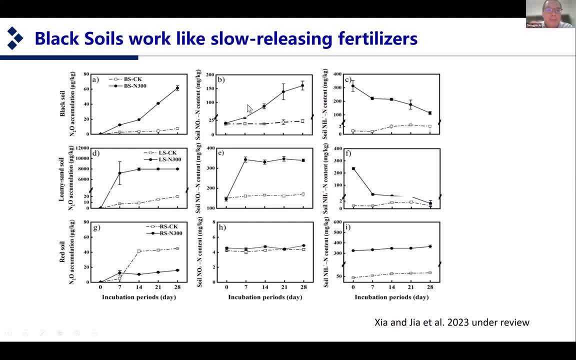 Either it is directly utilised by the plant or it is slowly transformed to the nitrate, then assimilated by the plant. But why is it important? Because if its ammonium is quickly transformed to the nitrate, as we know, the nitrate 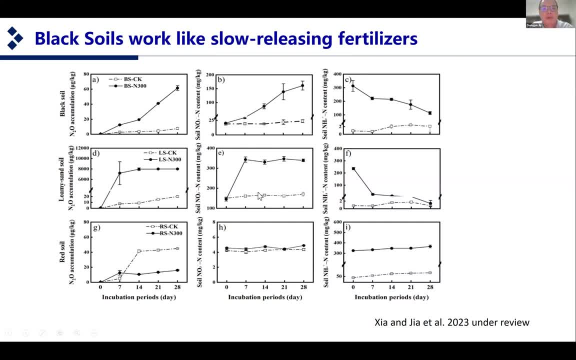 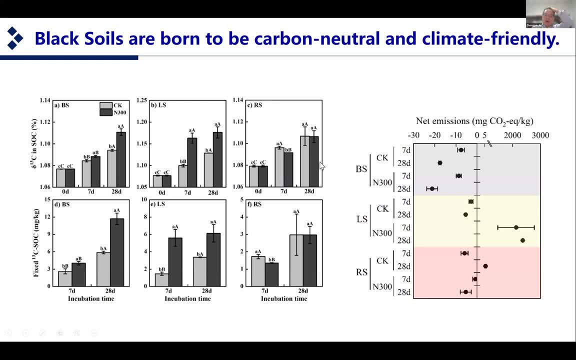 is very much mobile. it can be leached into the groundwater, leading to the pollution. And then this also, you can see, the black soil is born to be carbon neutral and climate friendly. As you can see, this is black soil, this is loamy soil. 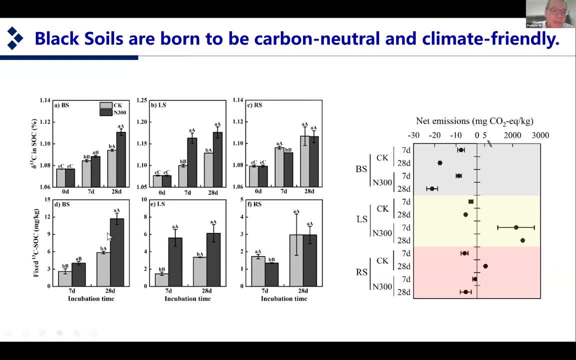 close to Beijing, This is red soil. in southern China You can see this YX15, this is eternal. this is feld, So the black soil. if we add the fertiliser, it can also fix a large amount of CO2. 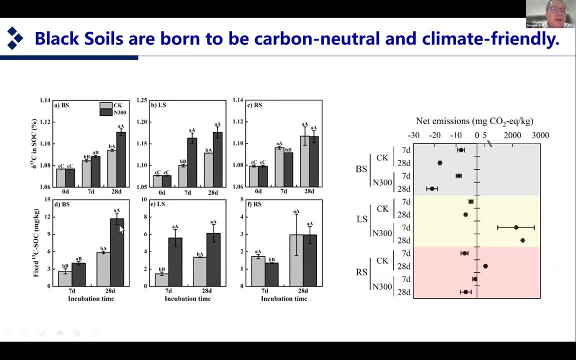 and then soil. organic carbon is increasing rapidly, But for loamy soil it also increased, but not that high, And we also know that fertilisation will lead to the N2O emission. So we do the black soil, loamy soil. 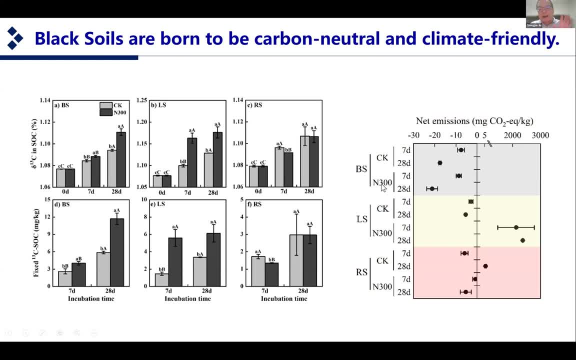 and red soil. You can see, even though we applied a large amount of fertiliser- 300 ppm, so still the net emission of greenhouse gas is still negative. But for loamy soil, clay soil, in the region close to Beijing. 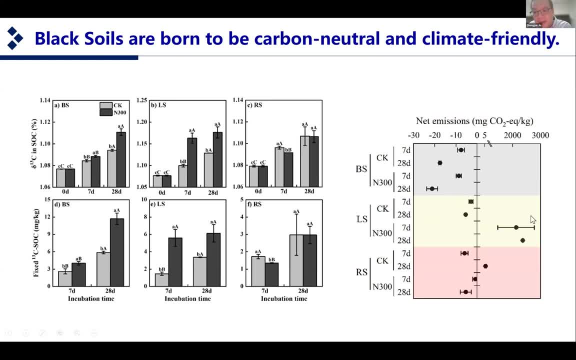 the net emission of the greenhouse gas is extraordinarily high. You can see, this is 2000,. this is just feld. So you see, the black soil is born to be carbon neutral. It's really, it's really surprising. I was also. 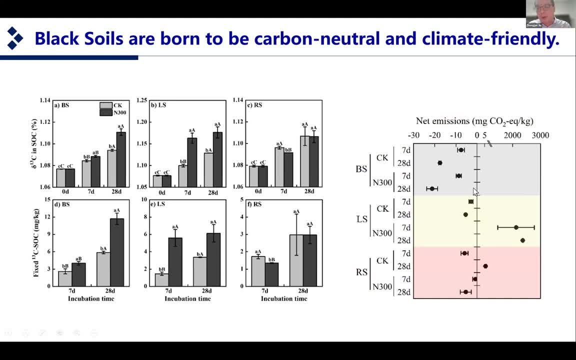 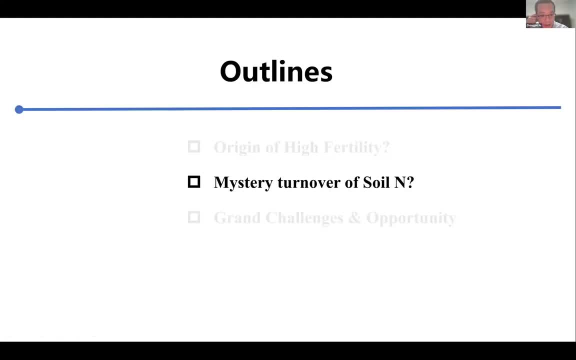 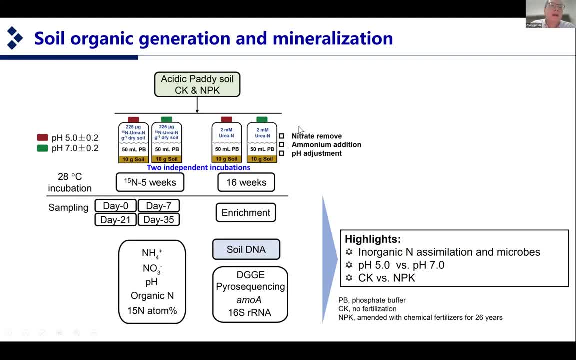 over. So we incubated two paddy soils, And one is the one soil received the low fertilisation in the last 30 years, The other soil that received the chemical fertiliser for the past 30 years. And then we incubated. 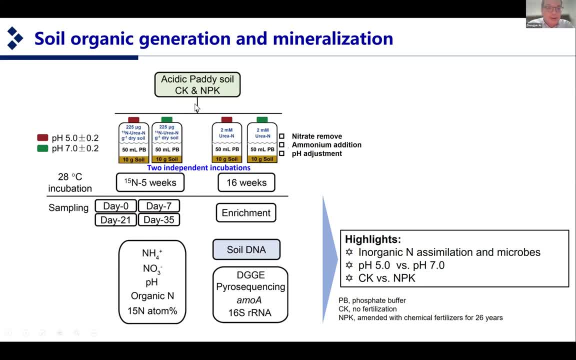 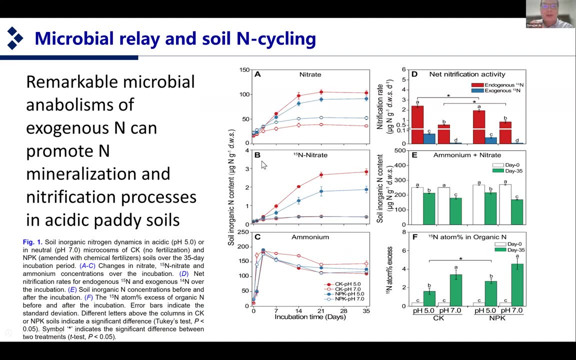 these two soils with the nitrogen labelled ammonia and then for the seven weeks. So you can see, so we incubated these two soils with the nitrogen labelled ammonia and then because of the ammonium is 100 ppm. 100 ppm ammonium is labeled. 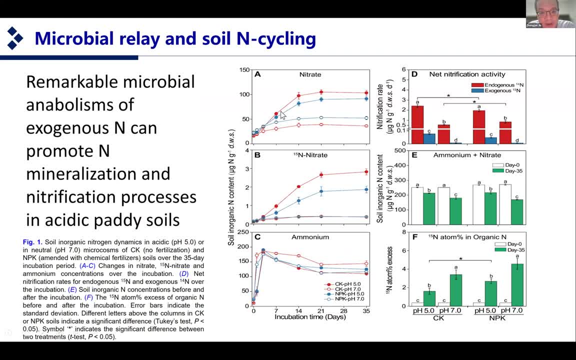 But then we see plenty of the production of the nitrate, But we can see only there's 100 ppm, almost 100 ppm and 15 ppm, But for the labeled nitrate there's only two or three ppm labeled nitrate. 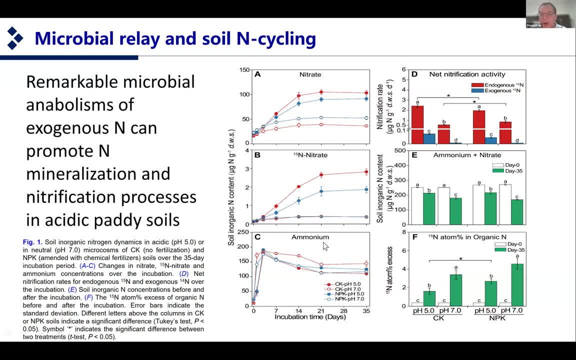 And then the ammonium concentration is also relatively high. So I would like to go to here, you can see. So the majority of the added ammonium labeled has been absorbed into the soil. organic nitrogen. You can see this is one soil, CK soil, NPK soil. 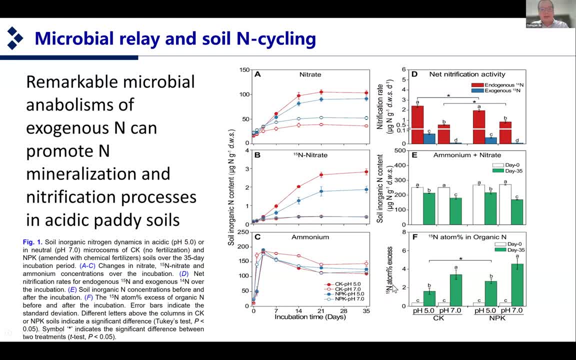 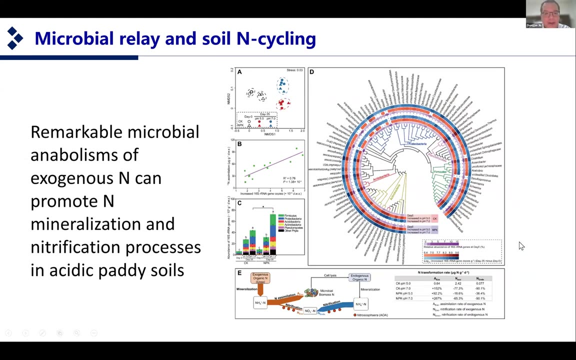 The after 35 days incubation, the nitrogen atom excess is extraordinarily high, because the background is only 0.336, but now it's almost two, four and almost 5% of the nitrogen atom excess. So we feel that. so we feel. I would like to show you the this: 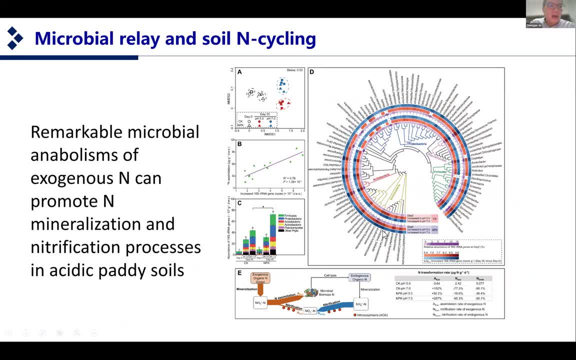 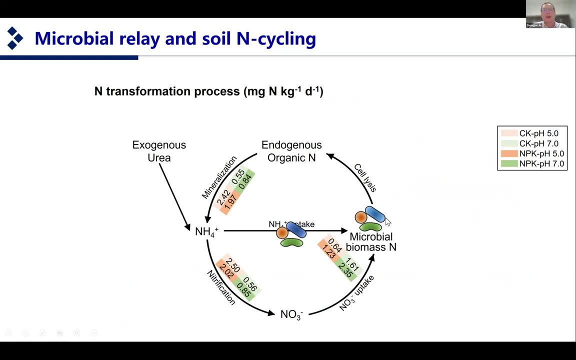 I would like to show you this, our conclusions, that remarkable anabolism of the exogenous nitrogen can promote nitrogen mineralization and the nitrification process in the paddy soil, in black paddy soil. So the key point is, I would like to show you 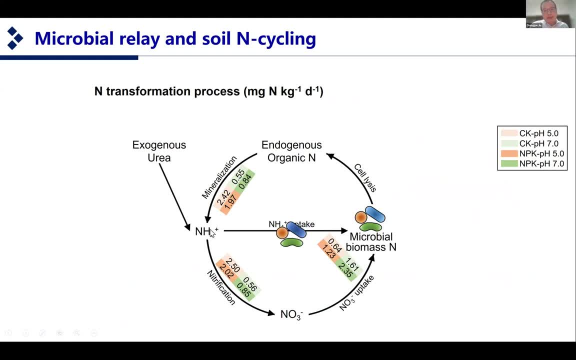 if we add the chemical fertilizer, like the urea, into the soil, so the nitrification is not stimulated. The majority of ammonium actually is assimilated by microorganism and the biomass synthesis is going off. Therefore the soil 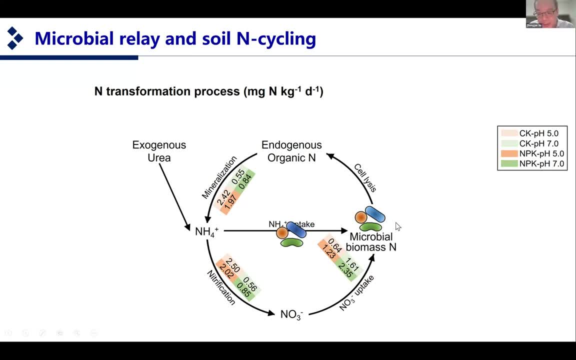 the organic nitrogen is going up. And then this: the microbial cell is dead After dead. so the cell is happening, And then lots of the soil. after the soil mineralization the inorganic nitrogen was produced, And then this inorganic nitrogen was again assimilated. 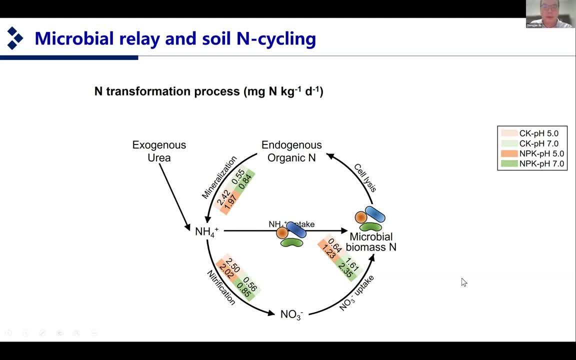 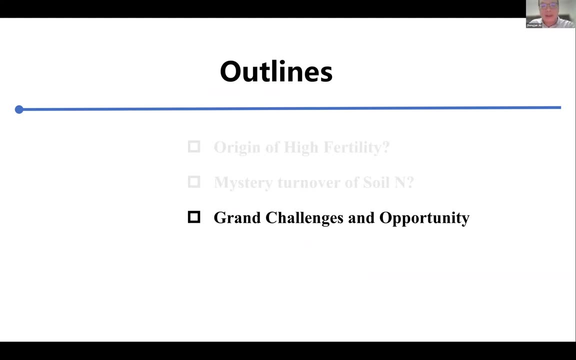 by the plant. I think this is very interesting. Unfortunately, our data is still not published yet. Hopefully, in 2024, we hope- it will get published. And then, in the final part, I would like to share with colleagues about the current challenge and the opportunity. 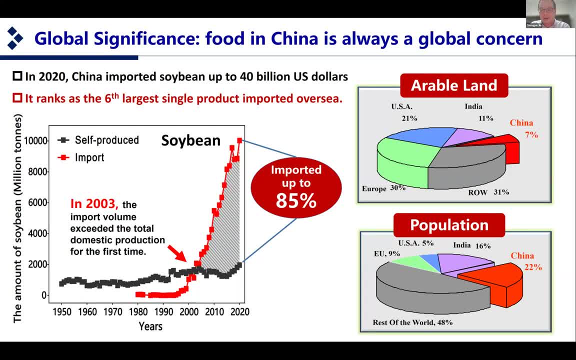 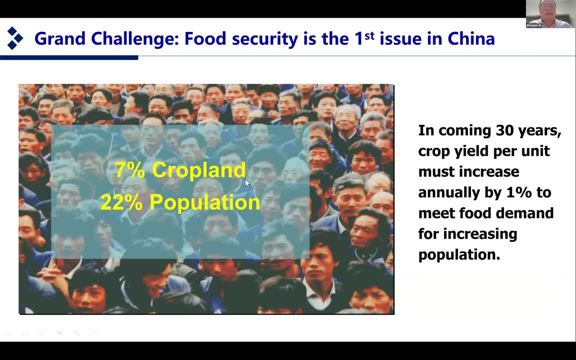 So, as you know, the food security is the number one issue in China, because we have only 7% of crop land across the world, but we have to feed 22% of the population in the world. And then you can see in northeastern China. 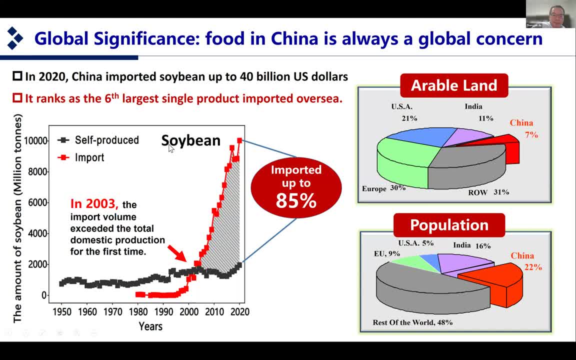 it's very important because more than 60%- 660%- of soybean was produced in northeastern China, And in 2020, China imported soybean up to 40 billion US dollars. It ranks as the sixth largest soybean producer in the world. 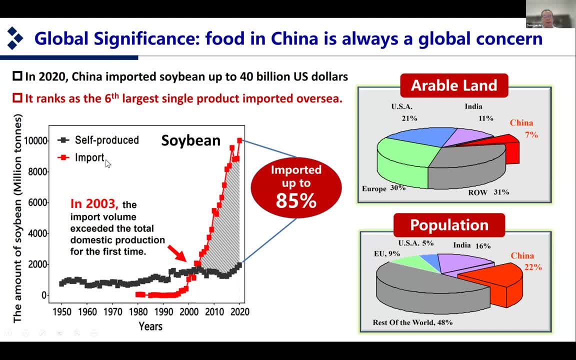 And it's a single product imported overseas. So you can see this soybean produced by China in the last 70 years. So the production is slightly increasing, but not that much. But this is soybean imported by China. You can see it significantly increased. 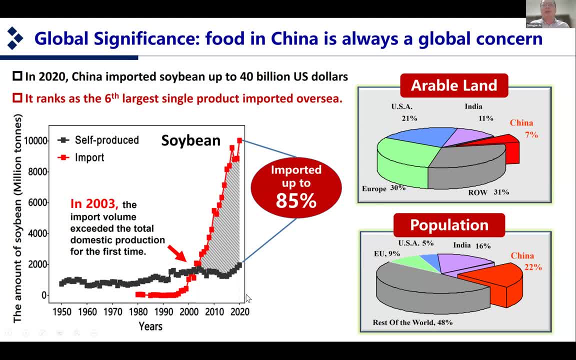 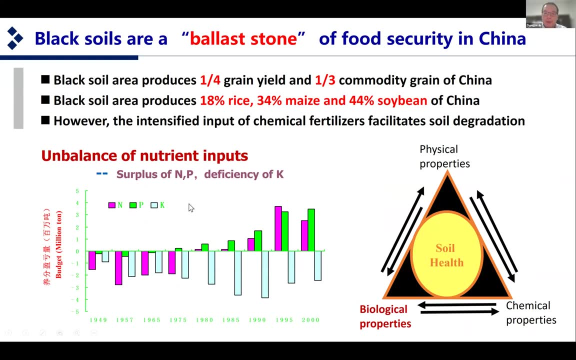 I think every year probably, we largely imported about 100 million tons of the soybeans. So so so, and then that also the black soil area in China. it produced 20%, 25% of the growing yield across China. 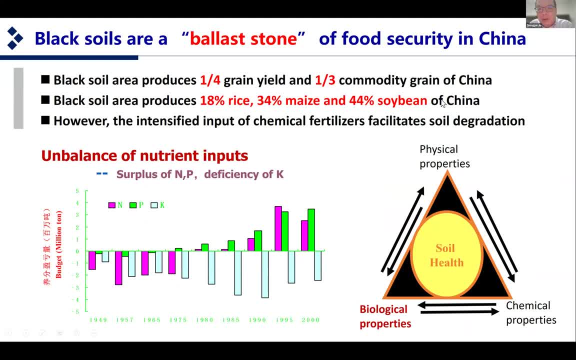 And almost one third of commodity grain of China And the black soil, as I mentioned. the black soil is also, but the problem is that we have the intensification of chemical fertilizers. So the problem is that we have the intensification of chemical fertilizers. 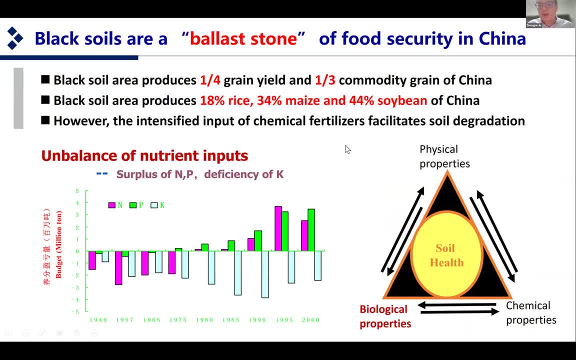 fertilizer input has facilitated the soil degradation And you can see in the soil in past 20 years, 40 years, the surplus, the unbalance of the nutrient input, the surplus of the nitrogen and the phosphate and the deficiency of the potassium is significantly high in the black soil. 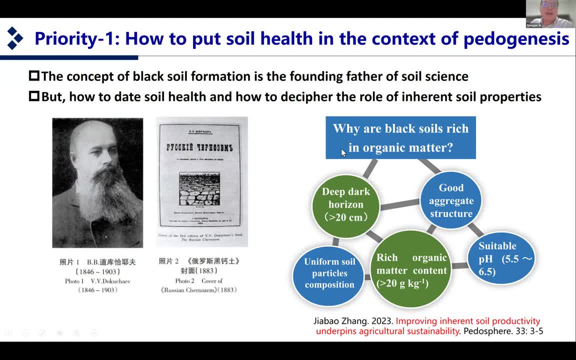 And then the priority for the future study. we feel there are three points. Number one point is how to put the soil health in the context of the pathogenesis, Because the concept of the black soil formation is the founding father of the soil science, as we said. 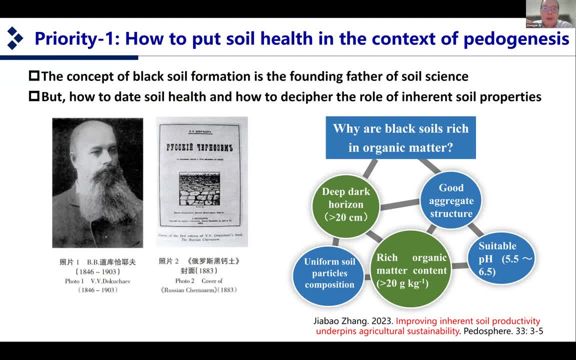 But still how to date the soil health and how to decipher the role inherent in the soil properties. I think is still it's a big problem Because, for example, we have no good index to probing or to measure the soil health. 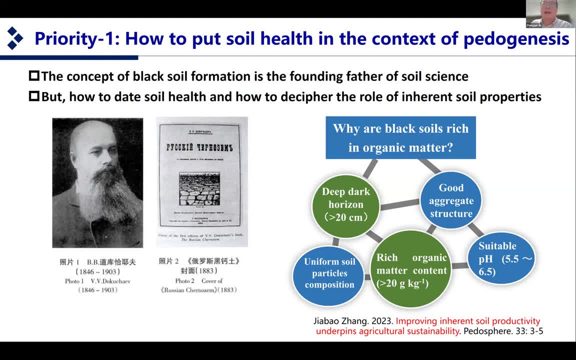 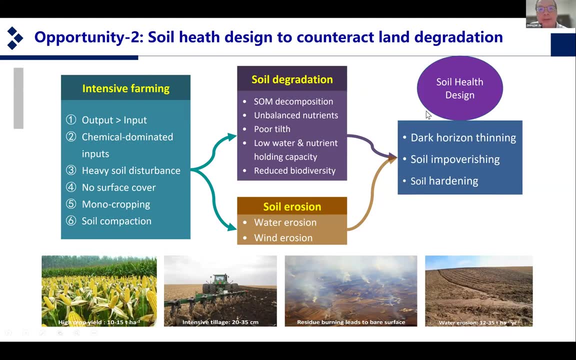 We feel the black soil is a good indicator, like, as I mentioned before, how nitrogen soil- organic organic nitrogen- is generated and released and then facilitated the plant growth And then the soil health should be designed to conduct the land degradation, as the doctor professor. 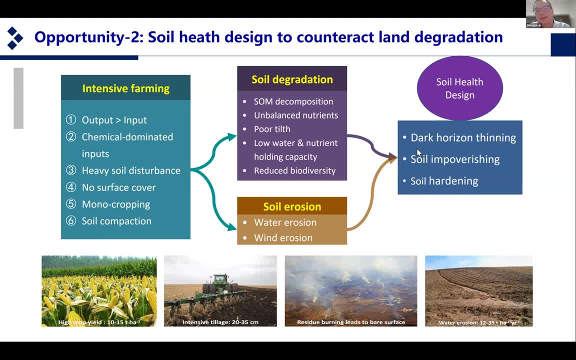 Tusheng Reng mentioned, We can see that the black soil layer is getting thinner and the soil organic matter is getting less and less and the soil structure is getting harder and harder. So this is a significant problem which is particularly important in Northeastern China. 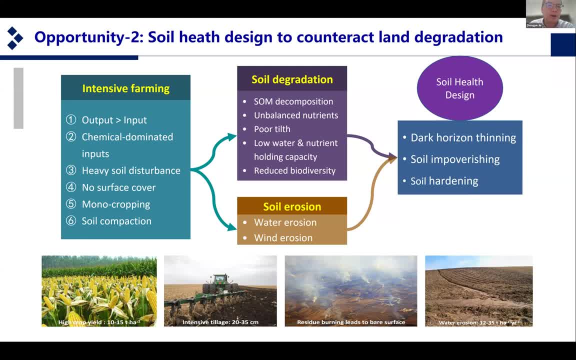 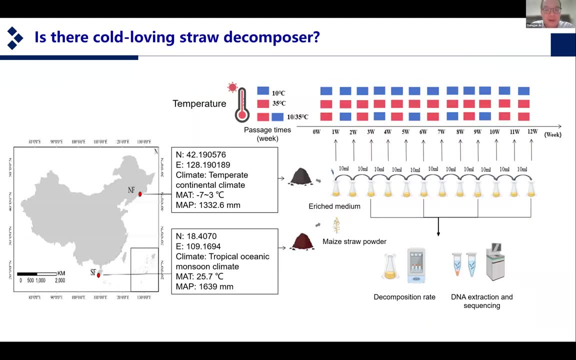 because it produced 25% of the grain across China. So there are lots of the input of the anthroponic panic interaction. So the final slide I would like to share with you about my interest. So is there a code loving straw decomposition? 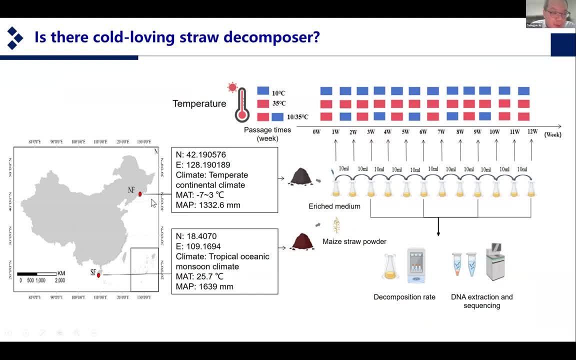 I would like to show you this in Northeastern China, where the black soil are located. So you can see, the mean annual temperature is about minus seven to three degree. So this is the tropical area in the Hainan province. The mean annual temperature is about 25 degree. 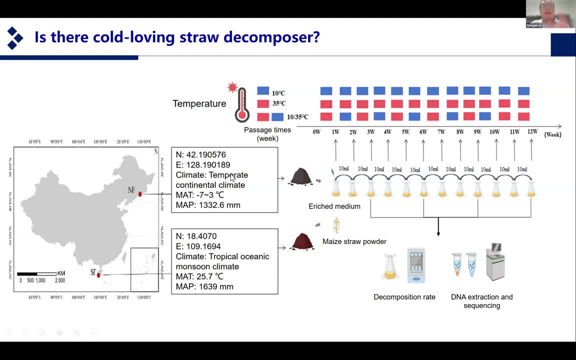 So we wonder whether there is because, as we discussed before, we feel the plant biomass decomposition is probably is a key source of the accumulation of the soil organic nitrogen production. So we wonder whether, in this low temperature, there is a specific code loving straw decomposer. 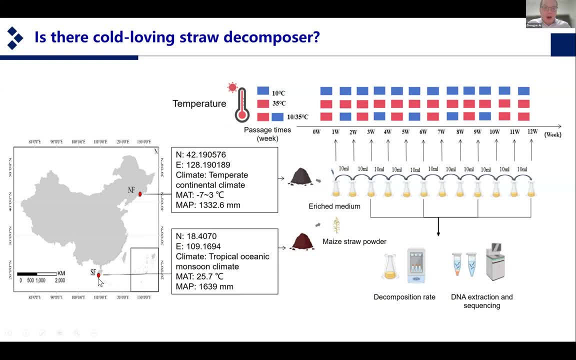 So we include the cold soil and the hot soil with the 10 Celsius degree, 35 Celsius degree, And then at the first week, second week and the 12 weeks, almost 12 weeks, And then we enrich the straw decomposition microorganism. 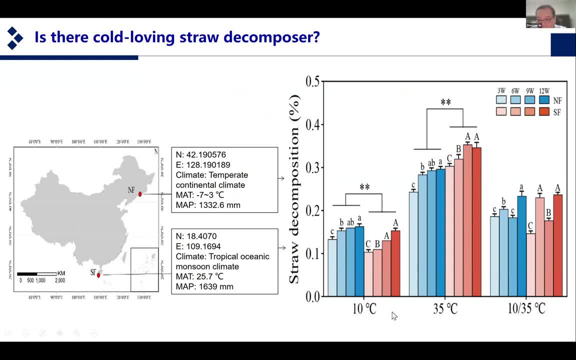 You can see. this is very interesting. So this is a code soil from the Northeastern black soil. This is code soil from the Northeastern China. This is the hot soil from the Hainan province tropical area. So you can see if we include this two soil. 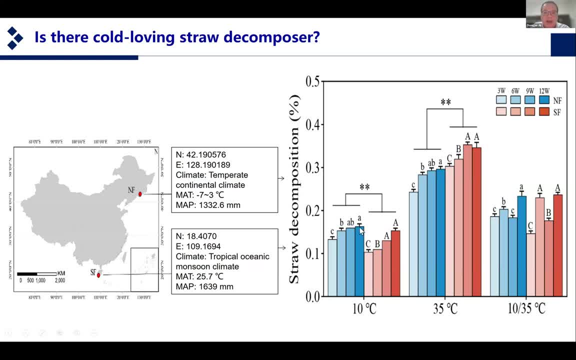 at the low temperature the black soil has much higher straw decomposition rate than the hot soil. But if we include the hot soil and the 35 degree and also the black soil in the 35 degree, generally speaking the tropical soil has higher straw decomposition rate than the black soil. 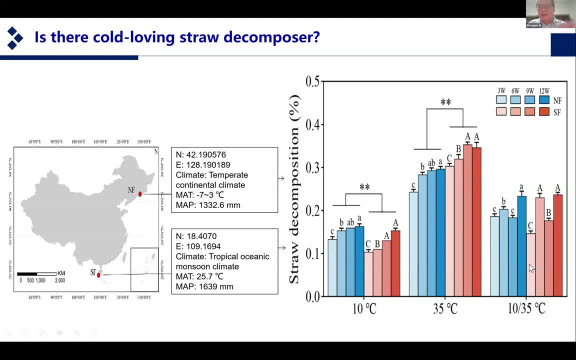 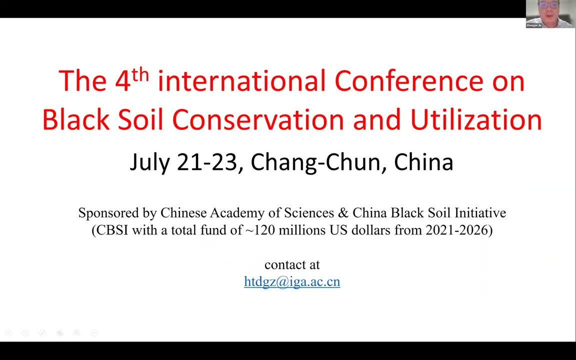 So, but for the trend, the pattern is a very much confusing for you if there is alteration of the temperature, the low-temperature and high-temperature incubation. So my fellow PBD I would like to share with you. in this July we are going to organize the 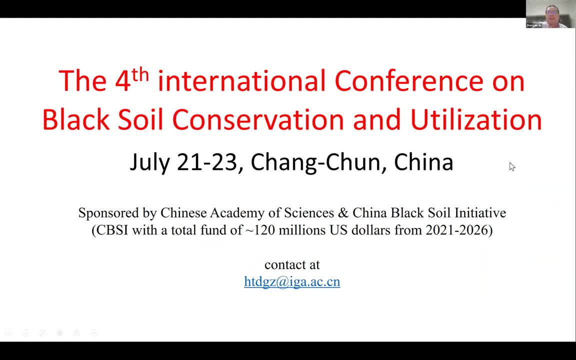 fourth international conference on the black soil conservation and utilization. So in this July in the northeastern China. this conference will be sponsored by the Chinese Academy of Science and the China Black Soil Initiative. This China Black Soil Initiative, CBSI, is called the CBSI. we have the total fund of the 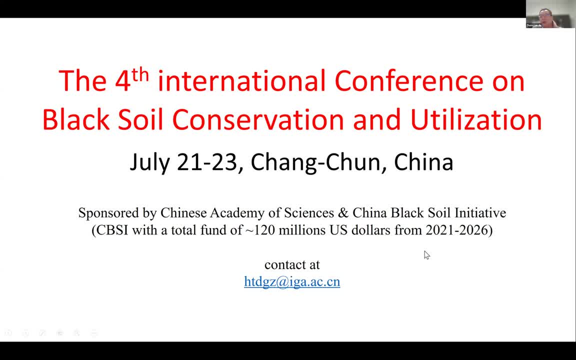 120 million US dollars from 2021 to 2026.. So we invested a lot of our money. We have we probably, as far as I think, many of my colleagues, like Dr Professor Gan Yinzhang and Tu Shengren, also joined us for this event. 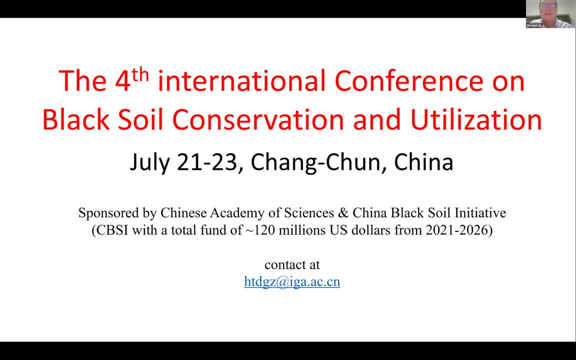 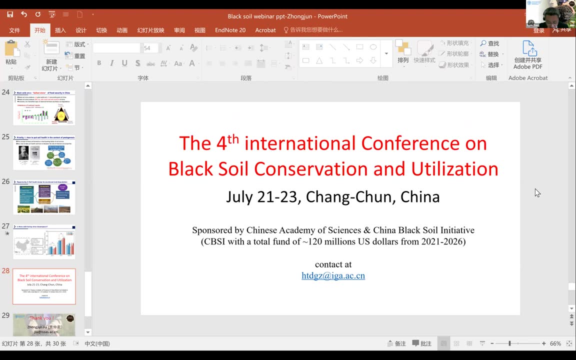 In it. we think we have made some very impressive achievements in the past few years. Thank you very much, Yu Xin. This is all my talk. I'm very happy to share with my work with colleagues. Thank you very much. Thank you very much, Professor Jia, and your excellent presentation. 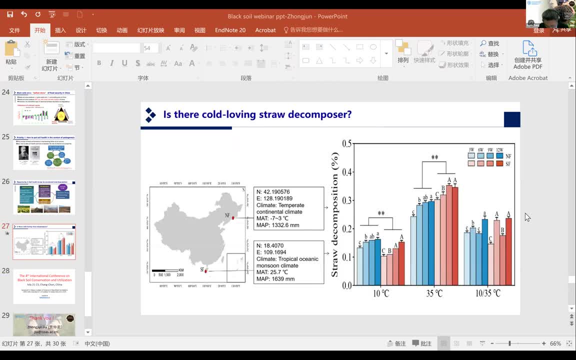 introduced the nitrogen-carbon dynamic on black soils And we you mentioned a very good point. I think it's very good. concepts like the black soils seems like a slow release of fertilizers. They can release so nutrients slowly and meet more demand of plant requests. 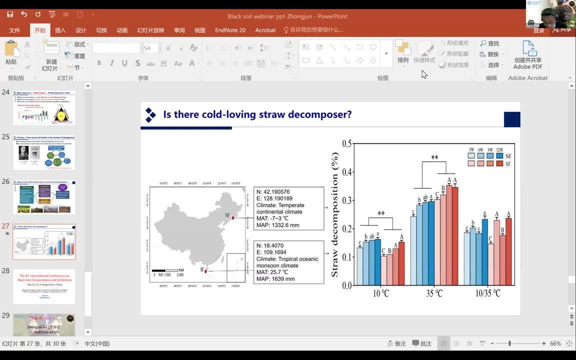 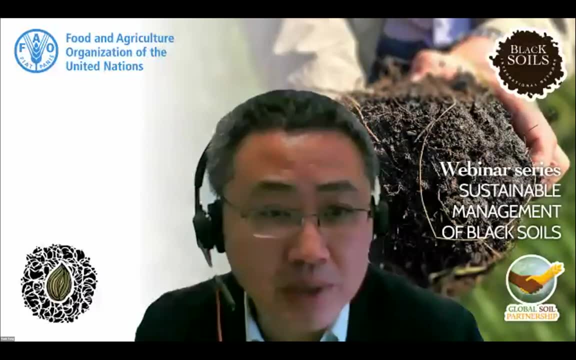 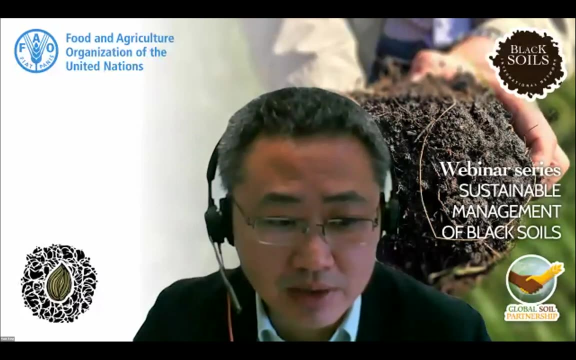 So that is a very good, good explanation. So thank you very much. Thank you very much for your presentation. And we also see there is big work in China to protect black soils and you have a big project And we are very happy that you, your institute and the Chinese government and also the Academy of 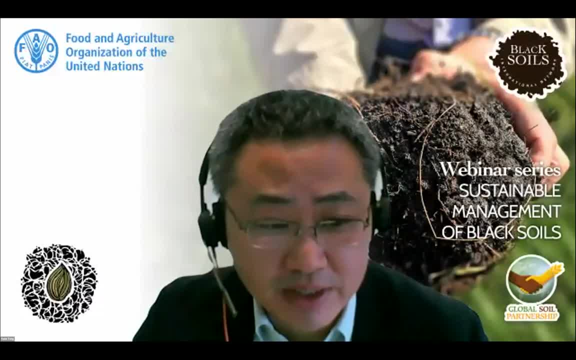 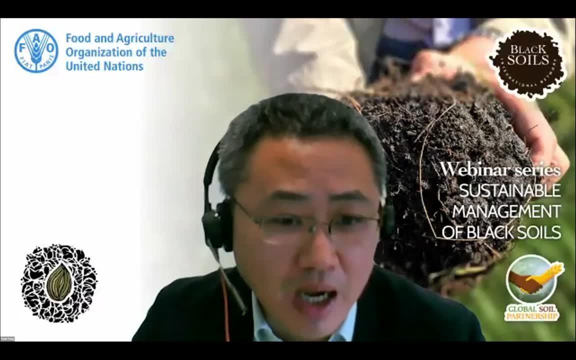 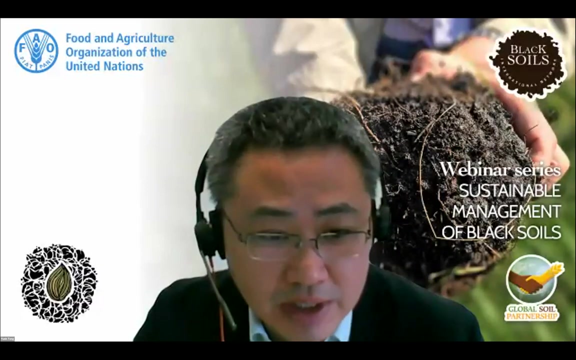 Soil Sciences of Academy working on this topic. Thank you very much. So I would like to take this opportunity to thank all presenters for their excellent contributions, And so now we can move to move on to the discussion part of our webinar. We will select questions from the audience and then try to answer as many as many questions. 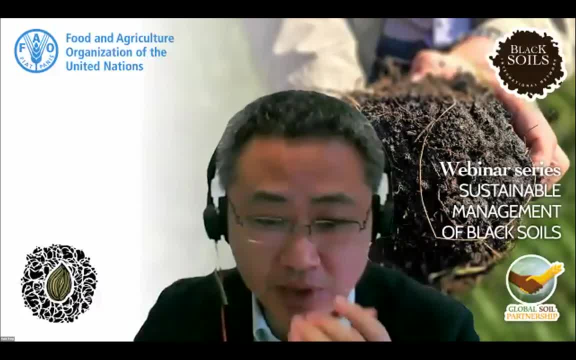 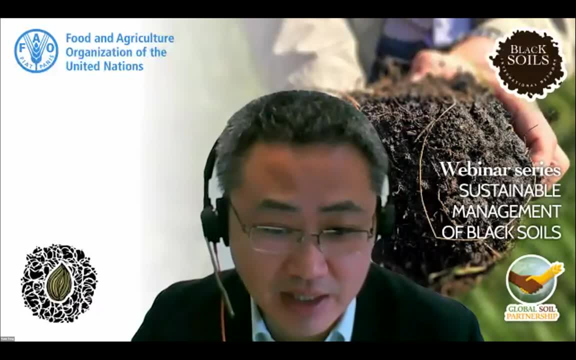 as possible. So I see there are many questions And so I think this is a very, very hot topic and our audience are very actively exchange with us. We are very happy. So now I would like to start from Professor Ganlin Zhang. some question to you. 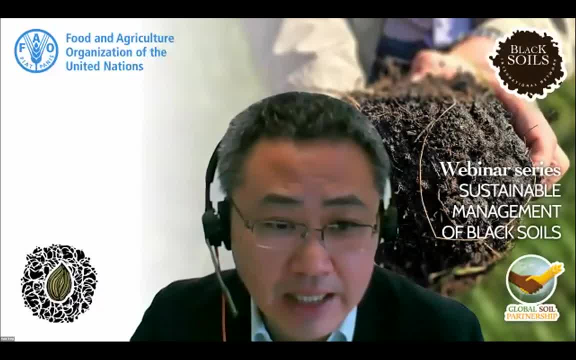 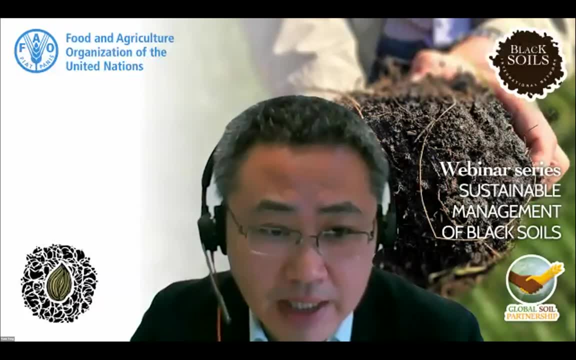 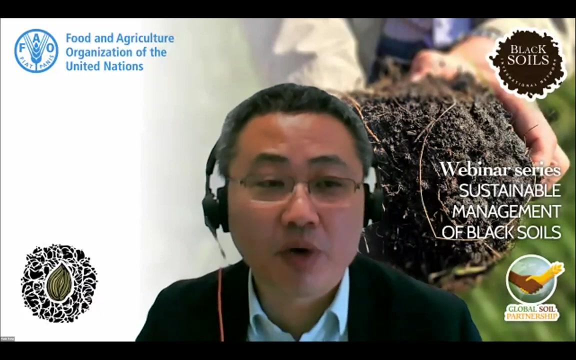 I think there is a question. I think there is a question about in what way could climate change impact the sustainability of black soils and the adaptation strategies are needed, how the climate change impacts black soils and their potential consequences. So, Professor Ganlin Zhang, because the formulation of 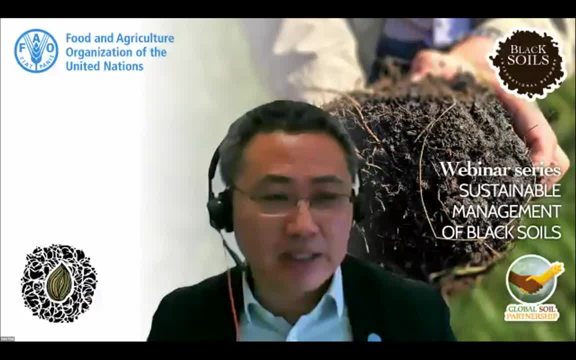 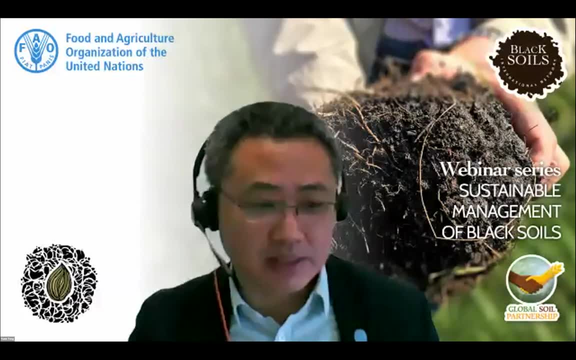 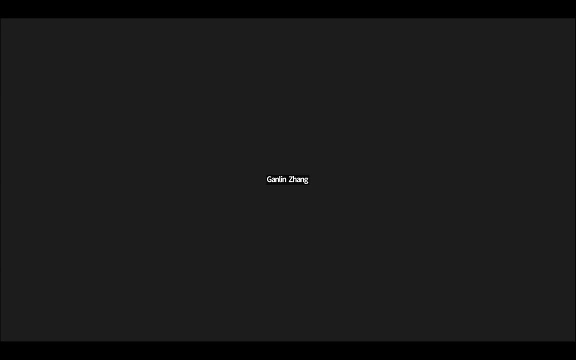 black soils, you explained. So is there some climate change in this recent year? Yes, So I think this is a very good one and it's a very big question. Well, first of all, I say the formation of black soil is dependent on climate. 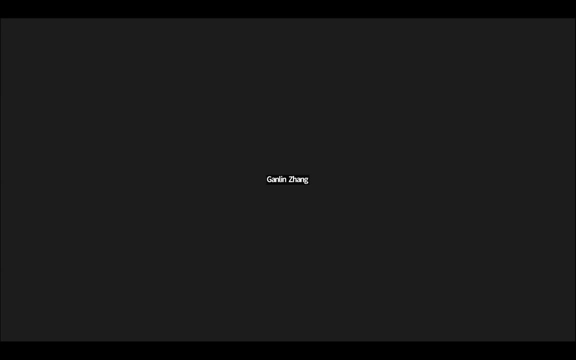 But during the glacial time and deglacial time, when temperature rise, only one temperature, temperature rise- it is possible. is it possible? it is possible for the formation of of organic matter. but now we are concerning more about the climate change nowadays. uh well, i i think, at least in in several ways, that climate change may can affect. 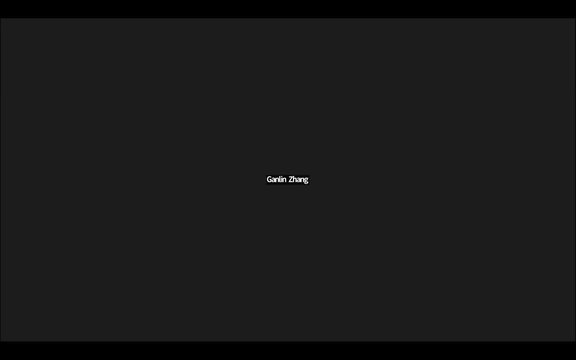 uh, the use of of soils and in general, of course, in also including black soils. first of all, we know, under climate change scenarios, um there will be more extreme weather condition, so including heavy rainfall and long-term growth and um so, uh, extreme in extreme in that temperature. so all those side the the possible. 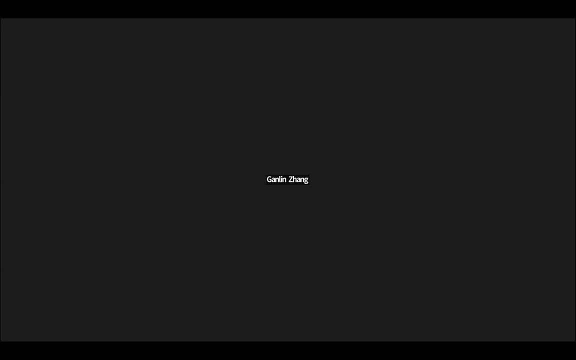 outcome of climate change. so this will have a very fundamental uh impact on on black soils. we know we we know black soil is vulnerable to soil erosion. so when we have a extreme climate, we have a heavy rainfall, then the uh the soil is uh subject to to be lost very quickly and um. 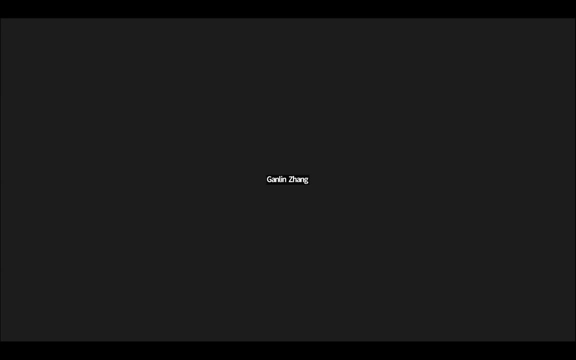 of course, when we talk about and this temperature rise, we know, with the shifting of climate zone to north, uh source in temperature, temperate and even cold regions, um, they are subject to very- uh, you know, very, very strong energy evaporation and they are also subject to. 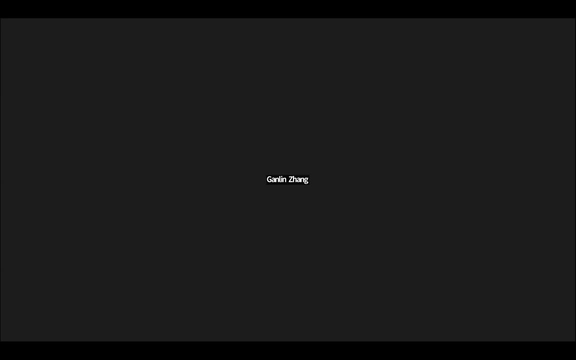 very strong energy evaporation and this will lead to rapid loss of soil getting matter and, of course, there will be a strong if, if we talk about strong, strong evapotranspiration and higher temperature Could be also a problem. So personally, I do not have a concrete study on this, but to my understanding, the future of climate change will have a negative impact on the use of black soils, on the sustainable use of black soils. 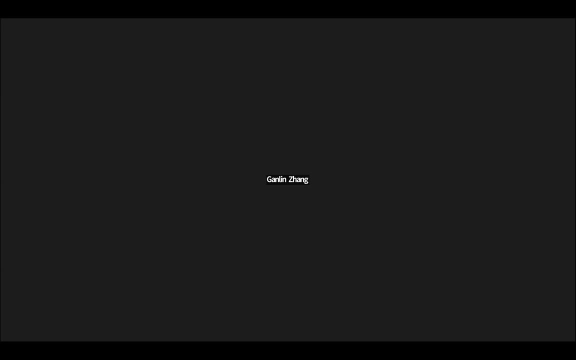 But we have to say temperature itself is a part of agricultural resources. I mean heat is also important. So when we have a bad temperature condition we may have earlier germination possibility. So the impact is not one side can be. 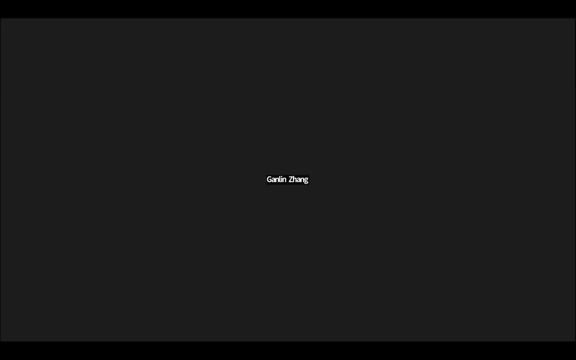 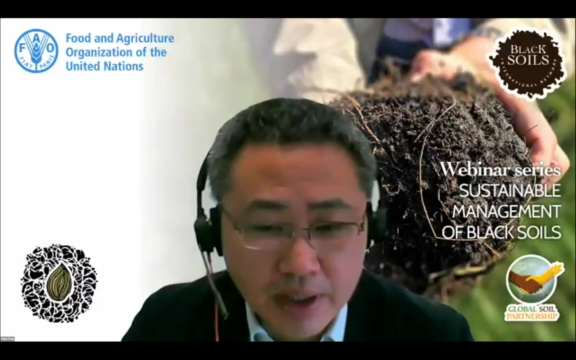 Complicated. So that's my very general answer to this question. Thank you very much, Professor Zhang, And I think another question I'm going to address to you is about: is there a difference between black soils and the vertigo soils? 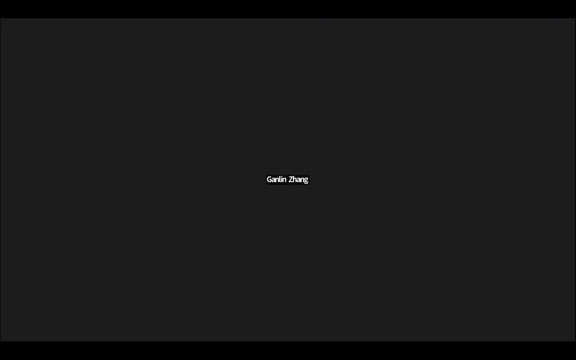 Oh sure, They are much different. They are much different. Well, Black soil is. the color is basically different. Is this the Wass kommt, or dato mas como o 가격? I think in Antan定inde 圧表 RAMPAD DOEH. 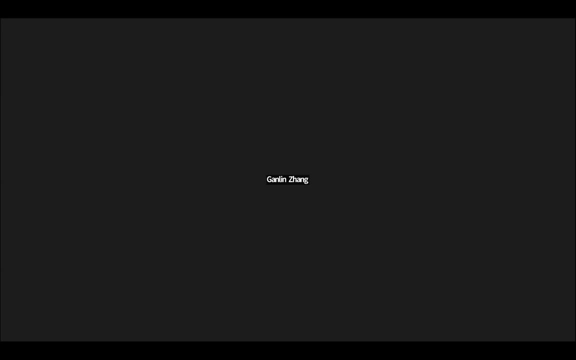 Pure material. material can be determined by the higher accumulation of soil, organic matter, and is well-structured, and it is the depends on the material is more or less, it can be or can be different, but more or less more homogeneous, and So the the texture is lonely to. 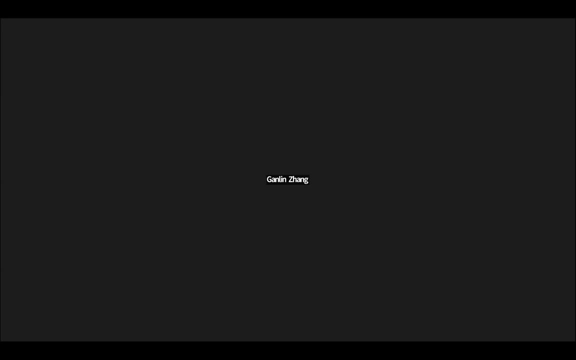 to more, more silt. it's um because of the, it is paramaterials and um it has um, has a low to medium calcium carbonate and uh, uh, well, well, it's, uh, it's, uh, uh. this is uh, more or less the the best and characteristics, but in terms of verticals, uh, we know the body source is higher. 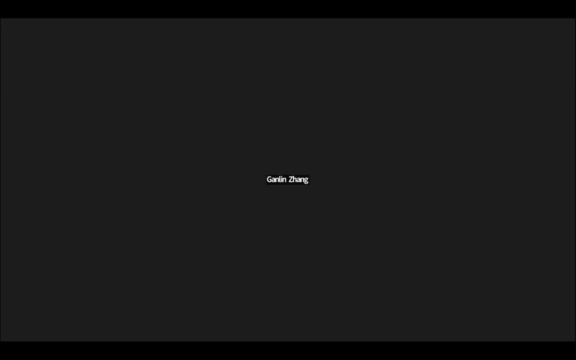 in in in clay and it is clear mineral is a so-called two-to-one um and uh silicate, um aluminum silicate, and it is due to this uh strong, uh water absorption absorption and capability, it can be um uh shrinking, shrinking and swelling, so uh, so so it. 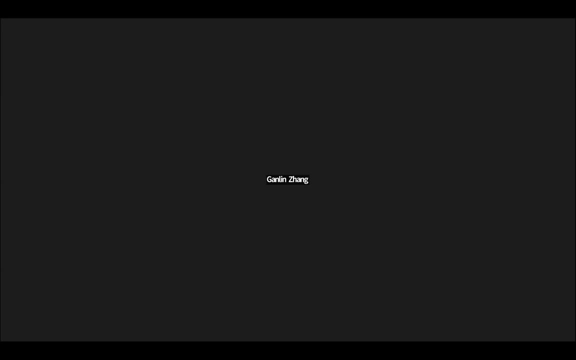 uh is a is a problematic, problematic soil and, um, though, uh, very soil is black, but it is organic matter is not high. that is because of the special, very special uh, um uh chemical problem, chemical futures of these uh, of these uh organic and inorganic complex, because, uh, it it is a, it is a it. 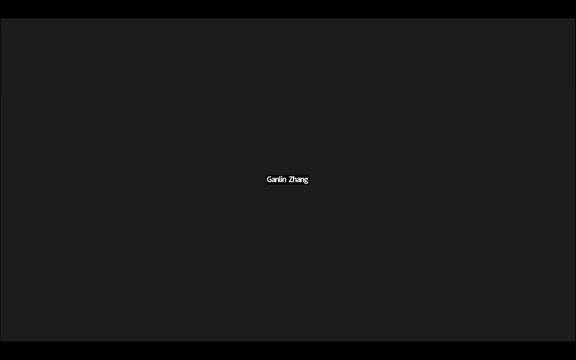 is the работать. there is a very, there is a very special um mechanism behind this um plant and other way. uh, black soil is uh oriented always not can can have um can have uh very difficult. uh, what management problem in fact it it is, it is um uh. 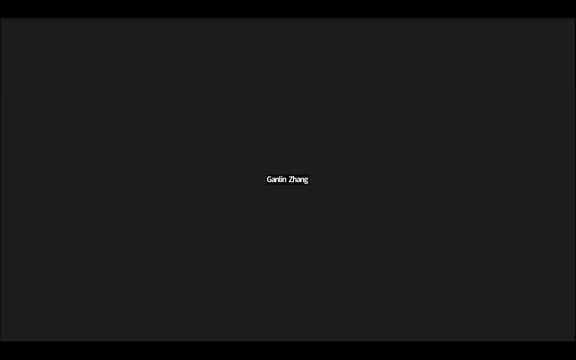 it has a very narrow, suitable word. uh. what content i mean in terms of tillage. If you have a higher water content then it can be very, very clay and the tillage is very difficult. And again, when it is lowered in soil moisture. 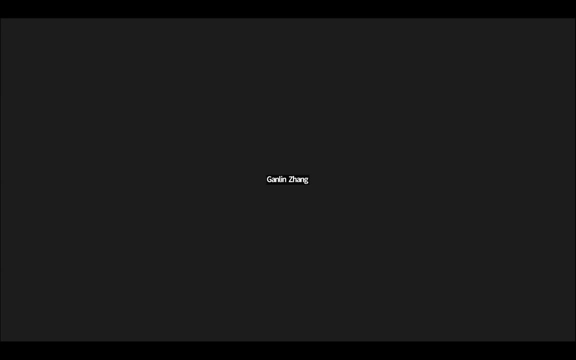 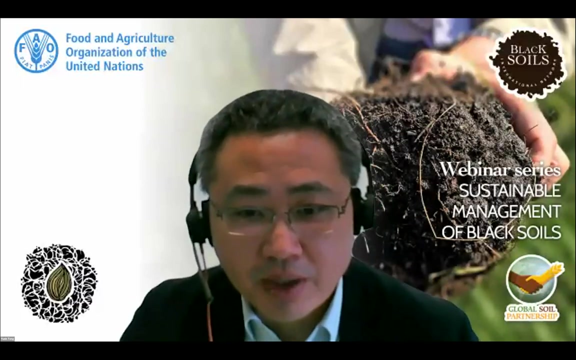 again it becomes very hard, very hard, and then it's also not easy for tillage. So these are quite different soils. Okay, thank you very much. Thank you very much, Professor Zhang, for your answers about the questions. So, thank you, thanks a lot. 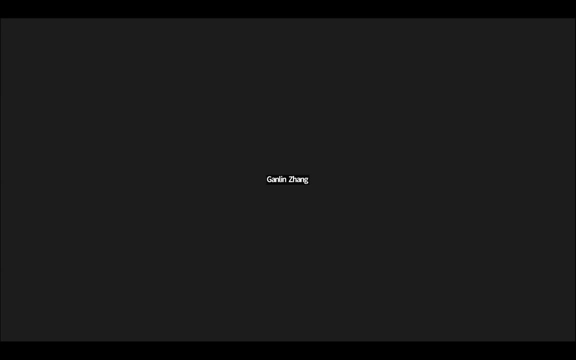 Now I would like to- Thank you. thank you, I also. yeah, yeah, yeah, we thank you for this quite nice opportunity and well, okay, thank you. Thank you, Professor Zhang. So now I would like to move to Professor Ren Tusheng. 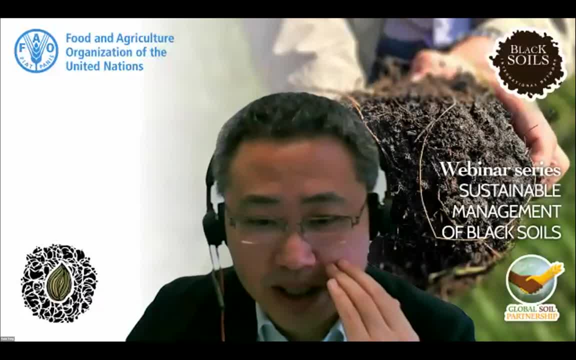 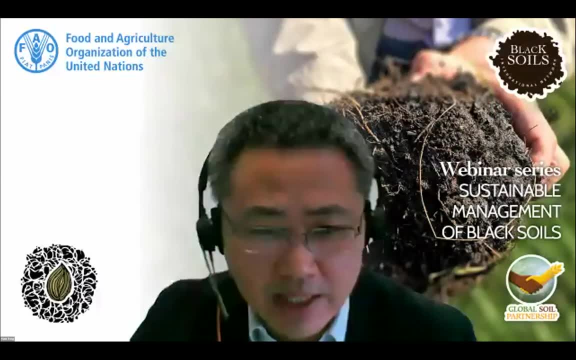 There are many questions about no-till tillage and the conservation agriculture of the land, Black soil use. So I think they are curious about the audience, curious about the traditional Chinese agriculture practices because you compare the traditional and the no-till. 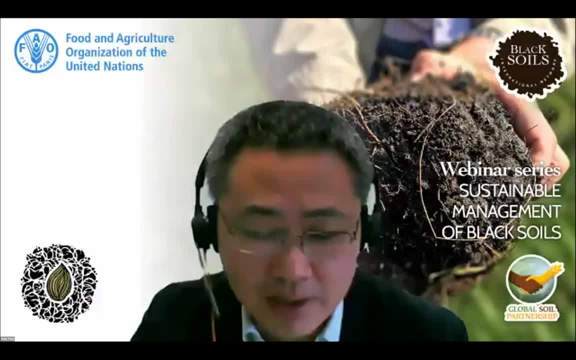 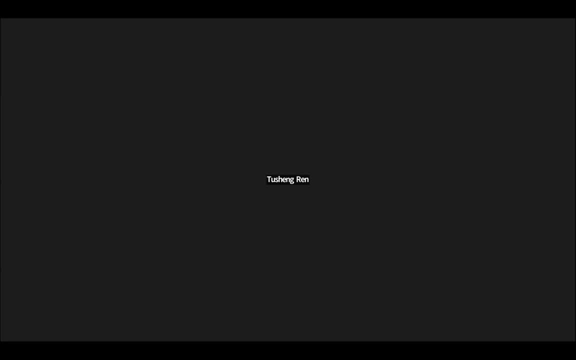 So what are the traditional practices in China in Black Soil region? Okay, thank you very much. Actually I have been working on the questions in the reply messages you know several times. Actually, the traditional system in North China is this: okay, 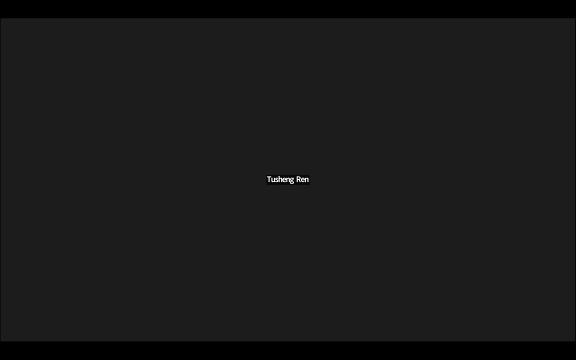 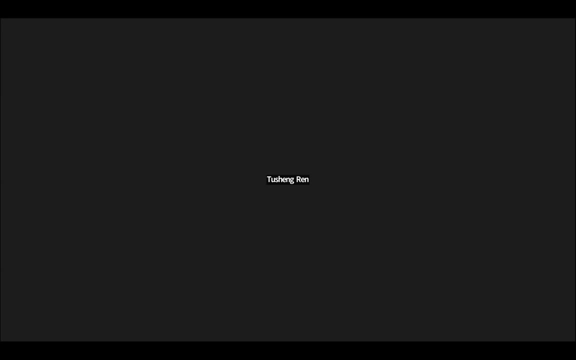 So it's really so. tillage and make ridges and planting: that's the three major operations And in recent years they because of the use of reduced tillage systems- systems like low-tillage tillage, okay- And now they have added another operation like sub-soling. 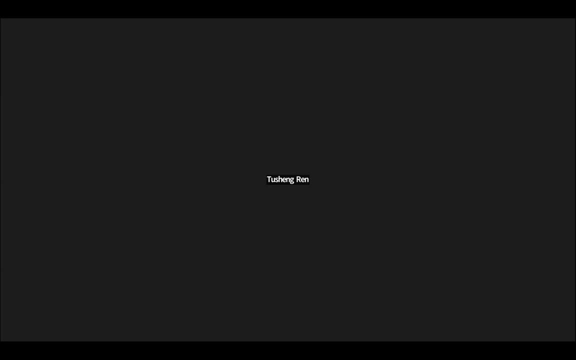 subsodium, sometimes in the after harvest and most of them do subsodium in the at the sediment stages. so the traditional system really. but I think, besides the trilogy, the farms always take the crop literature away from the field. so usually for for literature or in recent years, 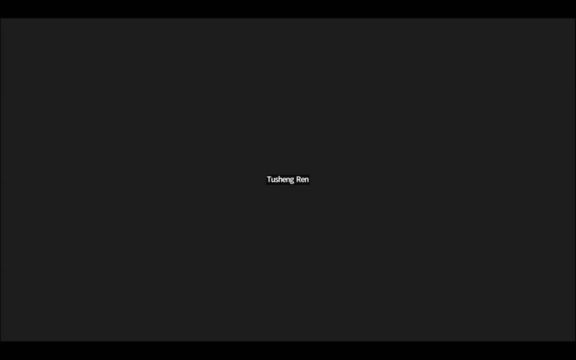 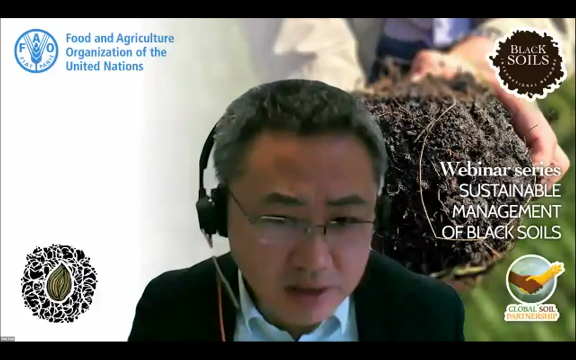 they just do building and making the feeding materials and also for making fields. so the crop legend was removed and the soil disturbances very often, you know, in that area. okay, okay, thank you, professor. and another question about the role of crop rotation and organic amendments in this system. what's the role of? 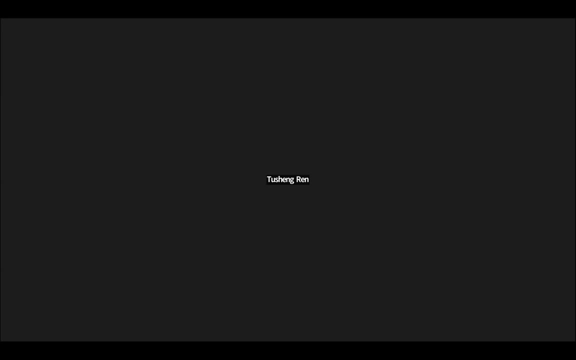 crop rotation and organic. that's a very, very good question. that's actually we have not resolved this problem yet, you know, because in after, let's say, several years of the no-kill system, because the system hasn't changed and some of the perennial weeds we kind of control with herbicides, so we 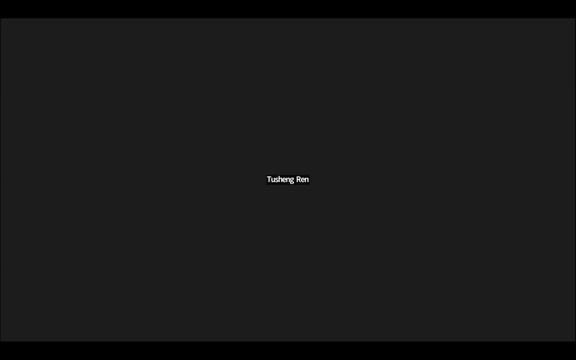 have to use just new rotational systems. like you might. you might possibly have soil behind the core so that can control some weights but not all of the weeds. so now we have do some other study like introduce some cover crops to control weights and all kinds of crops like rice and some other you know crops you know to control with. so we are still in study of 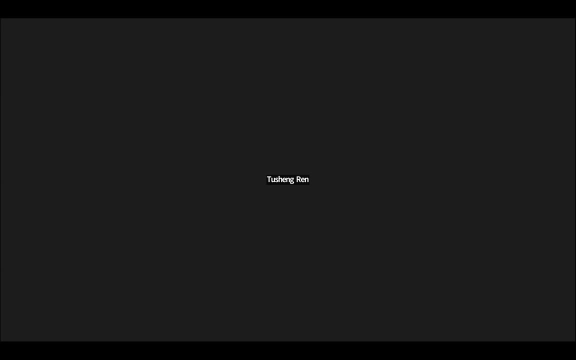 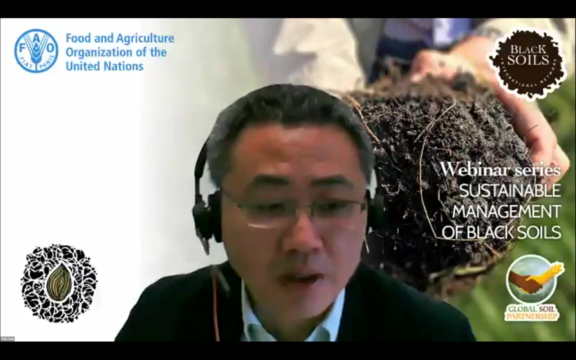 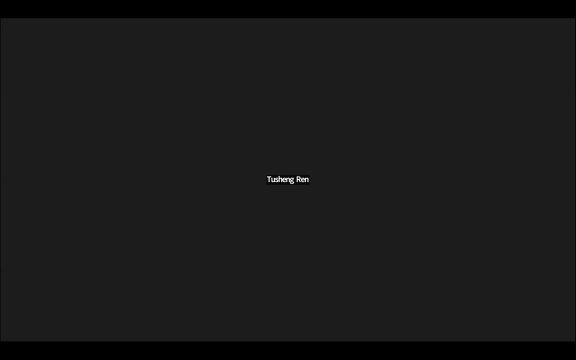 those kind of systems. So that's the one thing about cooperation. What is your other question about Organic amendment? Organic amendment, Yeah, That's a very good question. You know, actually a few years ago our students did some survey. you know, in the past the 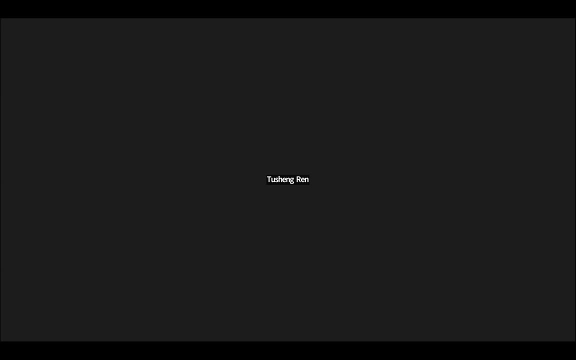 farms in North China had applied organic waste. you know a lot. That's the key way, that why the traditional system has been sustainable. But just in the last 30 to 40 years the farms have been forgetting the organic material and they use chemical materials. you know mostly. 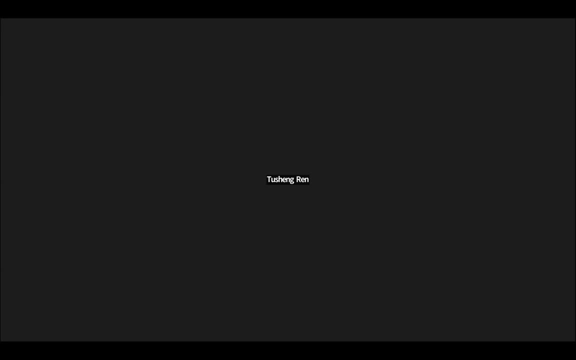 So we noticed that only less than 5% of the farms use organic manure in the past few years. But recently we have been doing research work to try to, you know, make some new things for the farmers to use the organic manure easily. 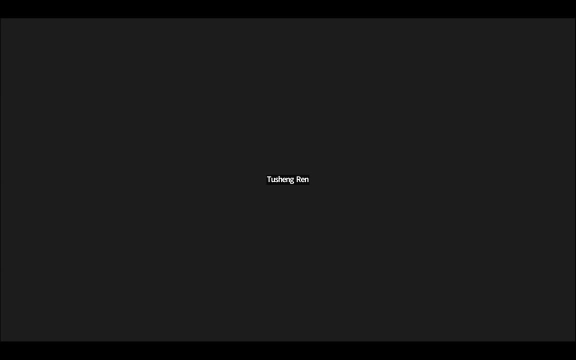 So there's some research and there's some equipment that has been developed, you know, in the last few years, And I think in the next maybe four or five years, organic manure will be used, you know, more and more by the local farmers. 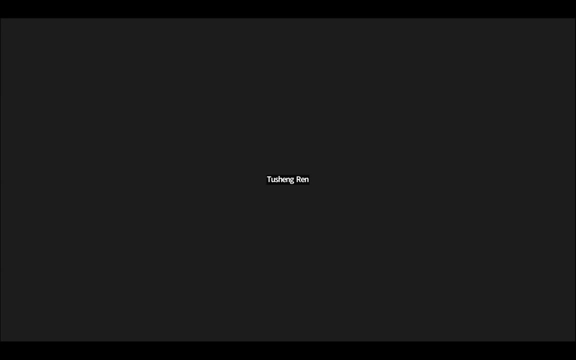 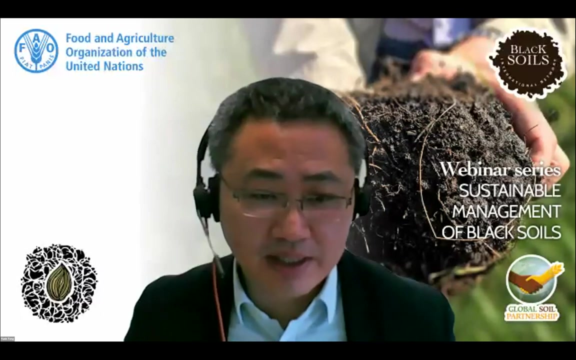 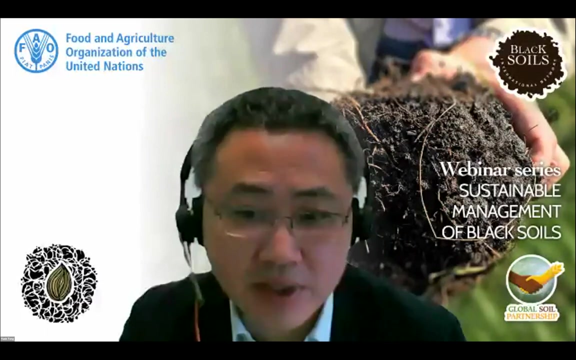 So we're still doing research and developing those technologies and equipment for the farmers to use organic manure. Okay, Okay, Thank you. Thank you, Professor Ren. A question is about what's the difference between conservation agriculture and no tillage. 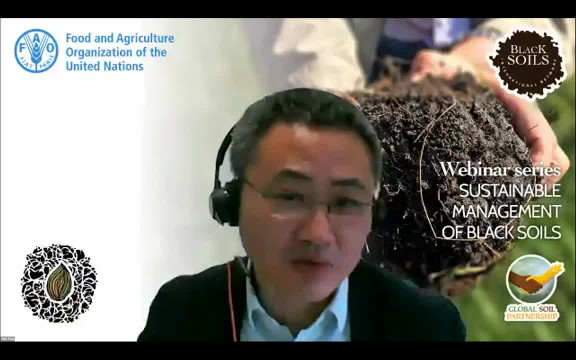 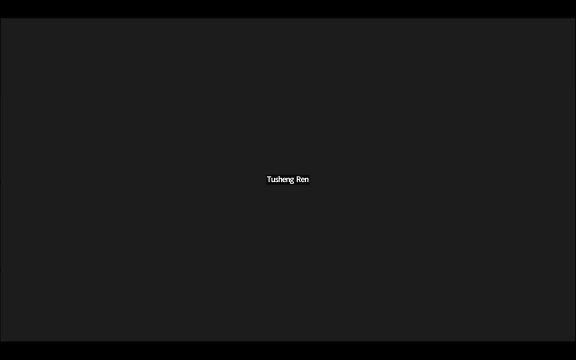 So what's the difference? Because some people are confused about conservation and no tillage. so please, thank you. That's also a very cool question. Actually, I just know, asked the question in the text message and actually conservation tillage is not really. it's a very big concept, you know. 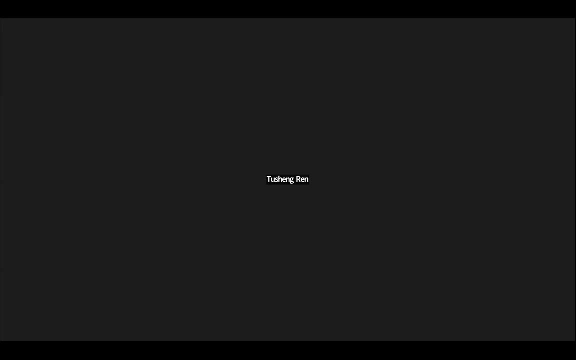 It includes many of the tillage systems. Just if you have a tillage system that knows the plot of soil, that's all conservation tillage. But no tillage is the extreme of conservation tillage, Because no tillage, you just remove all the tillage systems and also you have to have 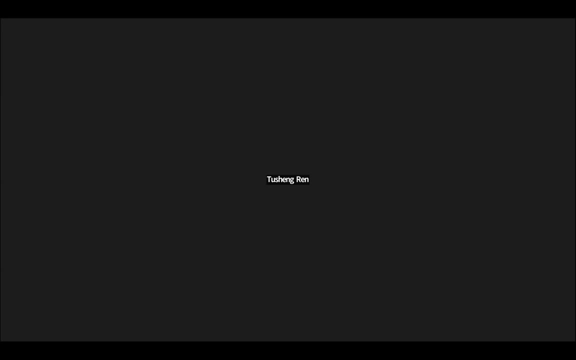 your soil surface covered by crop vole, At least 30% of the surface area should be tillage, Okay, covered by the surface. So no tillage is one of the extremes of the conservation tillage And also some people ask about the difference between conservation tillage and conservation. 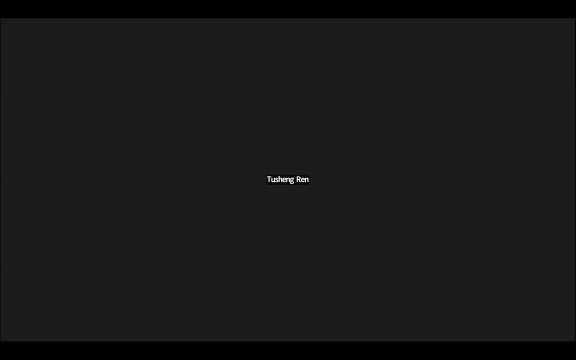 farming. So farming, I think, is even larger. You have to include crop rotation and other things in your system, So not really just tillage. So like passive control and fertilizer application and also the ratio between organic and chemical fertilizers. you know that all should be. 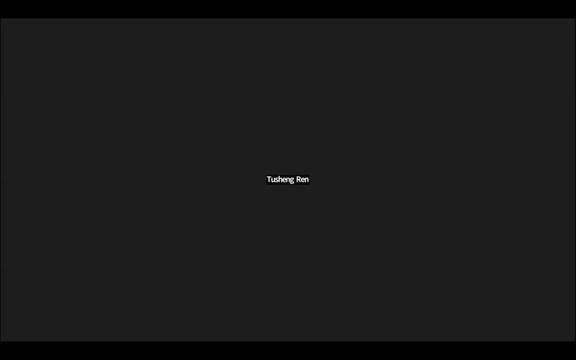 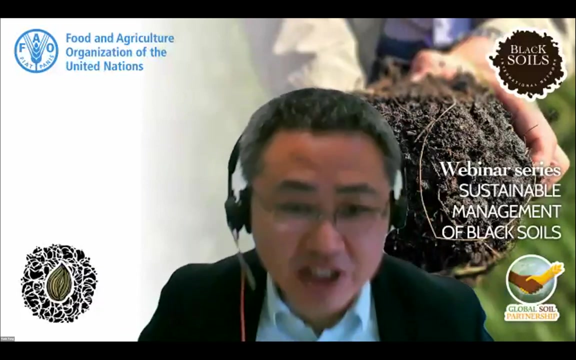 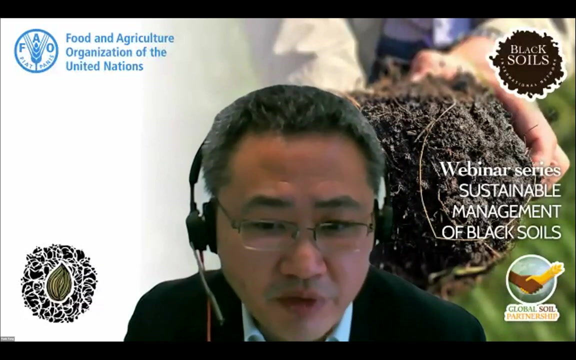 concerned in the conservation farming. Okay, thank you, Okay, thank you. The last question, the last question, So I think it's the reach to the extension services. So an audience participant asked how to reach farmers to really consume farmers, to adopt the good practices. 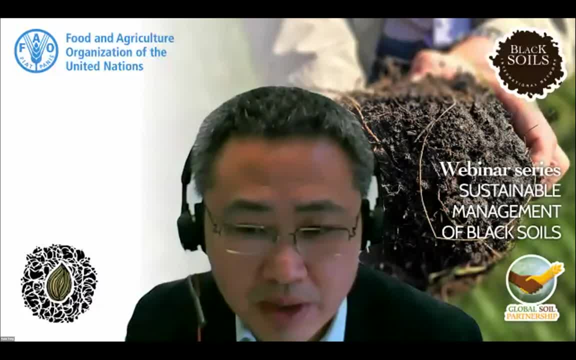 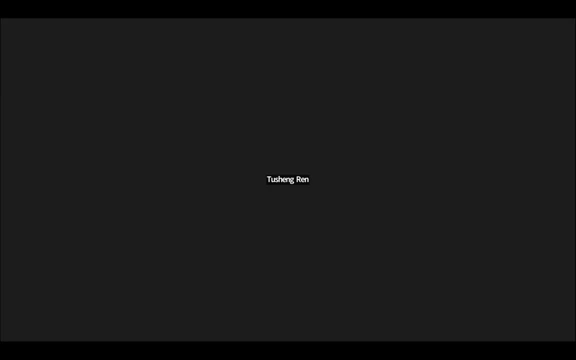 for black soil protection, How to reach farmers, How to- I mean- adopt good practices by farmers. I guess that's the hardest thing we have been doing in the past over 10 years, As I mentioned earlier in my presentation, that we extend a network of black soil conservation. 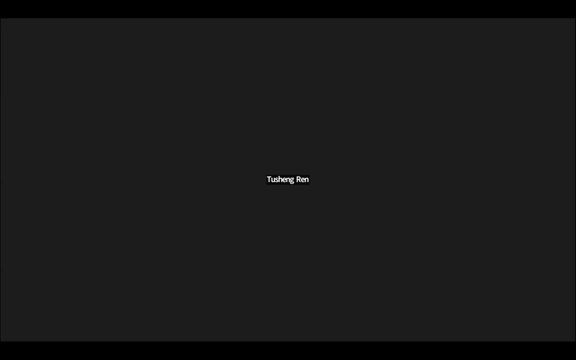 industry in China. Those are all the farmers. you know- At least I started. we started that in 2015.. We organized like 30 of our farmers in that area, So we gathered them together and we showed them how the No-Till Seller works. 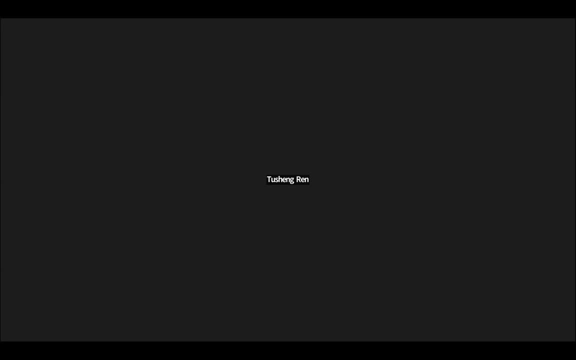 And they will give some training classes. you know How that works. That not only just us. you know those are engineers, okay, And they also helped them a lot and how to do the planting, how to control the weeds. 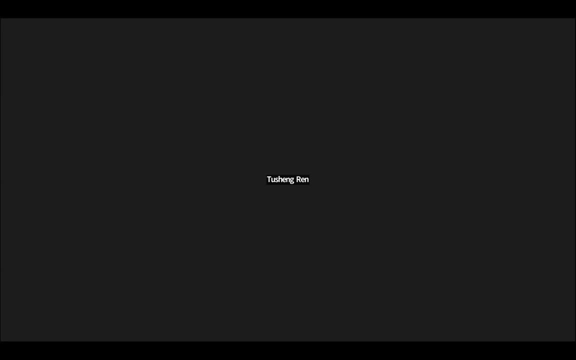 and how to apply 40 dollars. that's one thing. the other thing that you know, uh, uh. we are very fortunate that the local government are really helpful, but you know where else they give the sub subsidies to the farmers. so, uh, like, uh. if you use the local systems, they will give you like 40. 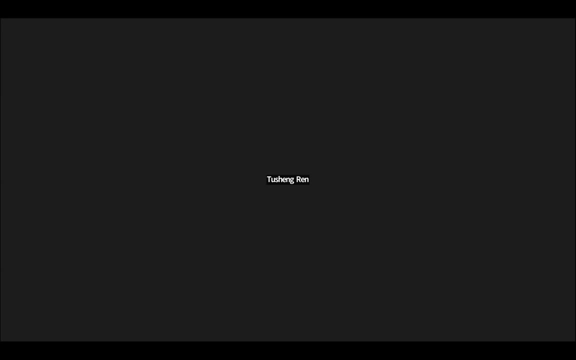 yuan to 60 yuan, you know, uh, for more, so, so, so the farmers can get some benefits from that. okay, that's another thing. the other thing that we did: some fair demonstrations. we have a note here, note here, and conservative plots, uh, yeah, in the summer and also in spring times and same times. 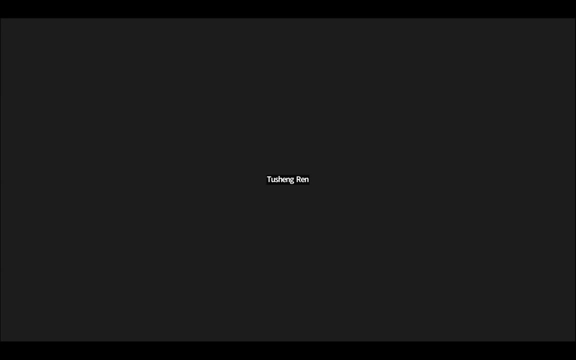 we invited the farm to see how that operates in the fields. and also, you know, at harvest times we invited them to go to fear to say: you know what's the difference between the different systems in crop yield and crop performance? and the last letter: you know, every year with uh in the winter times we have a summary about our progress, uh we made in the past. 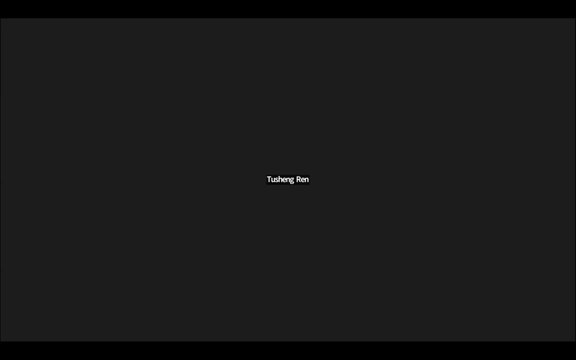 years and we give some awards to those farmers. you, they used our system, you know, and uh, so, uh, i think, slowly, the farmers are getting bigger and bigger and now we have our 100, uh, the bigger farms joining us, you know. and also i think we have to say that, uh, if we have those organizations, you know, we can. 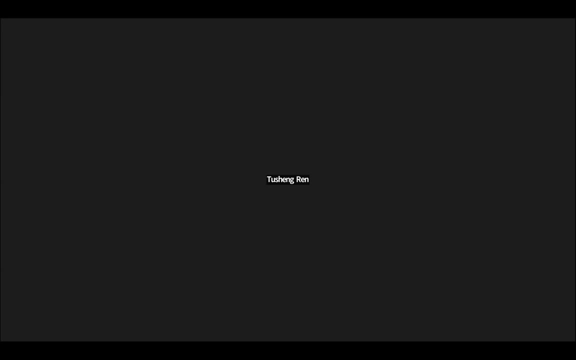 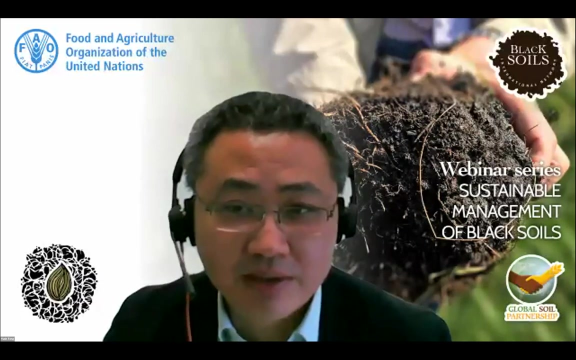 uh, make the price of the seeds and the fertilizer cheaper, so that is also attractive to them to to to use our system. okay, thank you, thank you very much. thank you very much, professor uh, and your answer to the question. thanks, thanks a lot. so now i i just have a suggestion. okay, uh, you can leave my 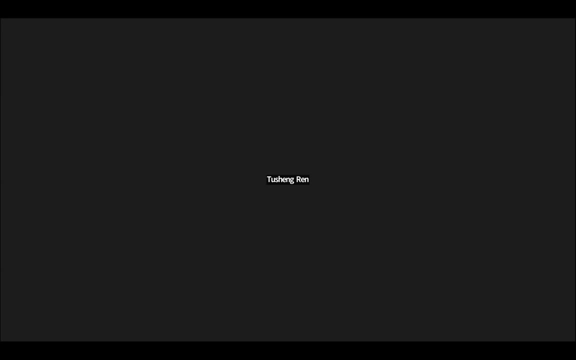 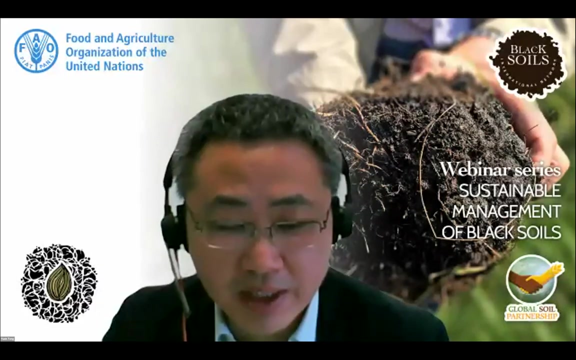 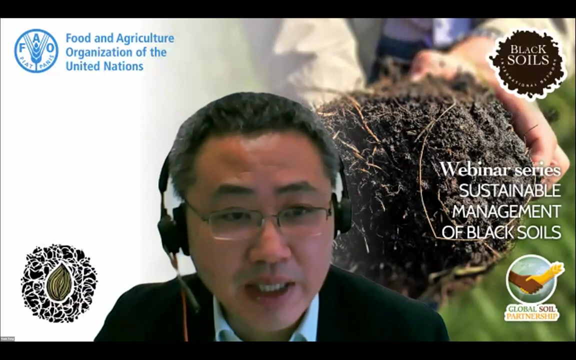 email message to to those people so they can send messages later. i can talk with them later. okay, okay, perfect, we will. we will share the information. thank you very much. so now i would like to move to professor chen xia li uh about the questions addressed to you. so, 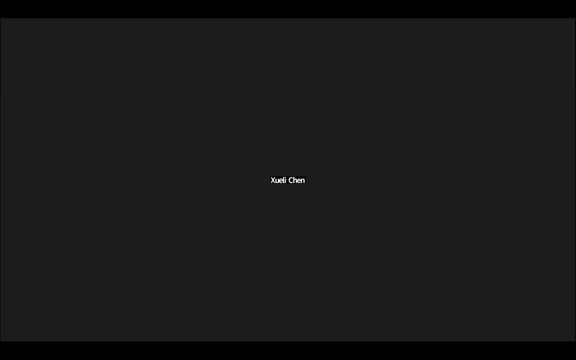 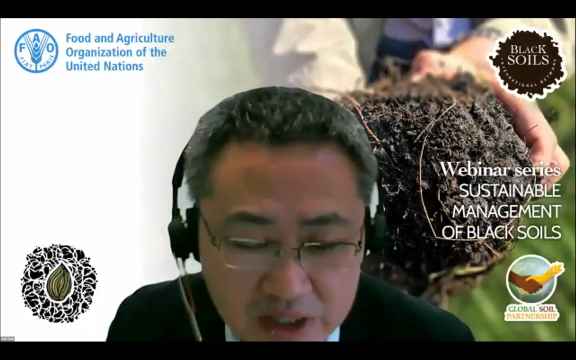 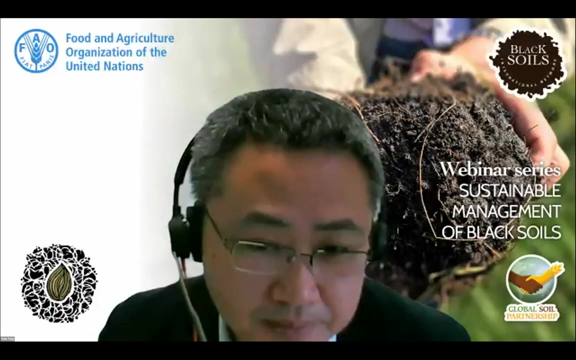 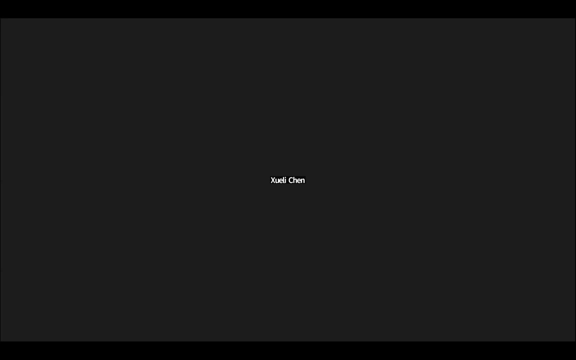 yeah, okay, yeah, thank you. so the first first question is about the quantity of organic fertilizers. so how? how much quantity of fertilizer, organic fertilizers, that is crucial for increasing soil organic matter- okay, actually, the organic matter, organic materials include manure and straw- is different types of. 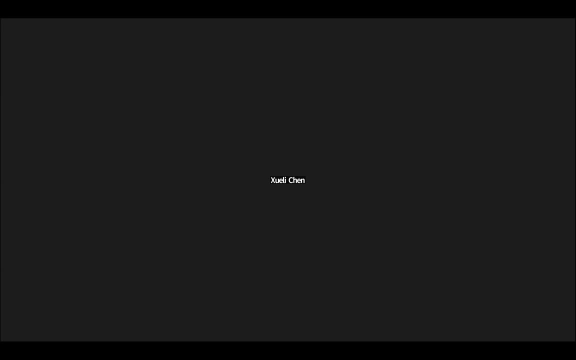 organic matter inputs the soil. actually how much and how the um? how much the organic carbon in the uh, uh a manure, uh could transf it great transformation to the soil. organic Republicans, you can use my biouuuuuuu catches. is it um largest? i think it's a. yeah, our research result: we found 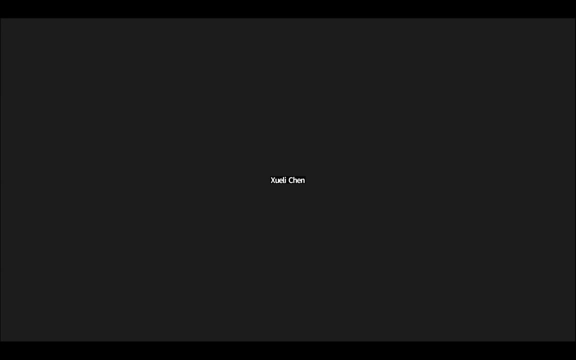 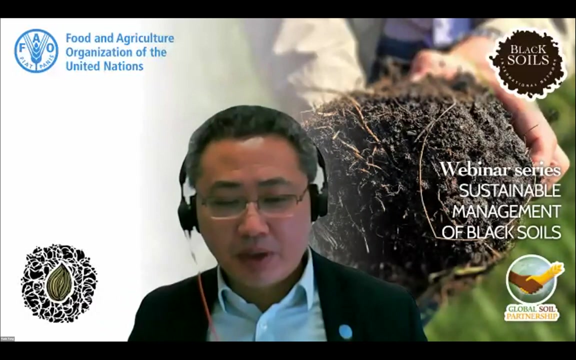 uh, worth, uh much value. something can calculated by the natural level, a content sample for the natural chemical, for the, the input, and then we calculated how much the manure input. is it clear, okay, thank you? thank you. i think another question is about biofertilizer. uh, what's your opinion about biofertilizers? 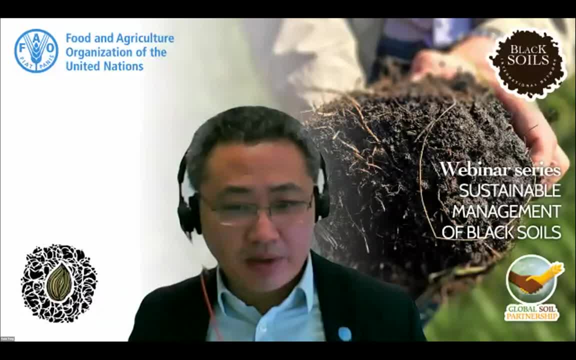 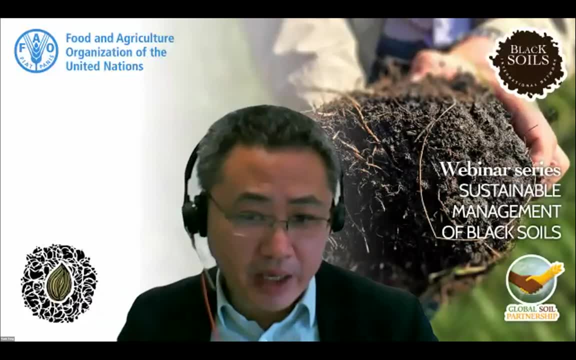 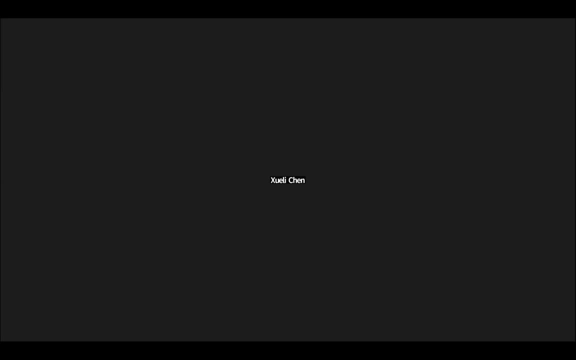 so, because sometimes it's not, it's complicated, but very important. so what's your opinion about the biofertilizers and how? how could you use biofertilizers in the field? yes, biofertilizer is a very important product to improve the soil quality, but, as you say, the 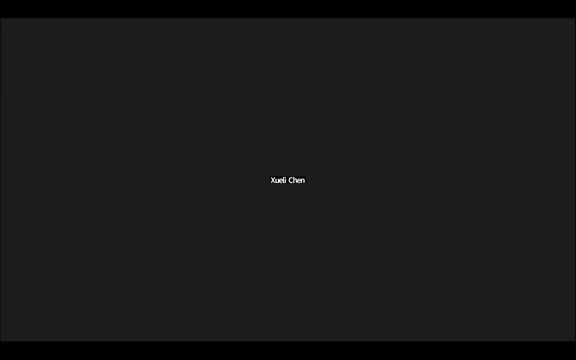 quality of the. the bare fertilizer is not really uh, uh, not really the the at the same level. uh, i think the first problem is the uh bacterial of fungi of the stomach. make your organism should be survived in the soil and then they can play some functions. so the 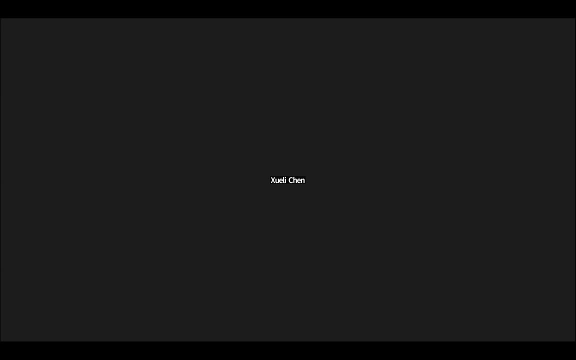 key problem is the how to give them the suitable environment. um, in my opinion, i think we could, we could do some research or application for the bell fertilizer used in in uh, used used by the uh, how to say in the high organic matter fertilizer, together at first, to make sure they are the real. 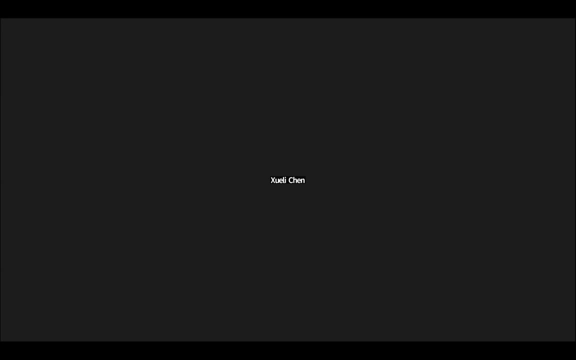 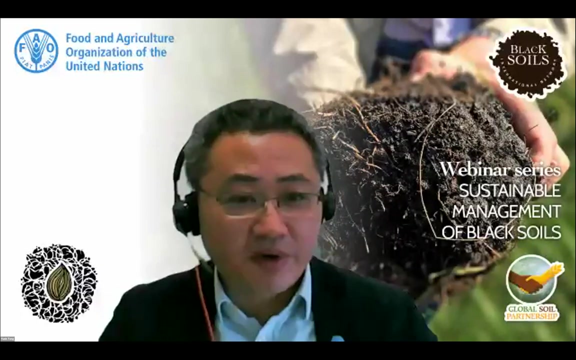 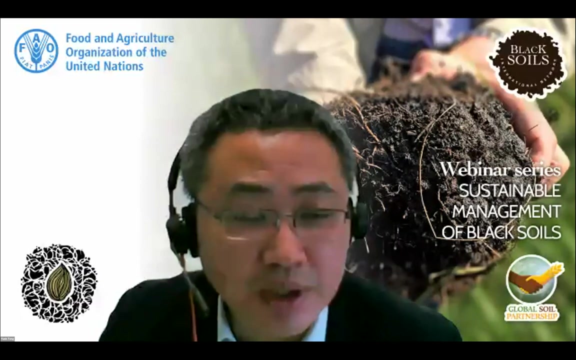 and the second, i think, in my opinion, is: uh, we should give more uh uh standard for the bell fertilizer production. okay, thank you. thank you, professor chen, and thank you for your answer to the questions, and now i would like to move to professor jia. professor jia, are you here? okay, thank you. 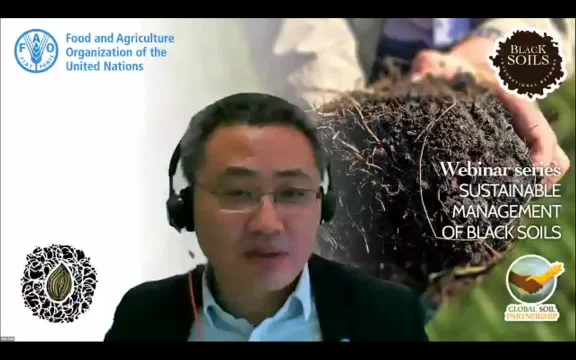 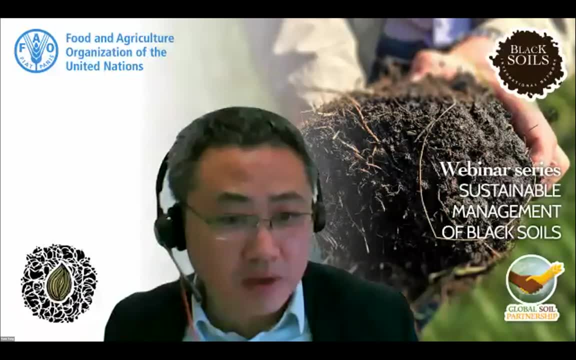 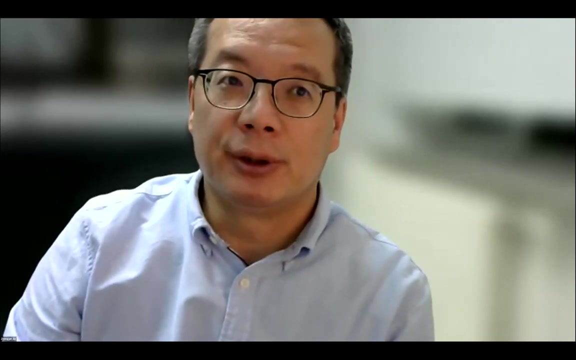 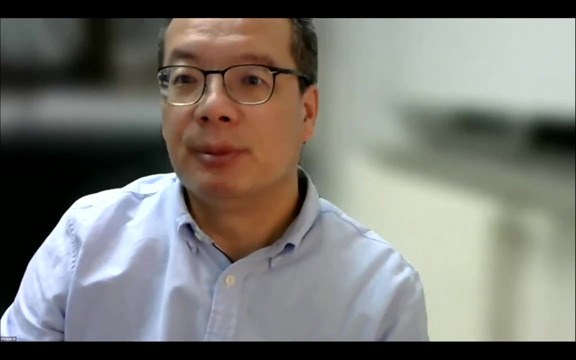 thank you, thank you, okay. so i think there is a question about the para parent rock. so can parent rock determine the black color of black soils? so, no, no, no, no, no, i don't think so. and if he or she learned from the presentation of the doctor, actually there are many dust, yellow, like the duster which is moving from. 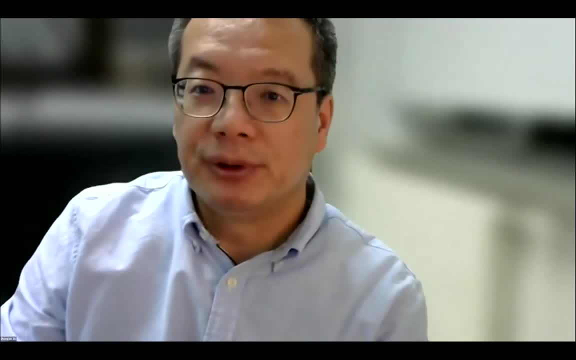 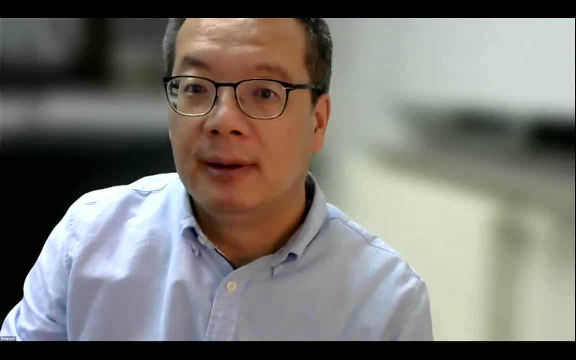 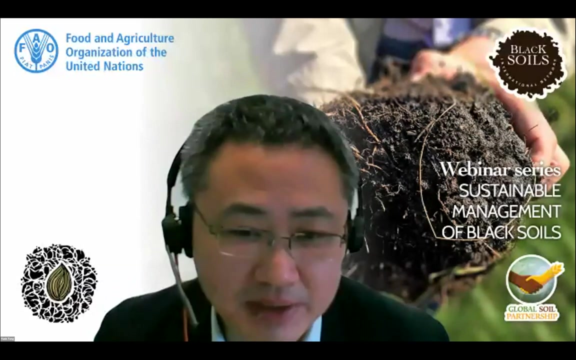 the central part of the channel and then from sent to the northeastern channel and then decompose as part of the black soil is a deep soil in a deep layer. thank you very much. okay, thank you, professor. another question is about- i mean, something happened before. is black soil adequate? 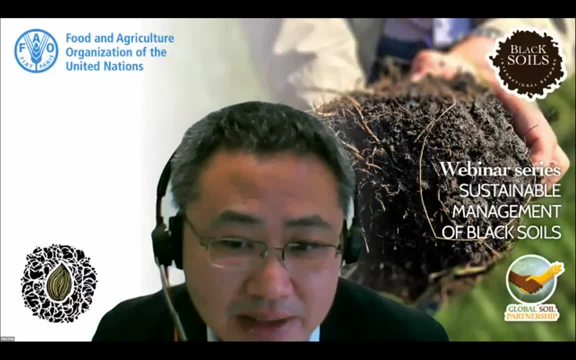 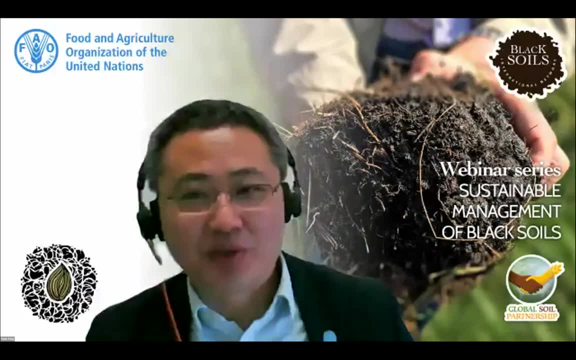 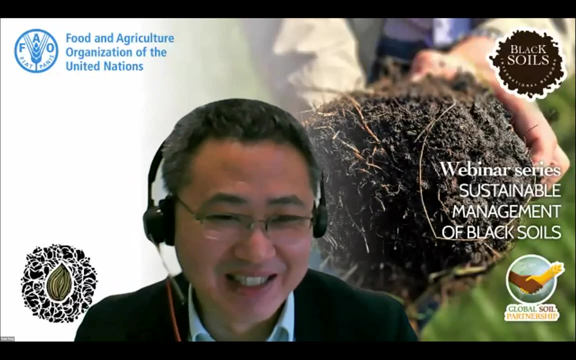 to mine or apply to other soils as a dumb amendment materials. i think this question is about to uh to to to use black soil in other regions to sell black skull use. so this is a question. yeah, now, in principle there is no problem, but i mean technically speaking, in practice, i think. 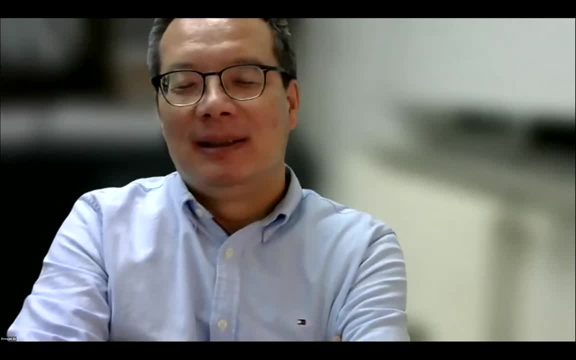 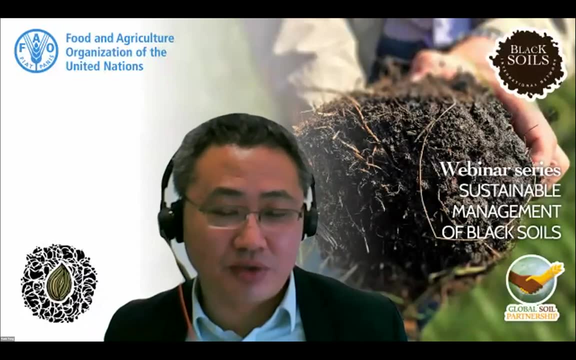 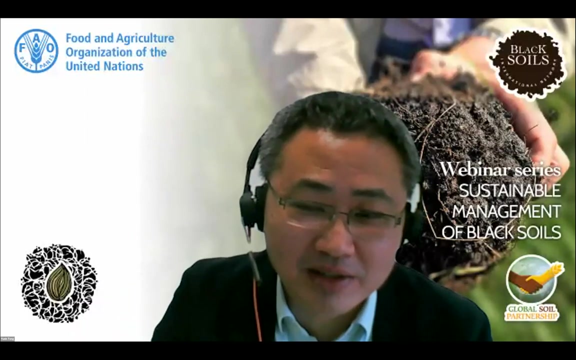 it's extremely difficult. thank you very much. okay, yes, i think also the from the blackstone in china it's forbidden to sell black soils to other countries. because i read the news like before, there are some people sell black soils, big, big aero black soils, and 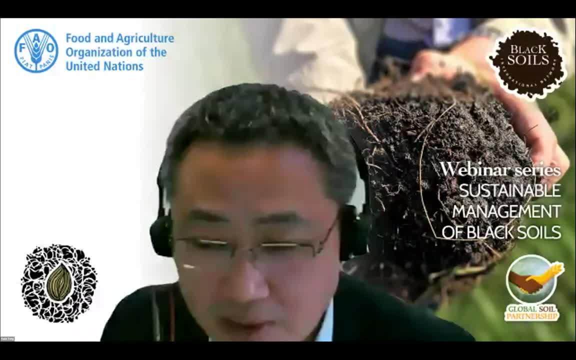 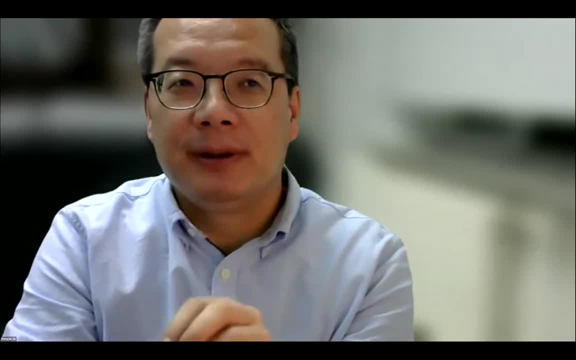 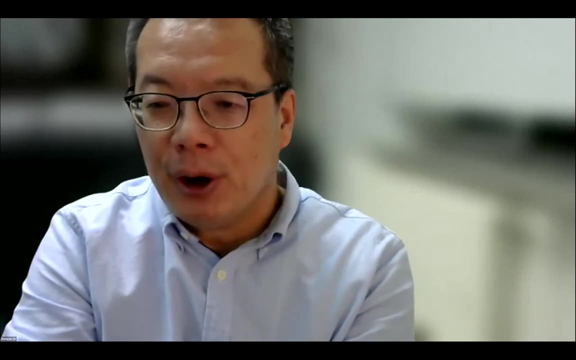 degradate the black soils in the northeast china and sell them in the southern china. okay, i would like to offset one thing the mr lee from dr lee mentioned at the very beginning of this seminar. he mentioned: uh, china now is the only country that has제. 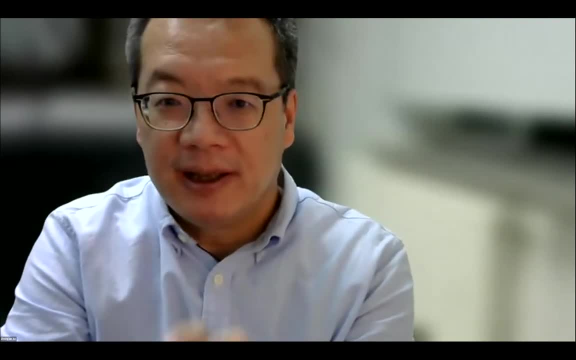 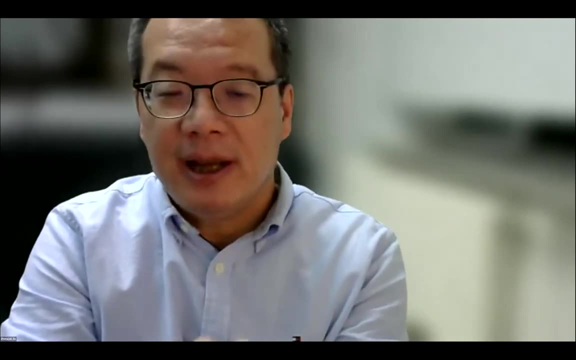 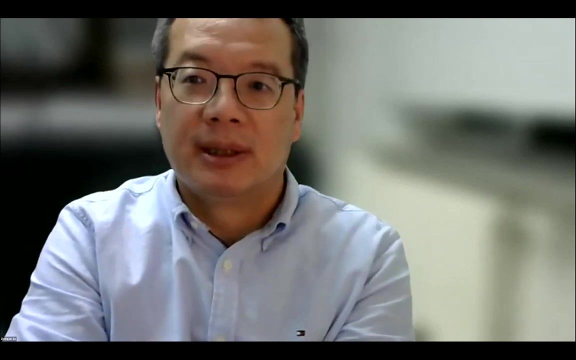 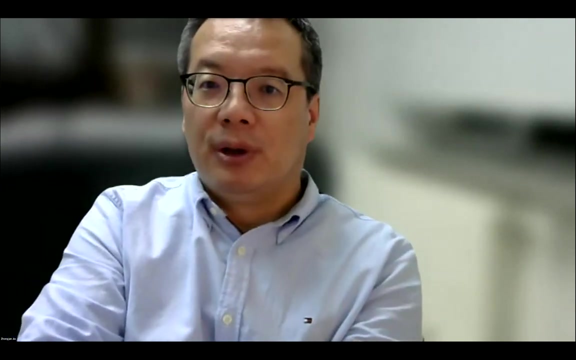 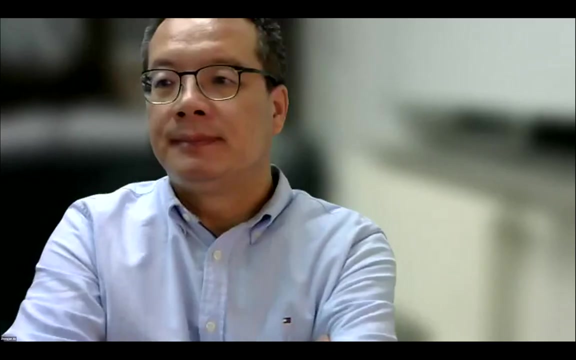 black black soil protection legislation which was issued by the chinese national congress, national congress of the chinese people. so this is the only one legislation in the world. so it's strictly forbidden to forbid. it will forbid the black soil. applications from the northeastern channel to other place is strictly forbidden. thank you very much. thank you. 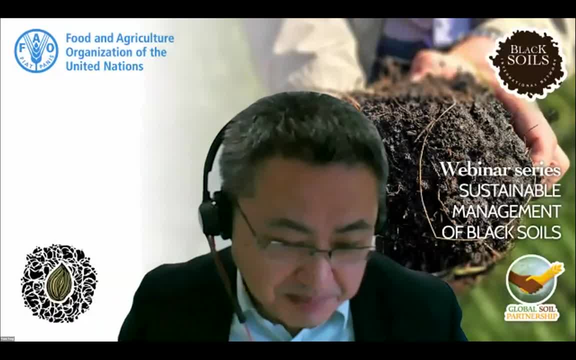 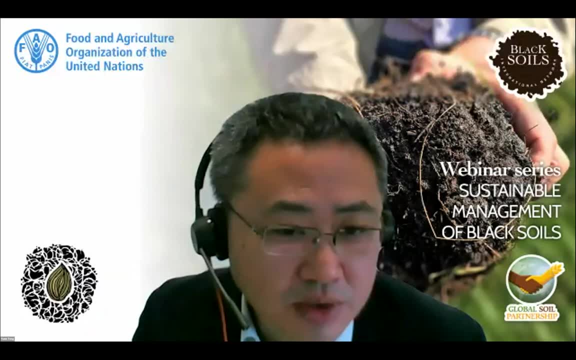 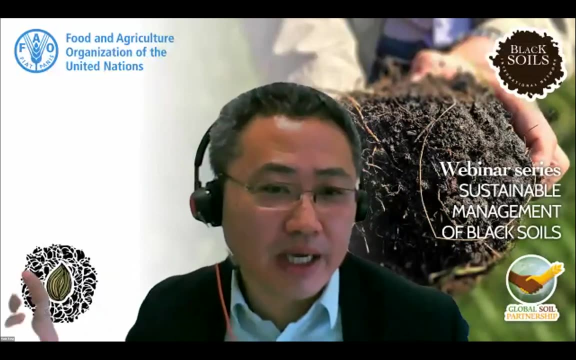 thank you, professor. yeah, another question is: uh, from my side. so i see you mentioned, i said, paddy soil, so it means those black soil are i have a problem of acidification. so because black soil generally have it's thought that the ph is higher. so what? the situation in northeast? 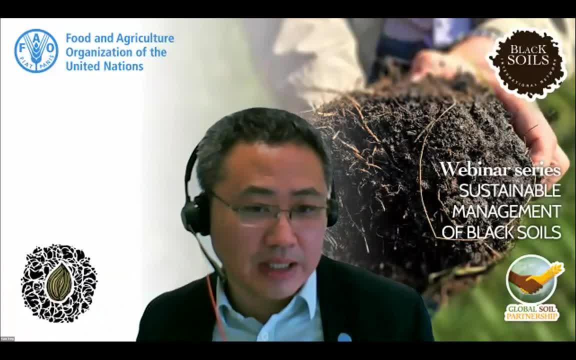 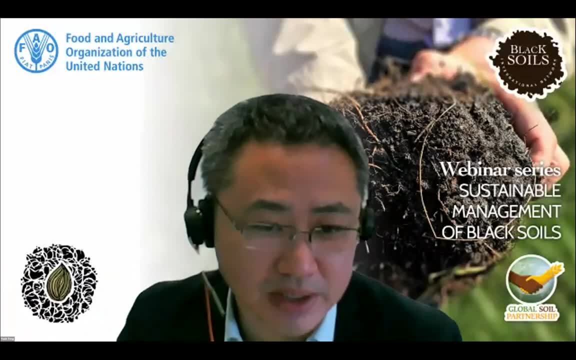 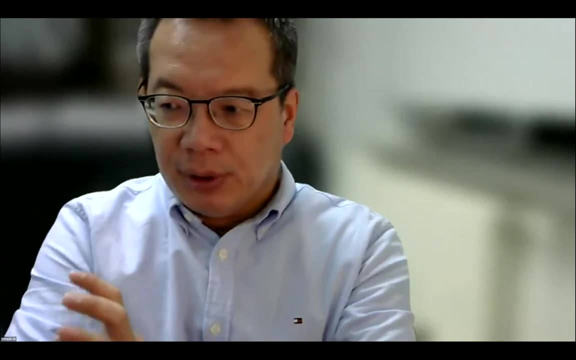 china about the acidification of black soils and but it seems it's very serious in party soils. so please explain a little bit. thank you, yes, thank you very much. i would like to say so because, as you, as you, as you remember, so the the acidification soil, acidification in the northeastern. 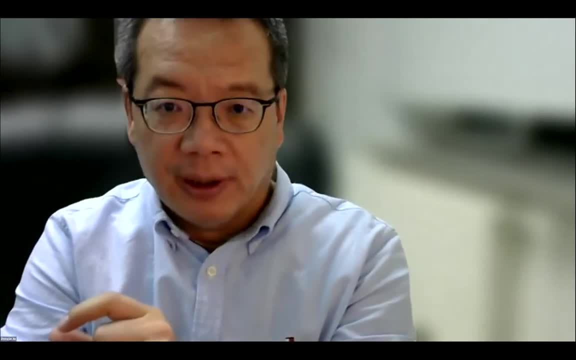 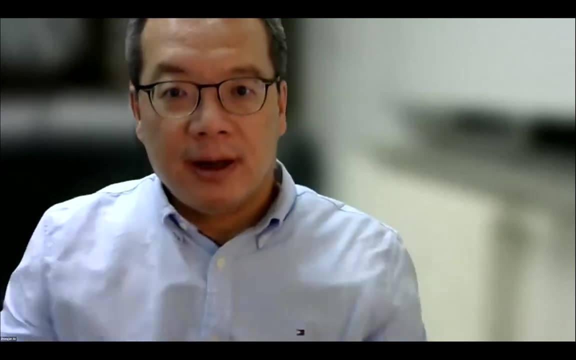 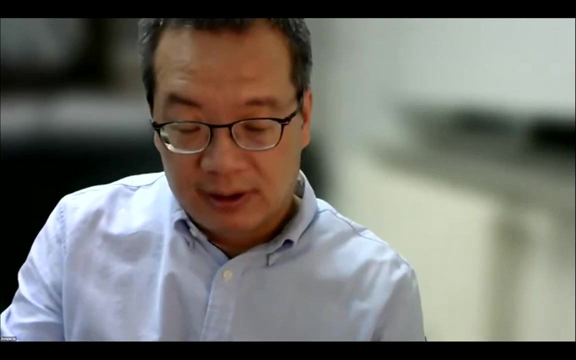 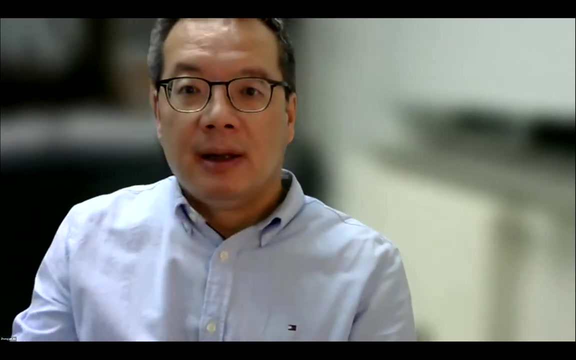 china is a severe problem very recently, because there are lots of the chemical fertilizer that are applied into the field and then, and in the, mostly in the form of ammonium, and ammonium is is oxidized to the nitrate and then, well, it releases the proton which makes the which makes soil acidification. so, as very a long time ago, generally speaking, soil ph in black soil is around the 60.5 to 7, but now many place is it the? the range is largely between the 5.5 to 6.5. so and then, this is one thing. the other thing is uh. 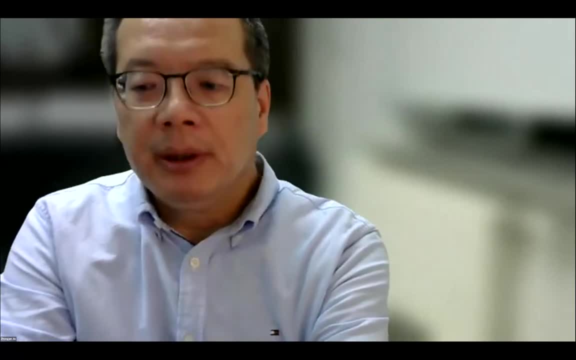 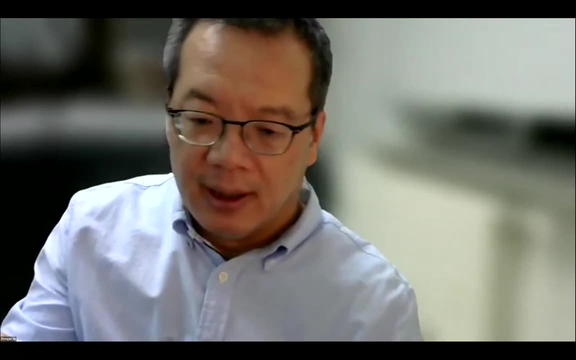 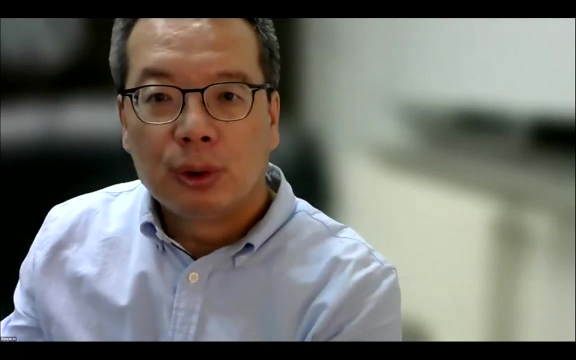 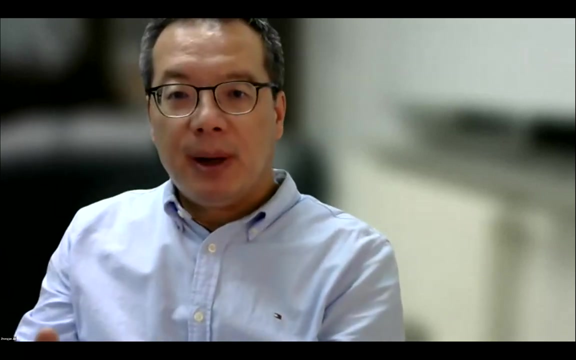 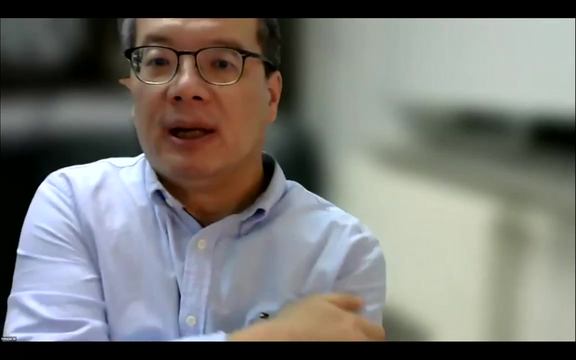 because you see there is only the three crop here: the, the, the, the C, C, depression, contraction from the, the synthetic 德 road and low-raspid expression of the soil. so it is a severe problem and if people are very concerned, you know the me Ranger Rudolph. hydrogen, Rap, sex, TED program, because i would like to say, you know, the the, even though negative, most directly emerged into the plant is if the natural activities are already in good quality, the plant is seemingly隨. gifts are in felicitation. in return, the nitrate or ammonium. in return, the protein also released into the soil to make the any protons. 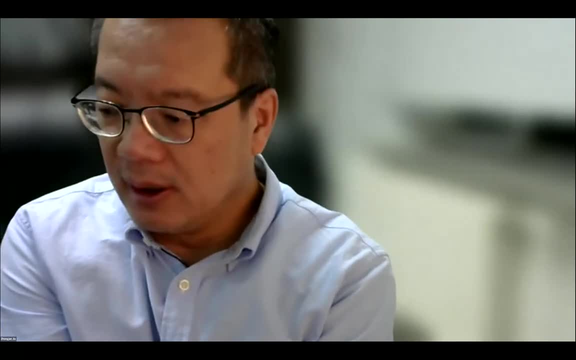 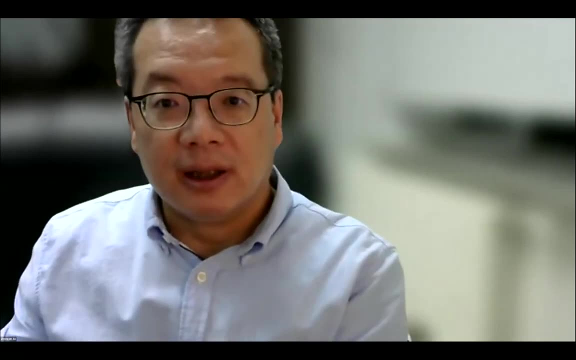 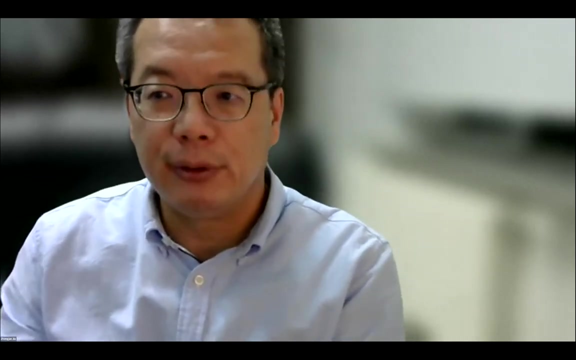 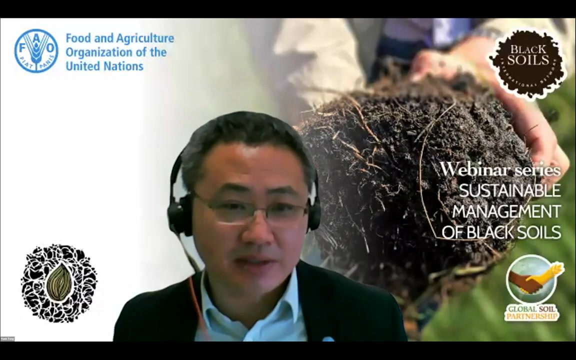 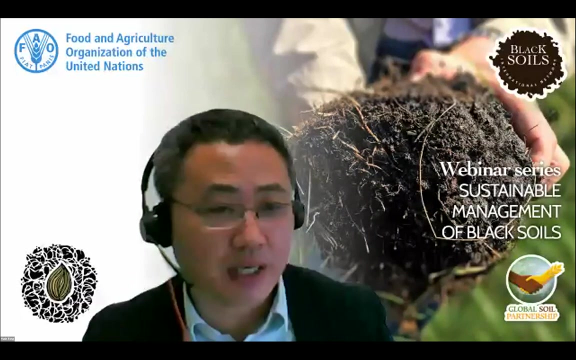 The Academy of the Chinese Engineering Academy also launched a program about the soil acidification in China, particularly in Northeastern China, very recently. Thank you very much. Thank you very much. Thank you very much for your answer And we are happy to see that the scientists and the government noticed that the acidification problem in Northeastern China black soil area would be a big problem and they start to address these issues now. 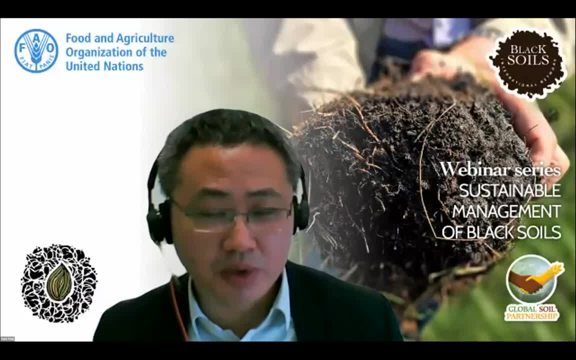 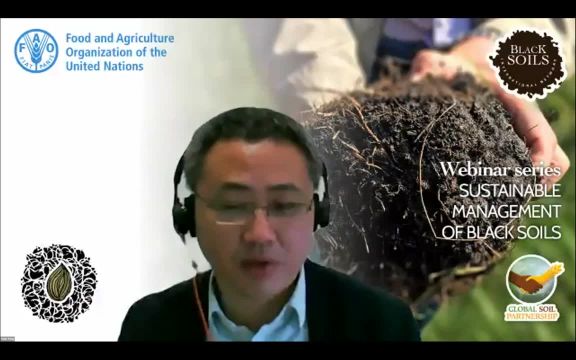 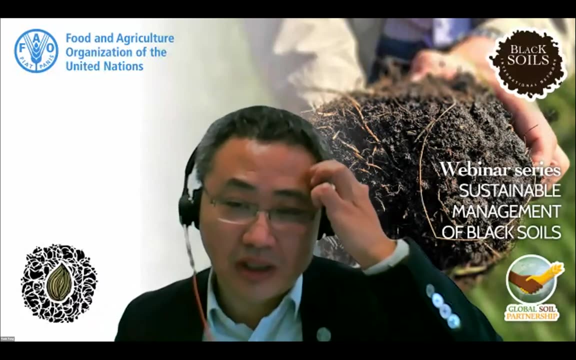 So that is very important because from the researchers they noticed this is a problem and then trigger projects from the government to start To prepare the solutions as soon as possible. So soon, it's good, It's very good, It's great. Thank you very much for your answer. 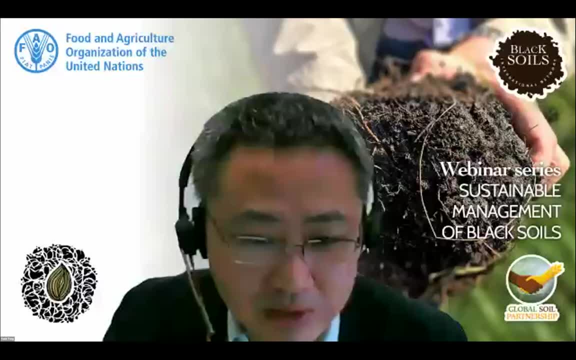 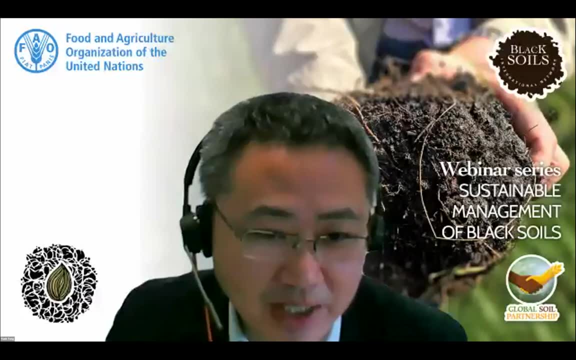 So, thank you. So I think we address some questions, but because of the time limitation we I'm sorry we cannot address all the questions from the audience, But we have saved all your questions and we will answer them in our webinar report. 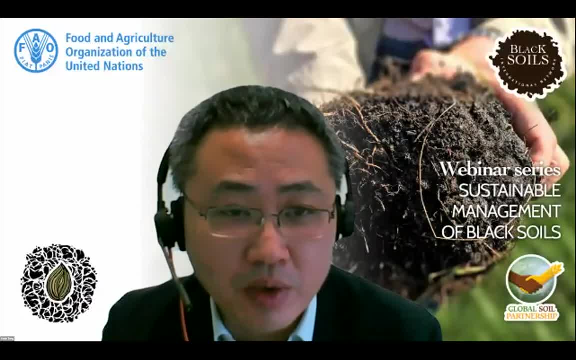 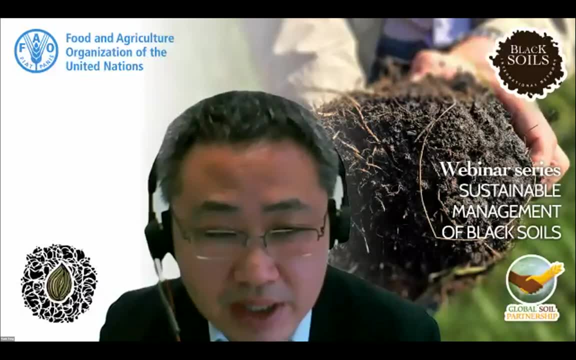 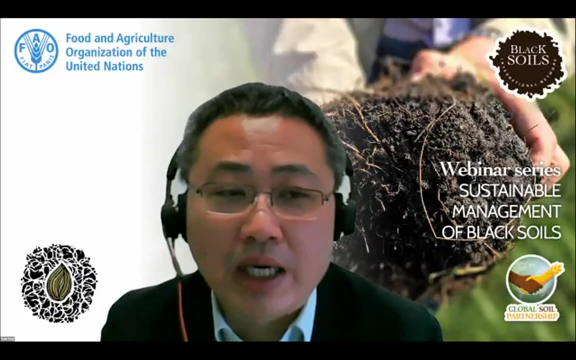 In the end. I will also want to answer a question from audience like: can we share the presentations? Sure, we will share the presentations on our website and we will send the link recording include the recordings, including the presentations and also the agenda, to use through emails. 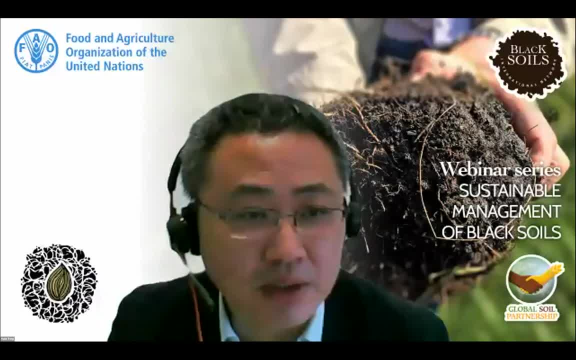 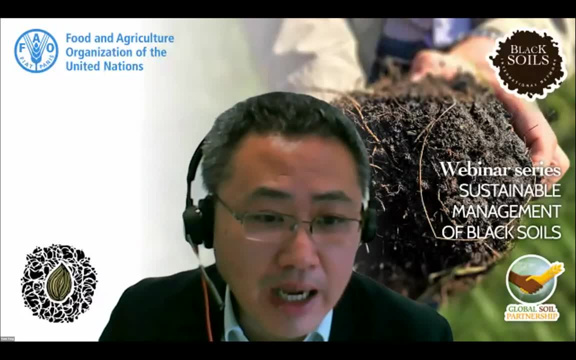 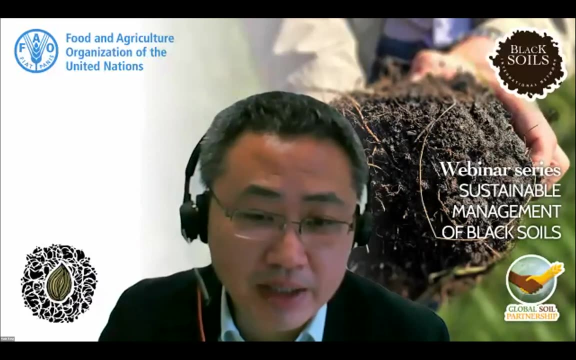 after two or three days, after we summarize everything later. So thank you very much. Now I would like to I'm glad to invite the chair of the International Network of Black Soyuz, Professor Miguel Cubacca, from Argentina, to give us a closer remark. 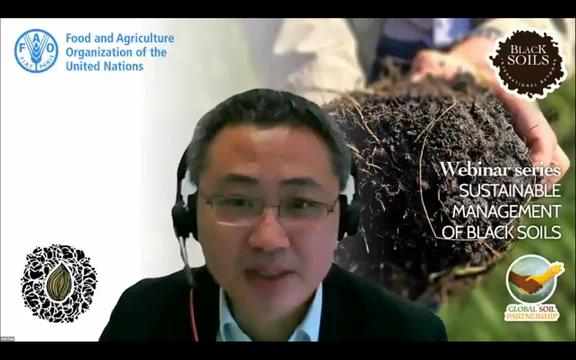 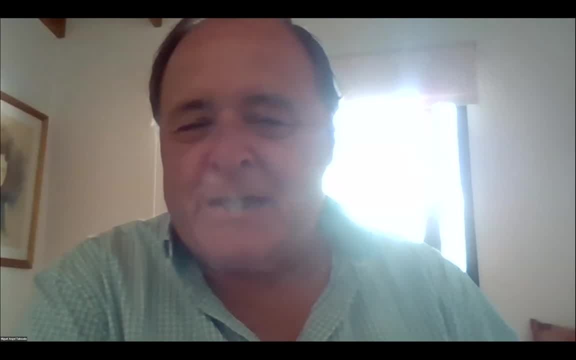 So the floor is yours, Miguel. Thank you, The chair, our chair, Okay, Okay, thank you, Yuxin. Thank you, thank you, And good morning, good afternoon everybody. I think that there are only a few minutes. 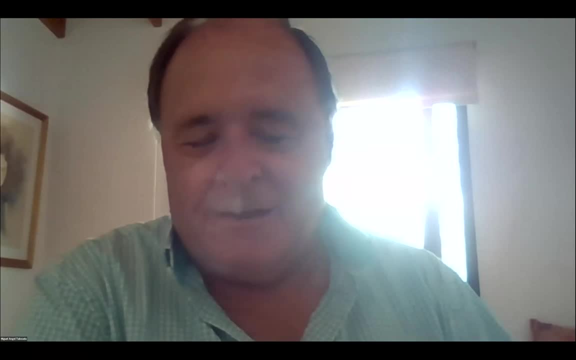 so I will try to be very, very brief. Many thanks to all lecturers and thank you by the excellent presentations and thank you for all the attendance. I think that the webinar was highly successful in terms of number of attendance. There were never lower than 200. 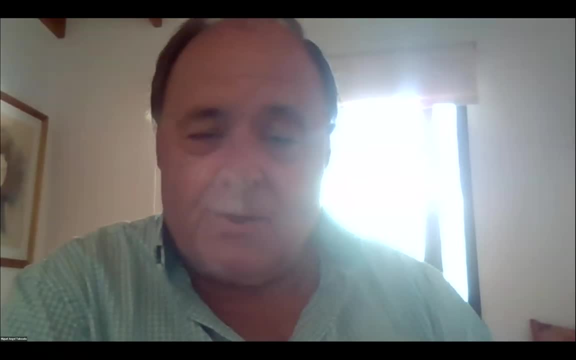 and averaged 280 during the two hours of all the webinar. This manifested all the interest in this webinar. I think that all the lecturers helped us to describe and to meet the objectives of this webinar that were to describe and analyze different good practices for black soil management in China and black soils in China. 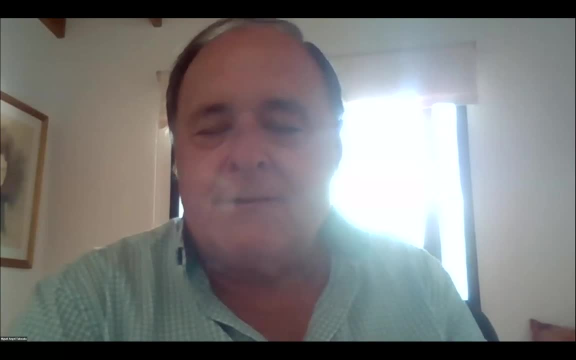 particularly where the use of no-till farming and all the limitations and benefits of no-till farming in China that they are. I listen to this very with attention because in my country they are also no-till farming and the conditions are very, very different, particularly in terms of. 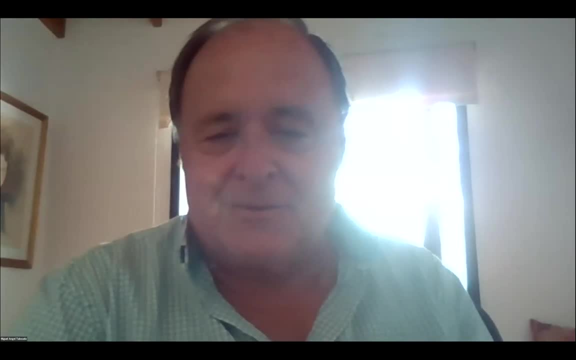 climate and soil formation. So it was very, very, very good. It was very good how to increase soil biodiversity by the application of different amendments and organic amendments and increasing biodiversity and the impact in different in soil microbes and soil bacteria. Very, very. 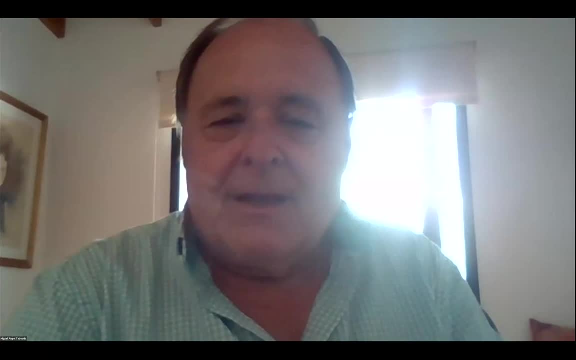 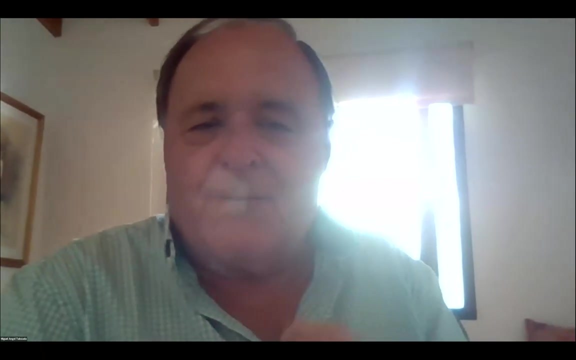 very good This presentation, and there's good, very good presentation in terms of the explanation of why soil nitrogen and soil organic carbon are so high in black soils of China. It's very interesting, but it seems that the cold climate seems to have a particular, a very important, key role. 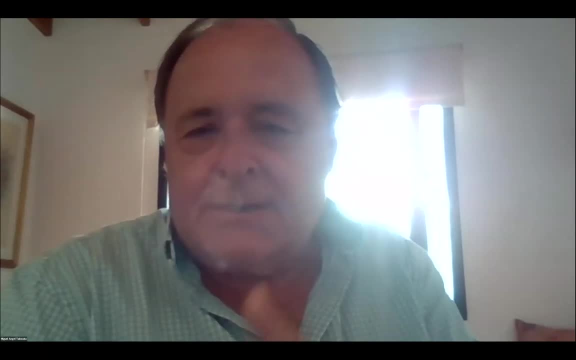 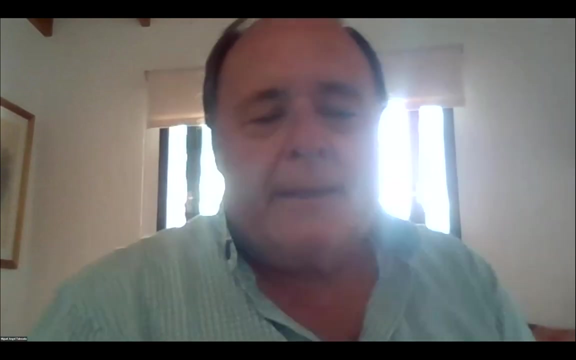 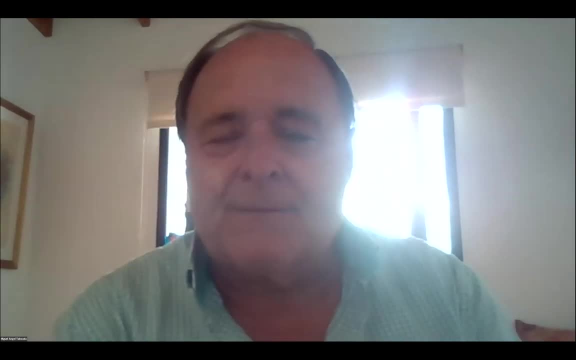 What as well, 55. indicative of this webinar, particularly in the gaps, are the general volume and some of the deductions within the in the lateral section Right. it also contributed to identifying gaps and challenges. It was the other objective. members, thank you. 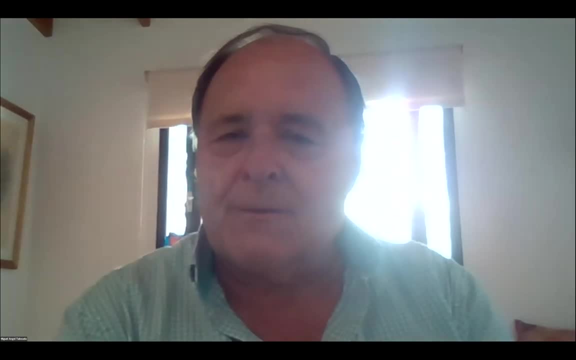 the interrogation about the, the time of formation of black soils, that it seems to be longer than supposed, and the uh, the analysis was, was very, very interesting and the influence of these that have not only the different paramaterial and tone and climate, but also by observation and particularly the, the, the analysis of how fat soil is former, black soil is a former, and the role. 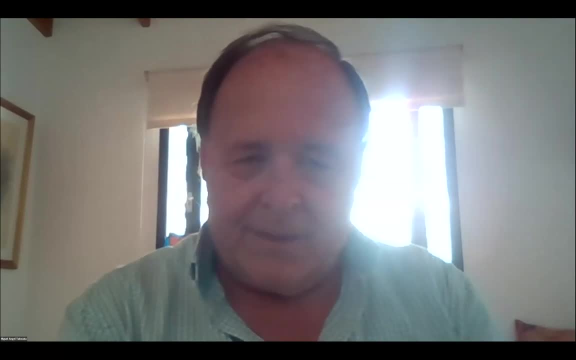 of bioturbation and does the position okay? and by the end, this is the second webinar. the first webinar was: uh was in argentina in november 2023. uh was highly successful and this second webinar they're highly. they're closely connected because both countries have black soils, and particularly argentina, black soils of argentina. 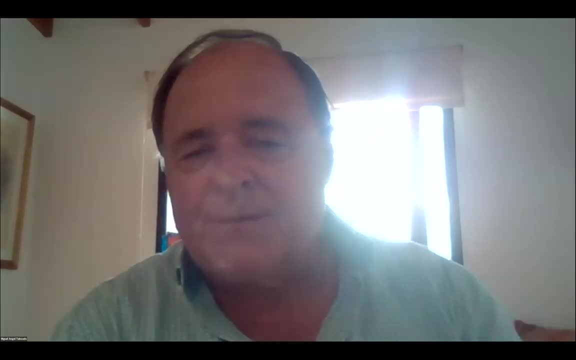 are devoted to grain production and most of the grain, particularly soybeans, exported to china. and so, despite this difference, at a different climate- because we have no snow in our country- the threats on the soils are quite similar, so erosion, lower organic matter content and balance of plant nutrients. so it's very interesting to analyze how. 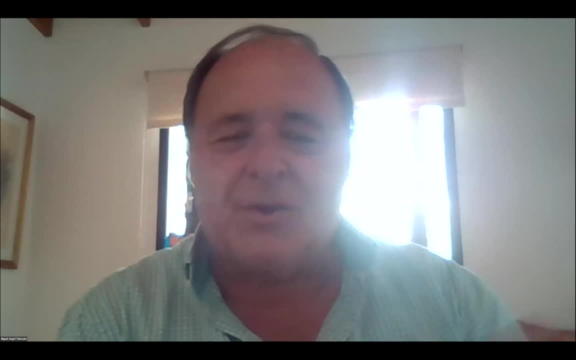 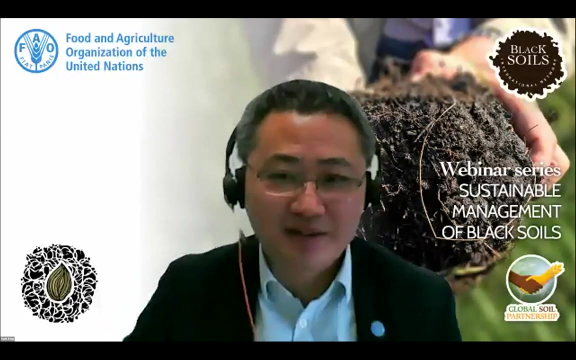 different conditions led to deep, to similar soil fruits. so, uh, many thanks to all of you and i see i i hope to see you in another webinar. many thank you, thank you. thank you very much, chair. thank you very much, miguel, for your conclusion and the summary. 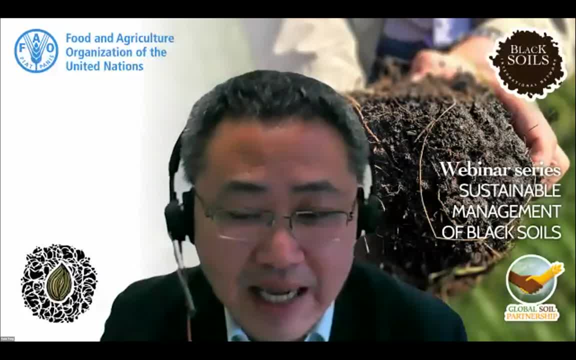 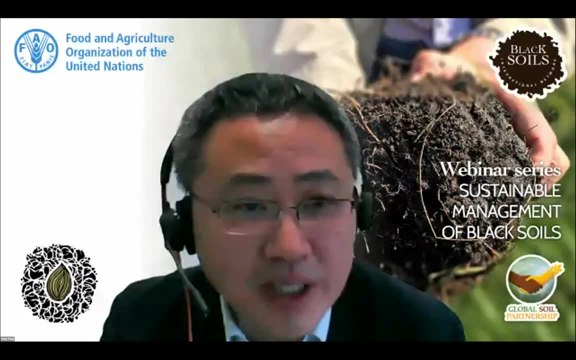 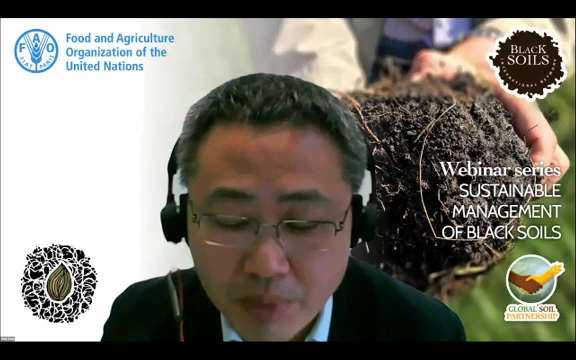 yes, you are right. this webinar is excellent and we invite a very, very knowledgeable uh experts from china and they introduced their practices, their good studies and also some scientific point of view, like the formation of black soils. i also learned a lot from this webinar and i'm very